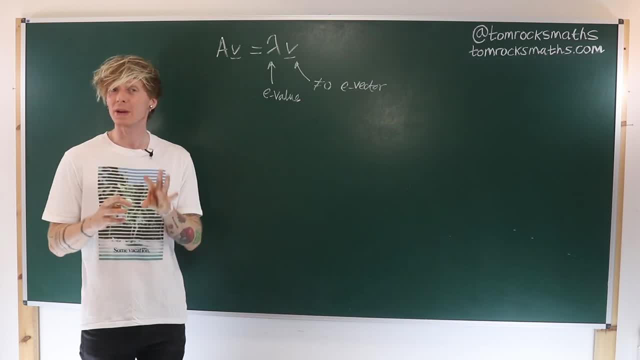 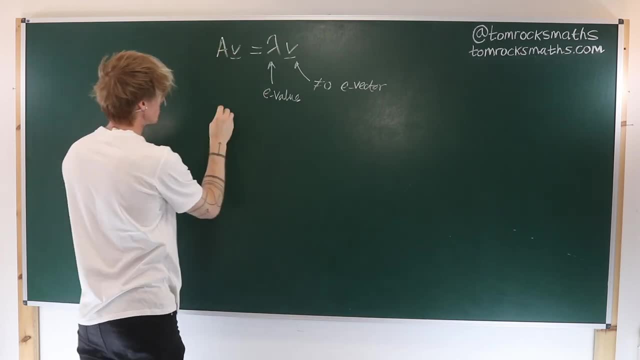 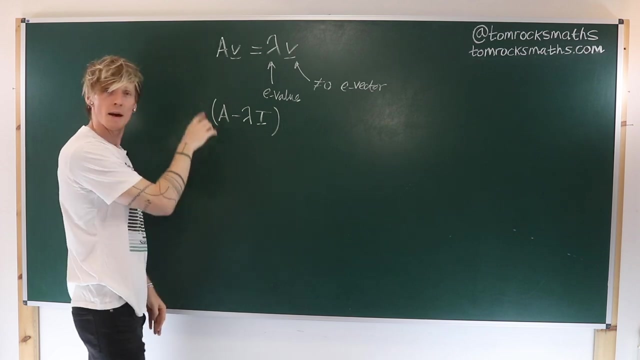 actually lies in determinants. But before we get to that we can start by rearranging the equation. So if I take this over to the left-hand side and we factor out V, then I can say A minus lambda times the identity matrix, so that A minus lambda makes sense. 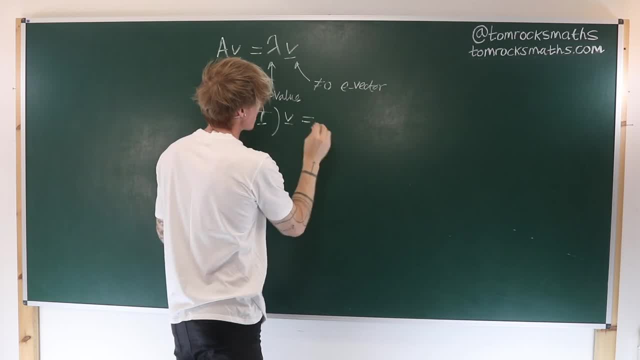 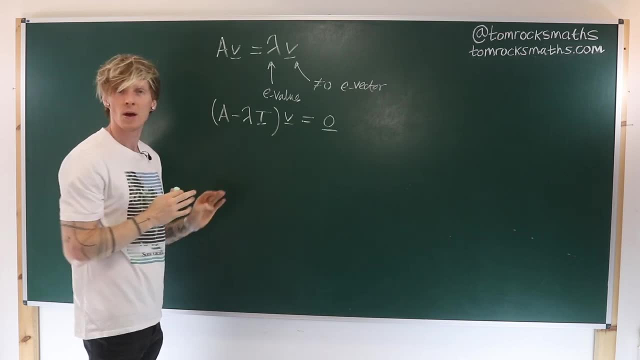 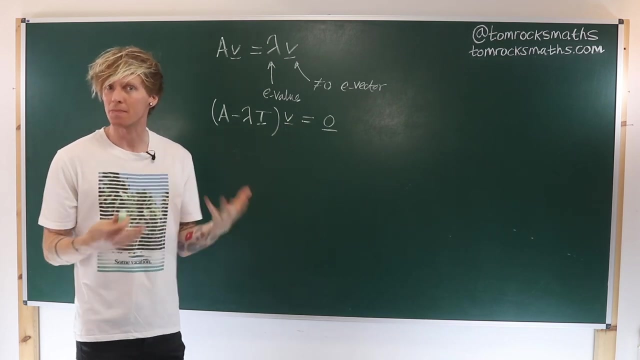 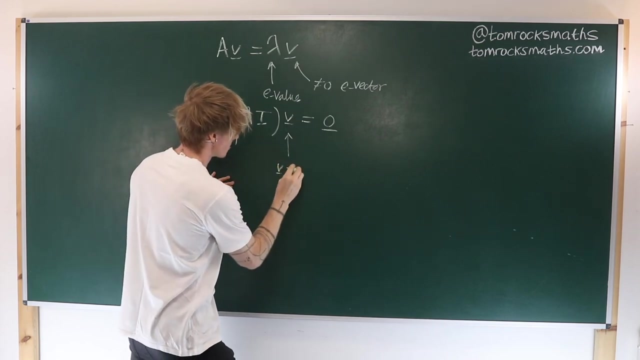 multiplied by V has to be equal to the zero vector. So now we have two terms, when multiplied together, that need to equal zero. So we can proceed in the usual manner and say: well, suppose V is zero, This is our first option, So V could be zero. and then this matrix multiplied by zero definitely gives me 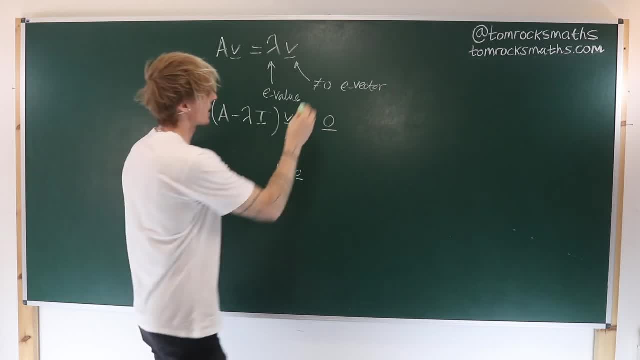 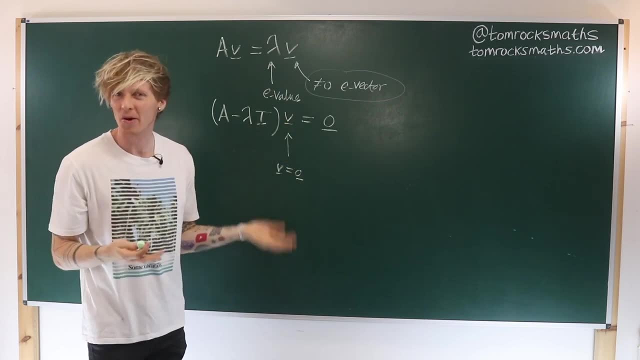 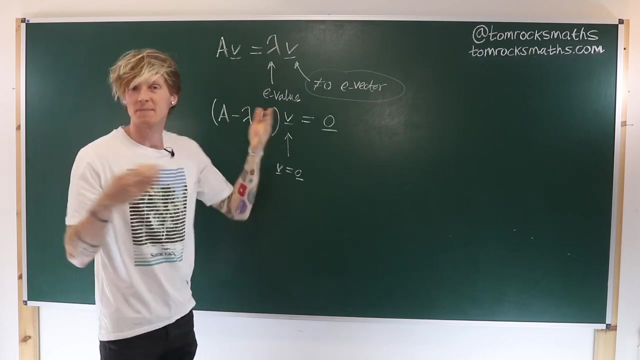 zero, And this is why we actually specify here that we want a nonzero eigenvector, Because if it's zero it's kind of boring and the whole equation is obviously true: Matrix times zero vector equals number times zero vector. They're both zero. 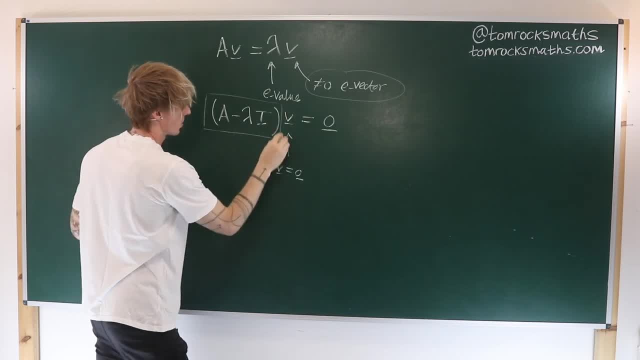 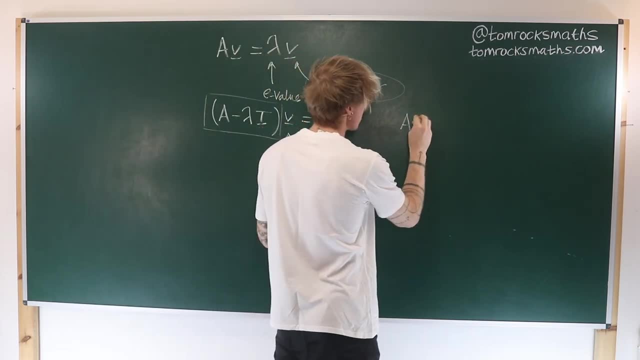 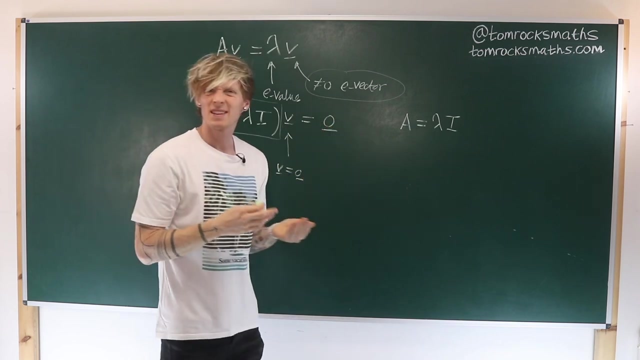 So instead we proceed by saying: we want this to be equal to zero. Now, if A minus lambda I is zero, that means our matrix A is equal to lambda times the identity matrix. but then that really limits the type of matrix A that we can actually investigate, because this 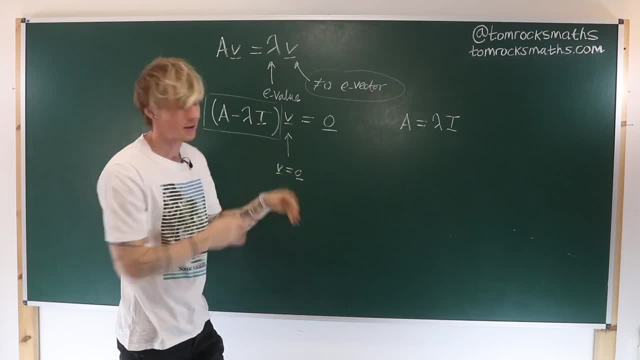 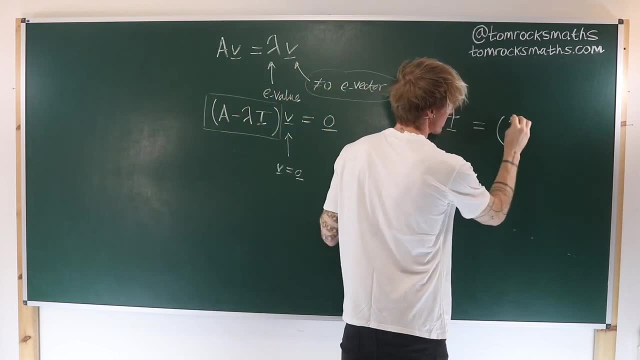 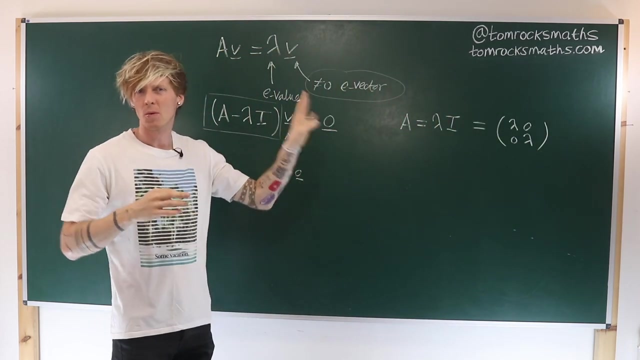 says. the only way this can be satisfied following this method is if A is actually just a multiple of the identity, So it would just look like for a 2x2 case, something like this. Very boring and again not really what we're interested in. We want to look at general matrices A, So what we 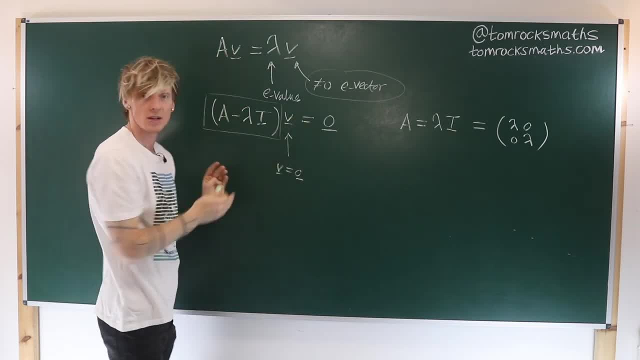 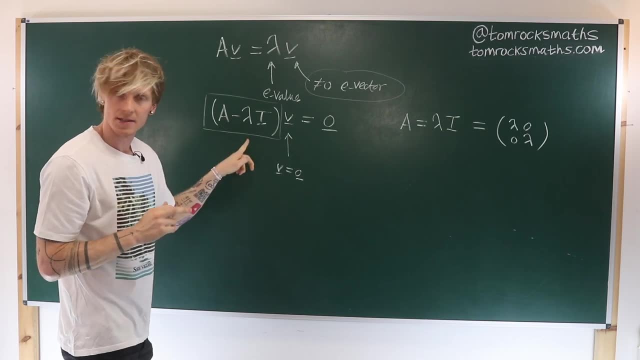 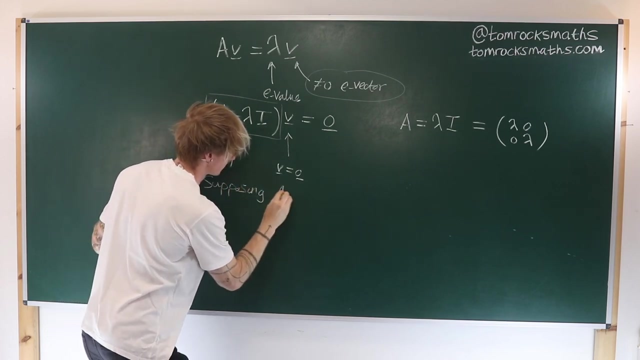 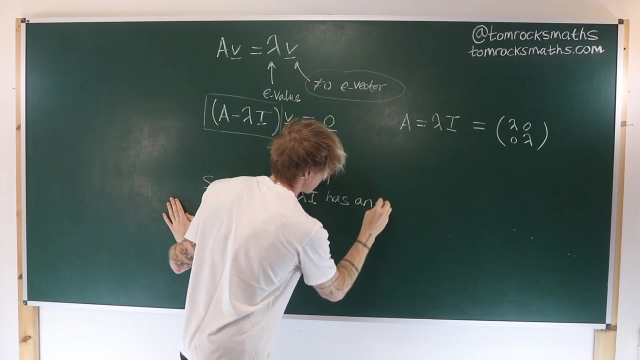 do instead is actually go back to the equation in this form and what we can say is if the inverse of this matrix exists. so if I say, supposing A minus lambda I, which is of course a matrix supposing that has an inverse, and we'll 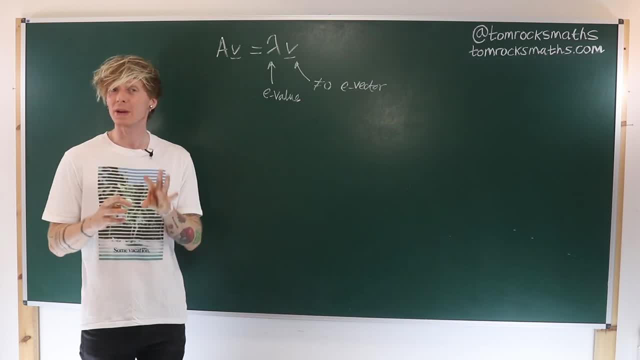 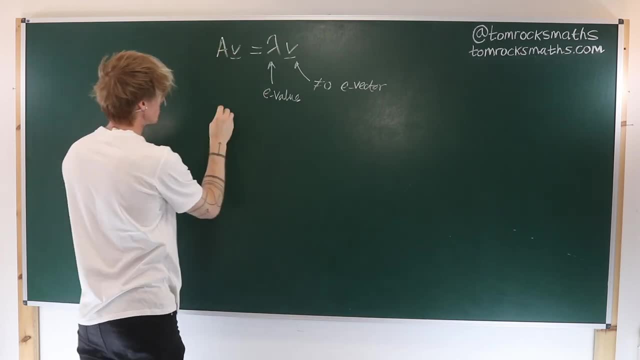 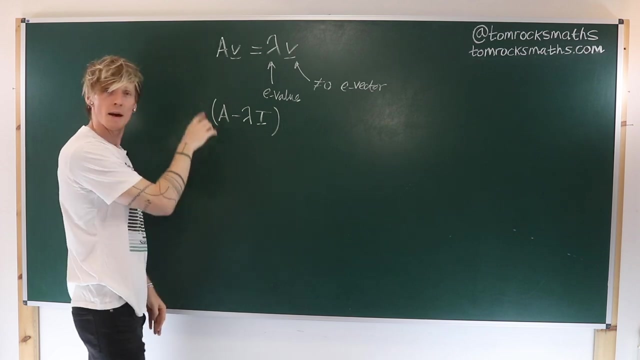 actually lies in determinants. But before we get to that we can start by rearranging the equation. So if I take this over to the left-hand side and we factor out V, then I can say A minus lambda times the identity matrix, so that A minus lambda makes sense. 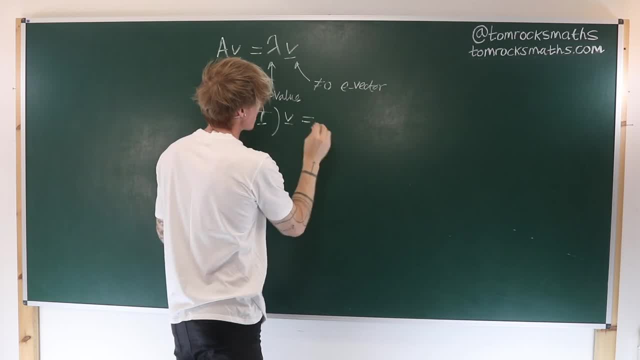 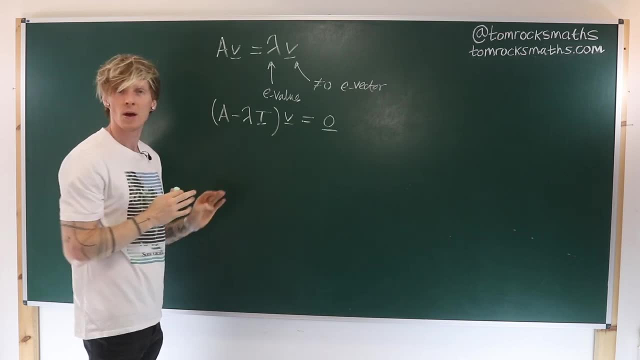 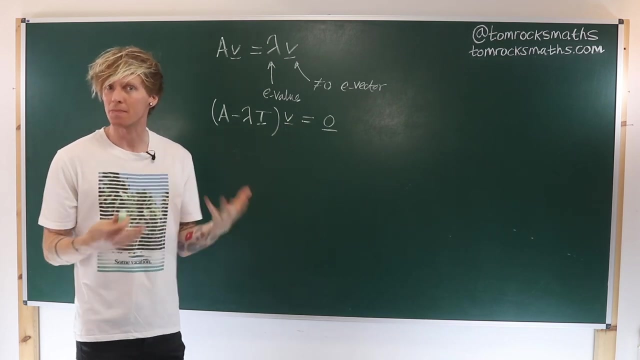 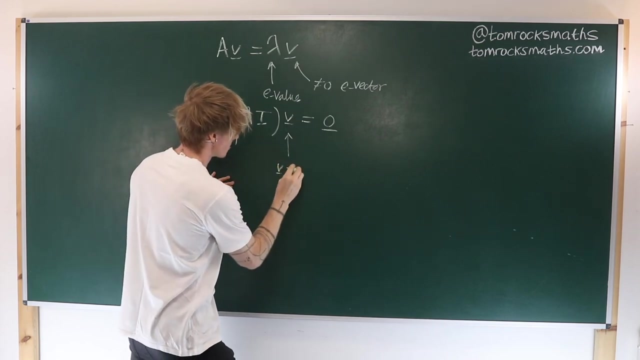 multiplied by V has to be equal to the zero vector. So now we have two terms, when multiplied together, that need to equal zero. So we can proceed in the usual manner and say: well, suppose V is zero, This is our first option, So V could be zero. and then this matrix multiplied by zero definitely gives me 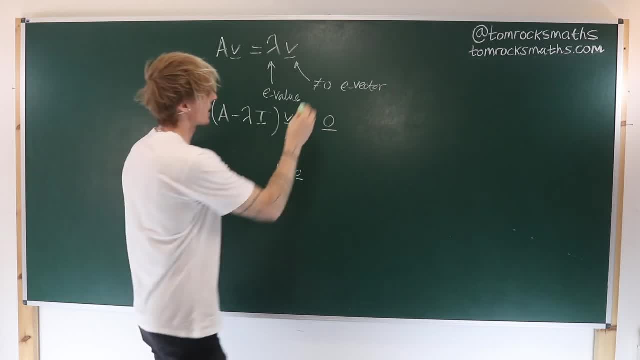 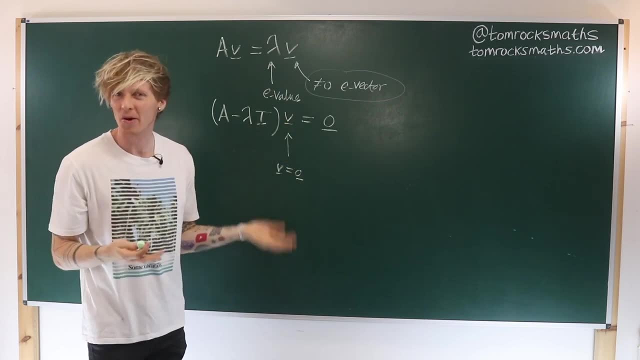 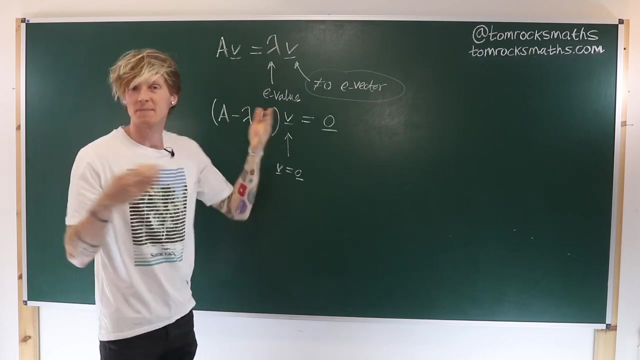 zero, And this is why we actually specify here that we want a nonzero eigenvector, Because if it's zero it's kind of boring and the whole equation is obviously true: Matrix times zero vector equals number times zero vector. They're both zero. 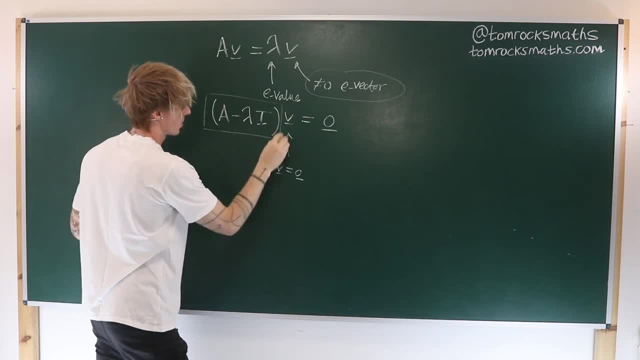 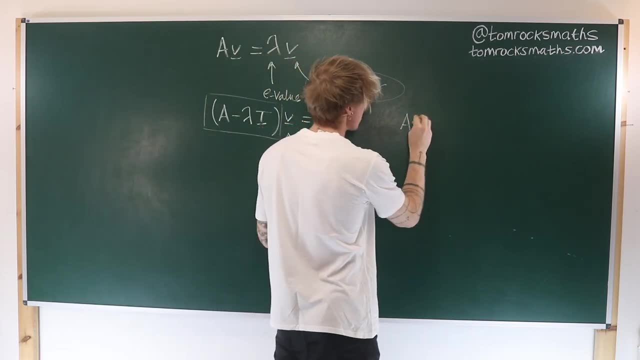 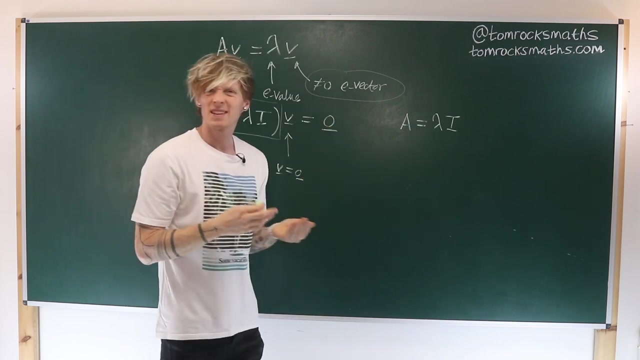 So instead we proceed by saying: we want this to be equal to zero. Now, if A minus lambda i is zero, that means our matrix A is equal to lambda times the identity matrix. but then that really limits the type of matrix A that we can actually. 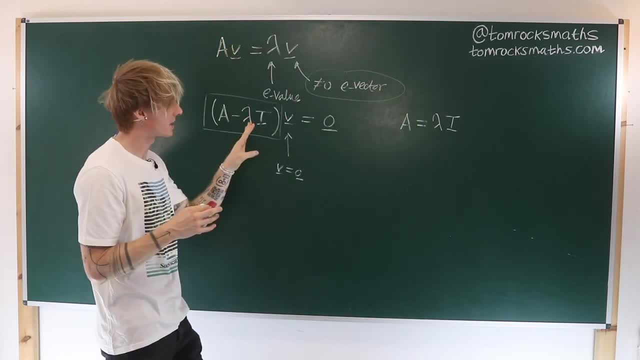 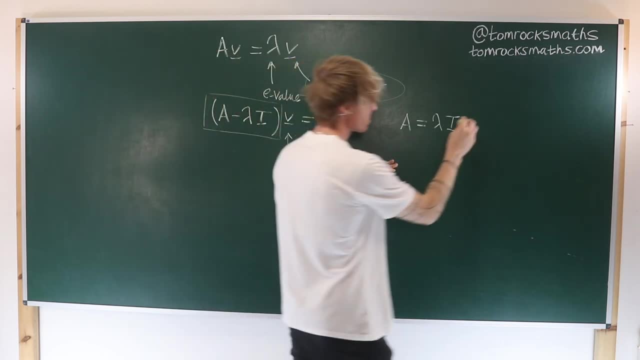 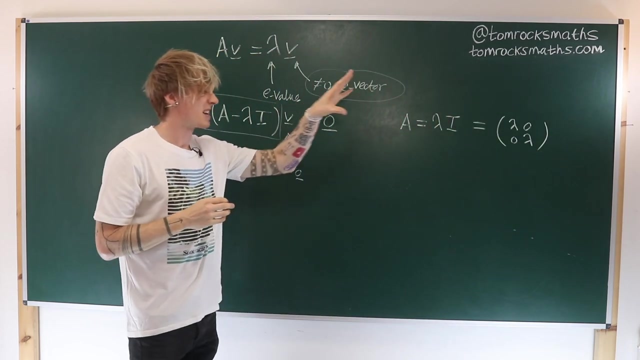 investigate Because this says. the only way this can be satisfied following this method is if A is actually just a multiple of the identity. So it would be just look like for a 2x2 case, something like this. Very boring and again not. 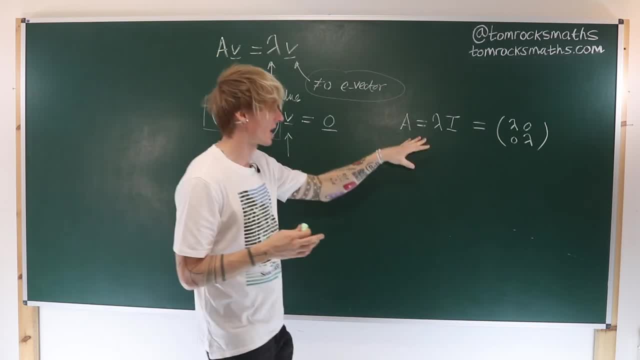 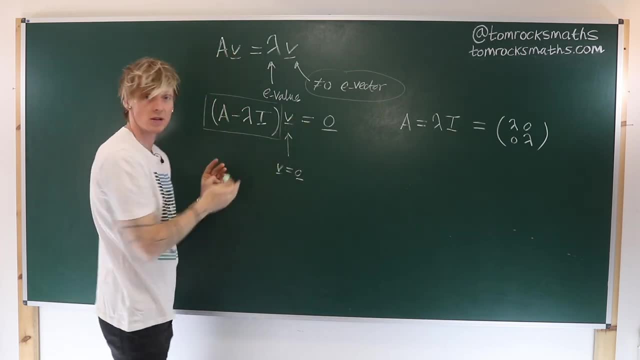 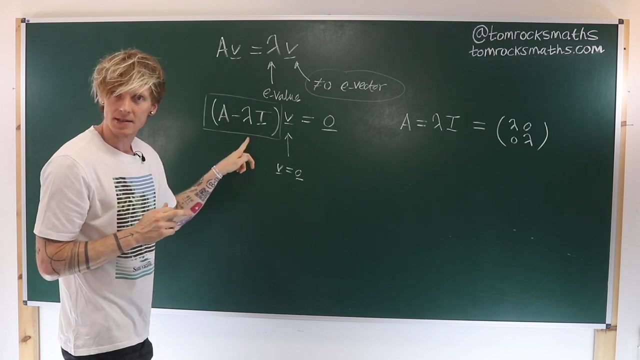 really what we're interested in. We want to look at general matrices A. So what we do instead is actually go back to the equation in this form and what we can say is if the inverse of this matrix exists. so if I say, supposing A minus. 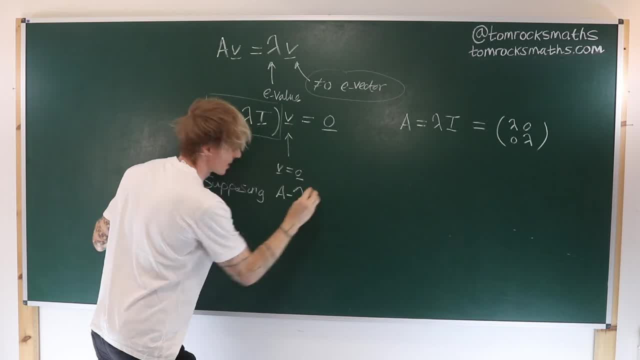 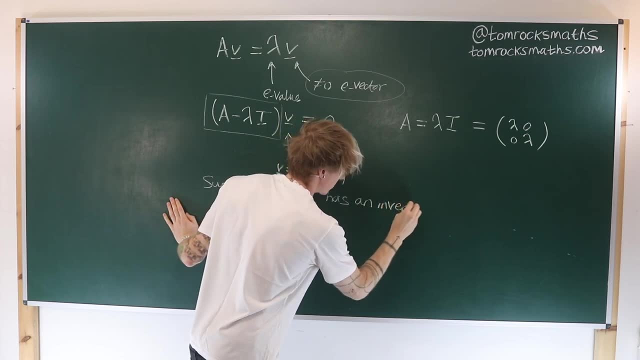 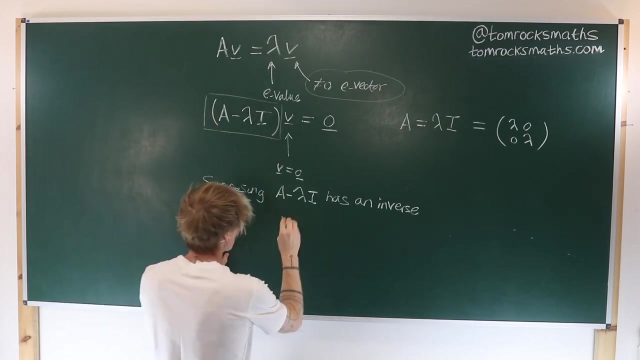 lambda I, which is of course a matrix. supposing that has an inverse- and we'll talk about the condition on that in just a moment- but supposing it has an inverse, then I can rearrange this equation and say: well, V has to be equal to. 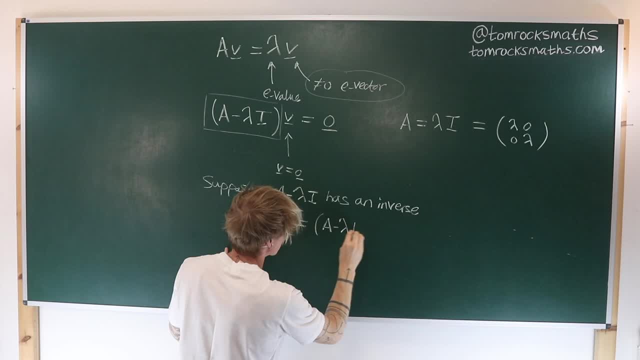 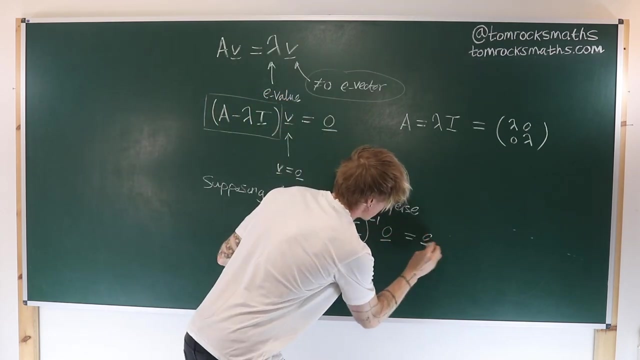 well, V has to be equal to well, V has to be equal to the inverse of A minus lambda I. so we'll put a minus 1 there to signify the inverse multiplied by 0, and now we have a matrix multiplied by 0,, so it's 0, and 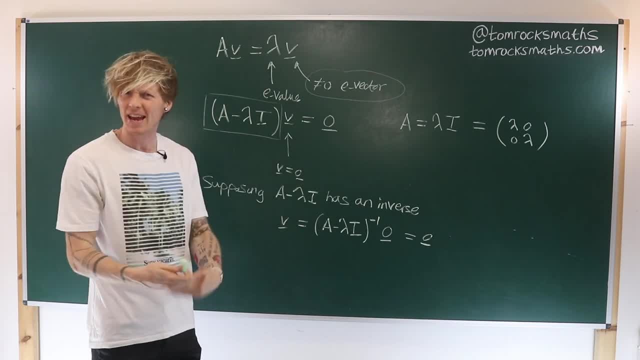 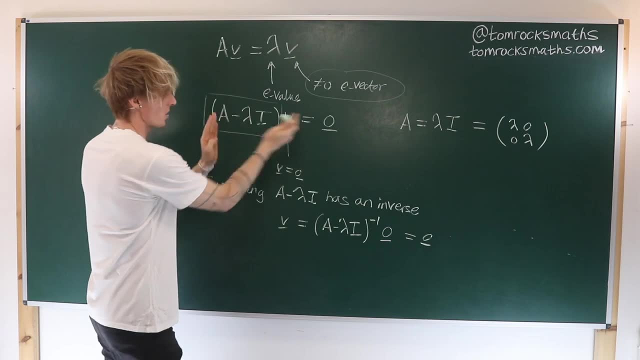 again we're back to the boring case- or the case we're not actually going to allow- of V being 0. So in both situations, from this equation here, we have two terms multiplied together to give us 0. If we follow the traditional route of two things, multiplying together equals 0,. 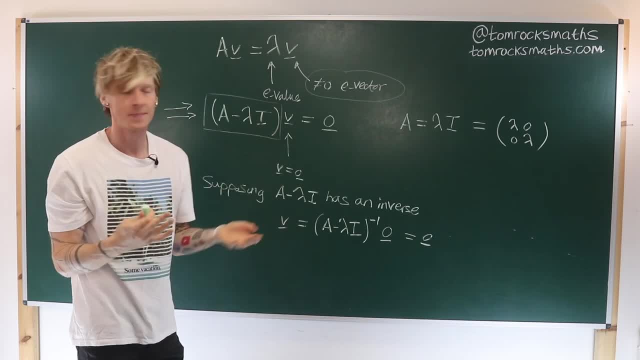 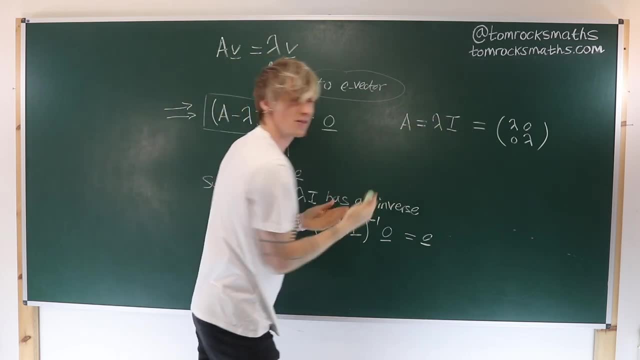 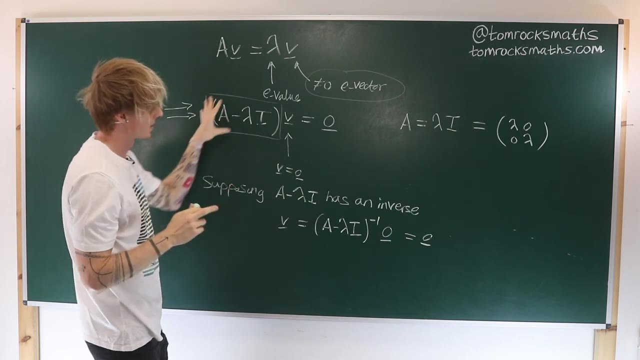 means each one of them individually could be 0. We don't want V to be 0, that's boring. And if we set A equals lambda I over here, that's also boring. So if this has an inverse, we can then multiply by 0. 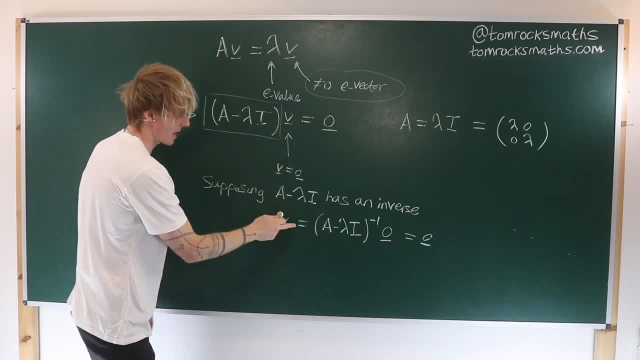 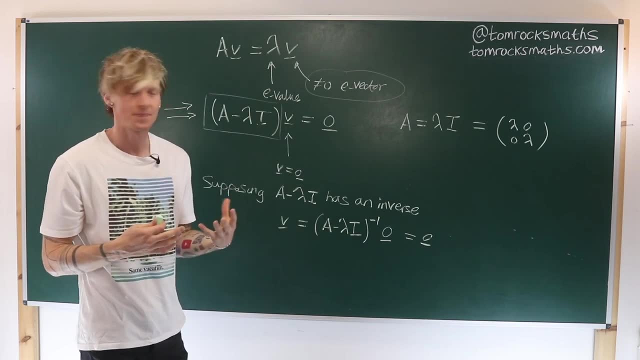 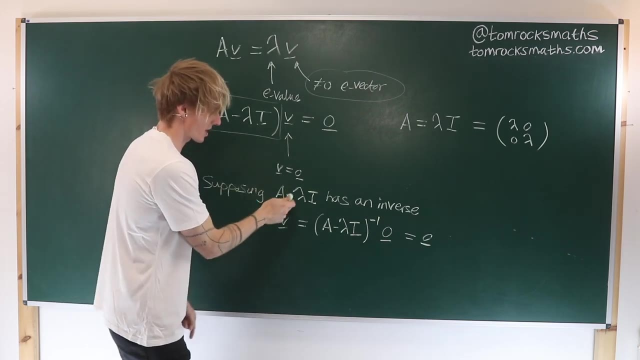 both sides by the inverse and we again get v is 0.. So the only way we can actually have something interesting, the only way we can, it turns out, find a non-zero v, is if this matrix a minus lambda. i does not have an inverse, So 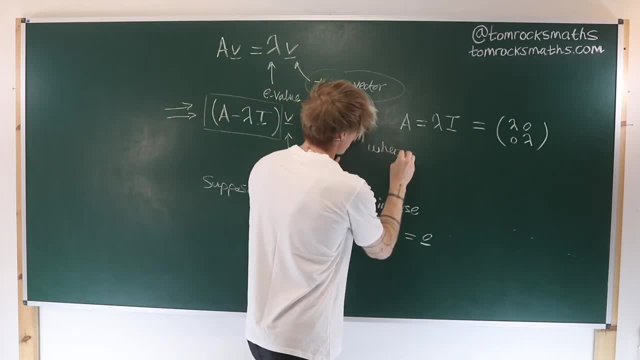 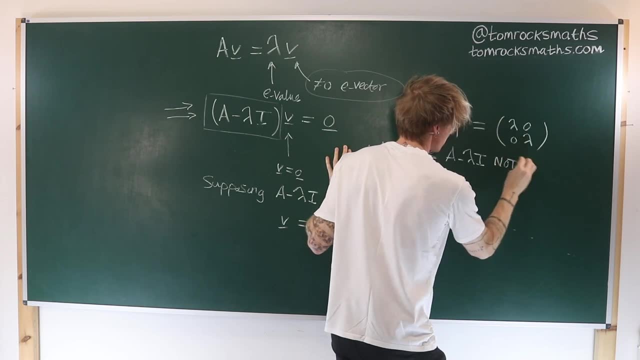 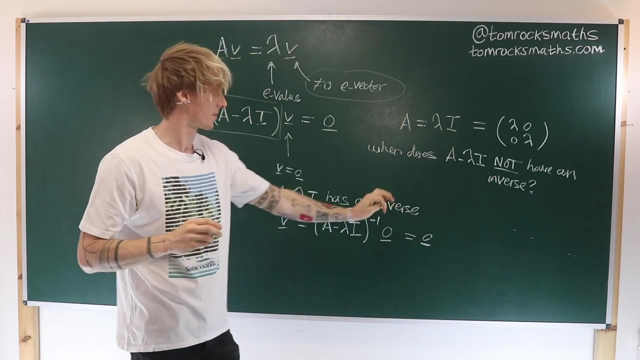 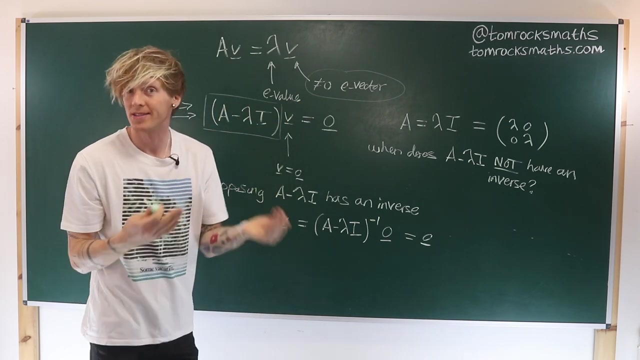 we're actually interested in answering the question: when does a minus lambda i not have an inverse? Because if it does not have an inverse, then we cannot pre-multiply by that inverse, and so therefore v is not 0. And so we actually have a chance of finding v. 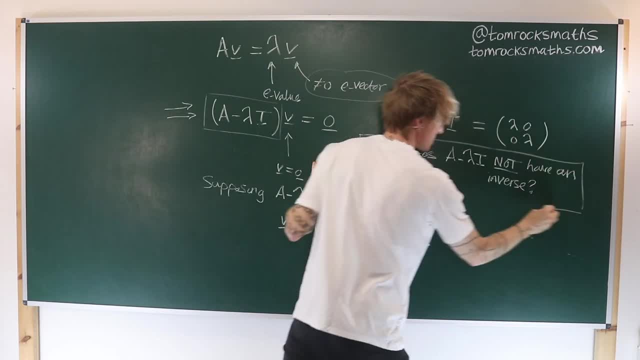 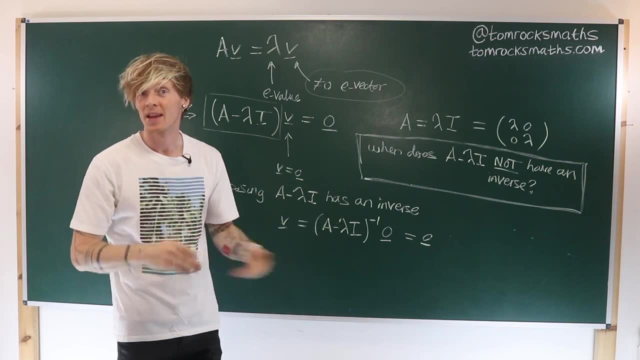 So it all comes down to who can compute this. programs has a greenES. Is there a value I biggest four? So when thischuck is positive down to this, When or what is the condition on a minus lambda i for it to not have an inverse? Now we've talked about inverse matrices in earlier videos. 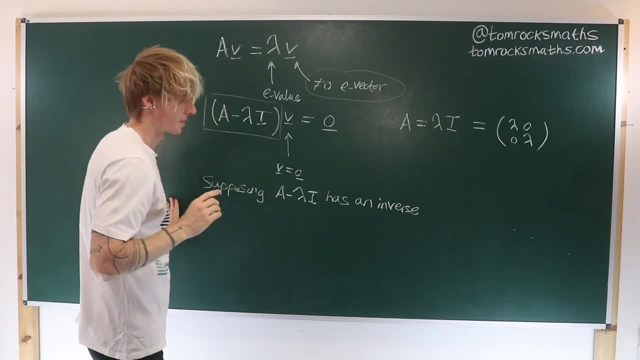 talk about the condition on that in just a moment. but supposing it has an inverse, then I can rearrange this equation and say: well, V has to be equal to well, V has to be equal to well, V has to be equal to. 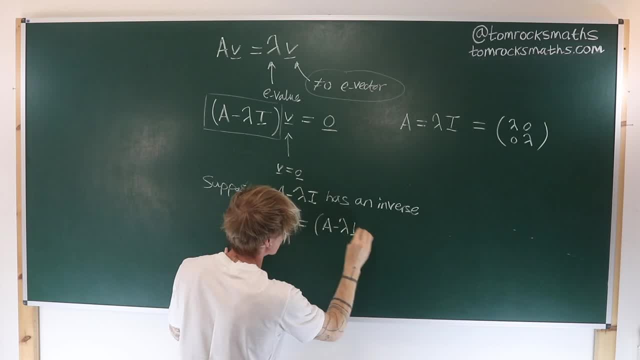 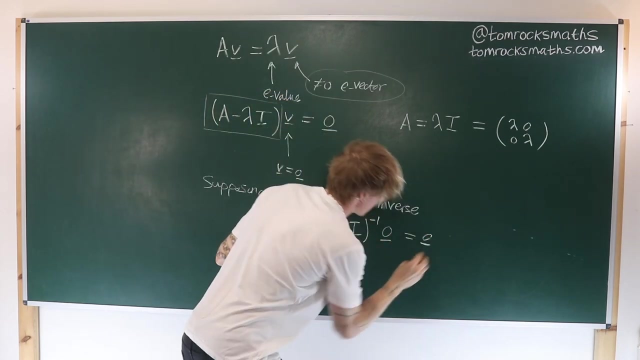 the inverse of A minus lambda I. so we'll put a minus 1 there to signify the inverse multiplied by 0, and now we have a matrix multiplied by 0, so it's 0, and again we're back to the boring case, or the case we're not actually going to. 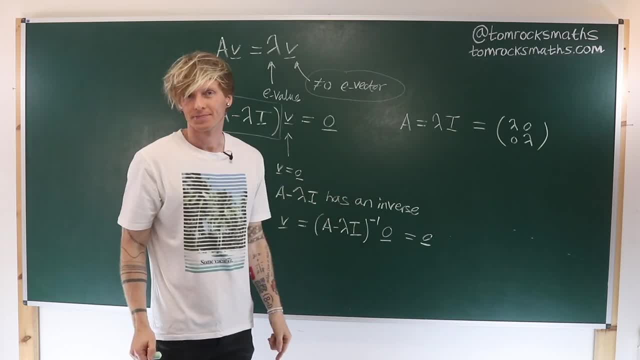 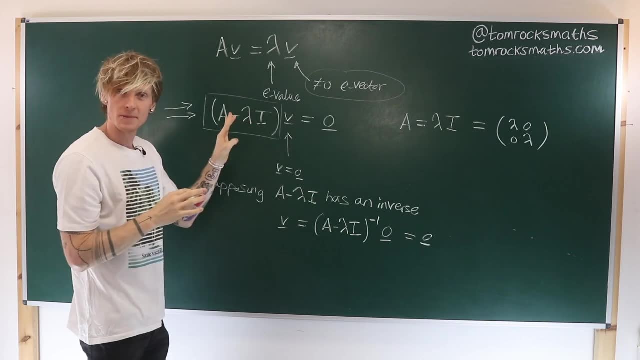 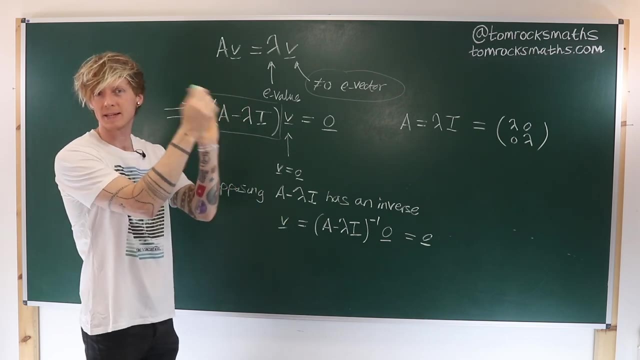 allow of V being 0. So in both situations from this equation here we have two terms multiplied together to give us 0. If we follow the traditional root of two things, multiplying together equals 0, means each one of them individually could. 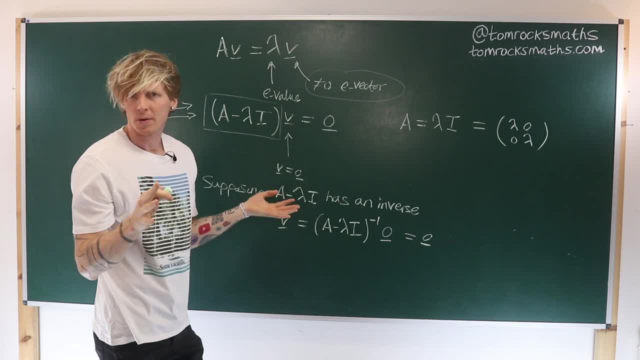 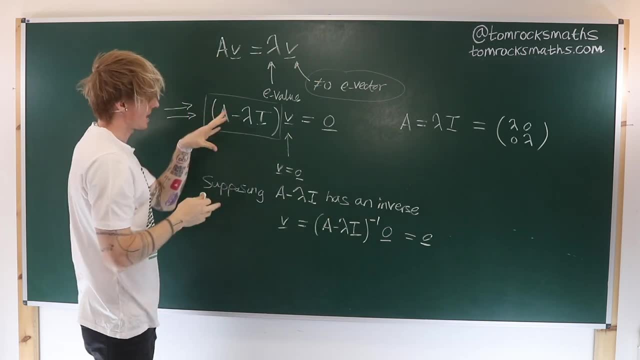 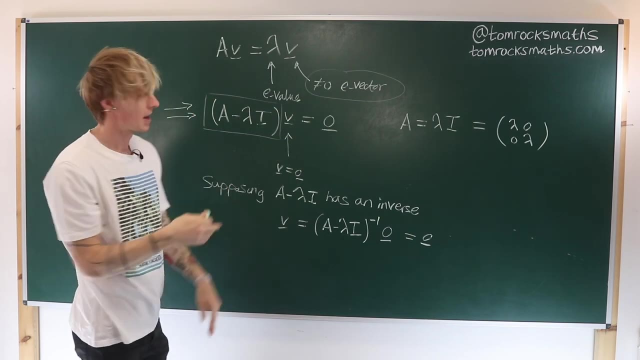 be 0. We don't want V to be 0, that's boring. and if we set A equals lambda I over here- that's also boring. So if this has an inverse, we can then multiply both sides by the inverse. 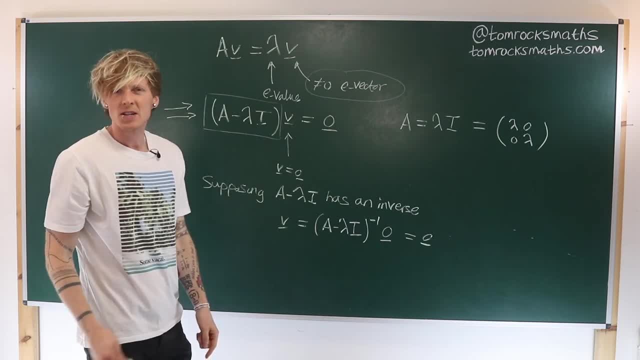 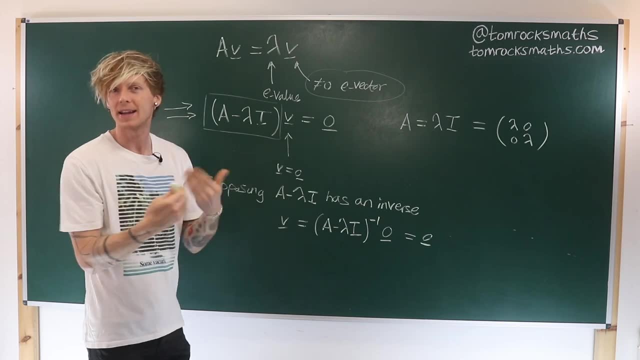 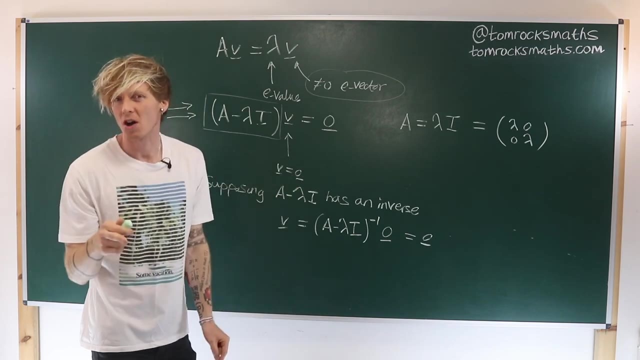 and we again get: V is zero. So the only way we can actually have something interesting, the only way we can, it turns out, find a non-zero V is if this matrix A minus lambda. I does not have an inverse. 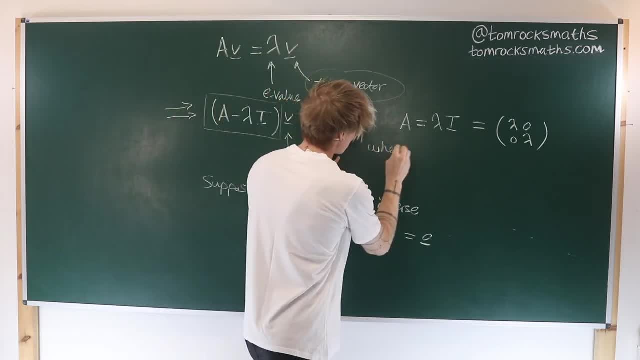 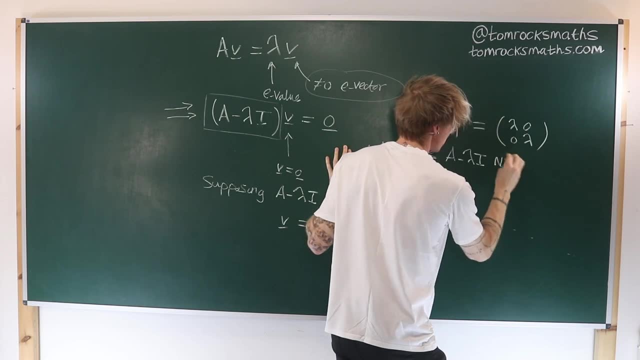 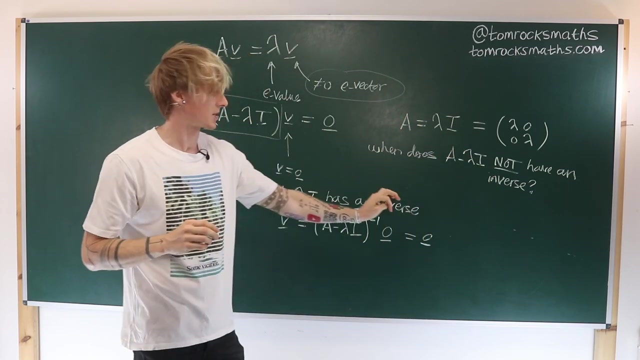 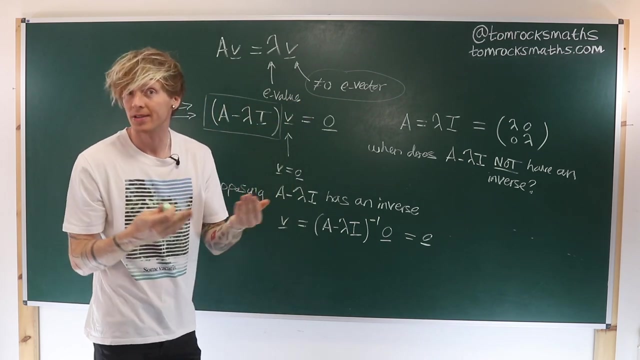 So we're actually interested in answering the question: when does A minus lambda I not have an inverse? Because if it does not have an inverse, then we cannot pre-multiply by that inverse, and so therefore V is not zero, And so we actually have a chance of finding V. 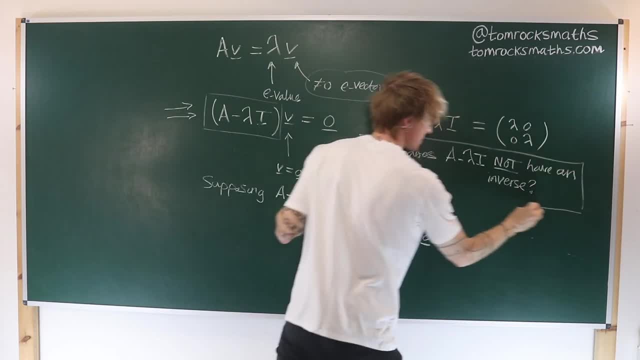 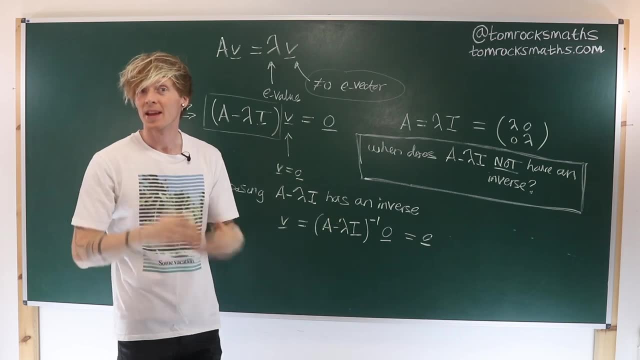 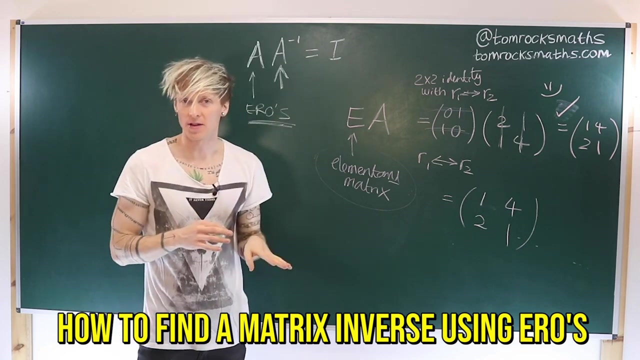 So it all comes down to this: when or what is the condition on A minus lambda? I for it to not have an inverse. Now we've talked about inverse matrices in earlier videos in the Oxford Linear Algebra series and we actually saw the condition to not have an inverse. 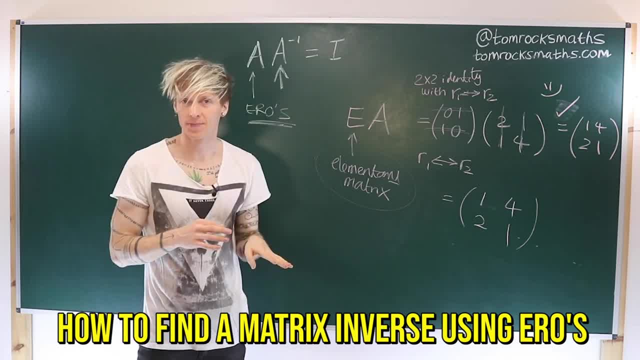 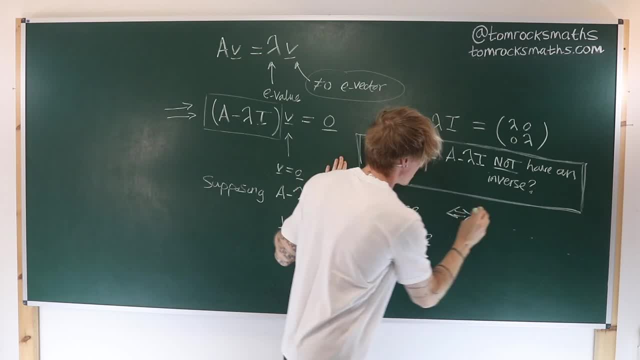 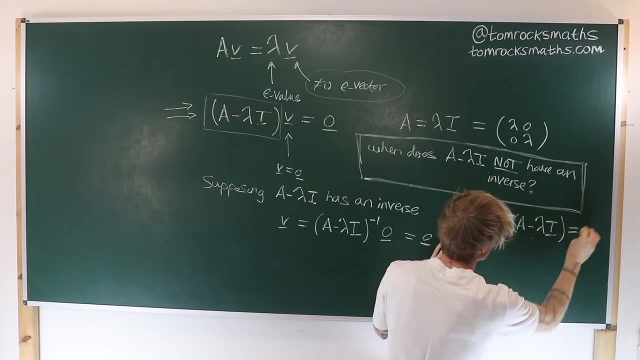 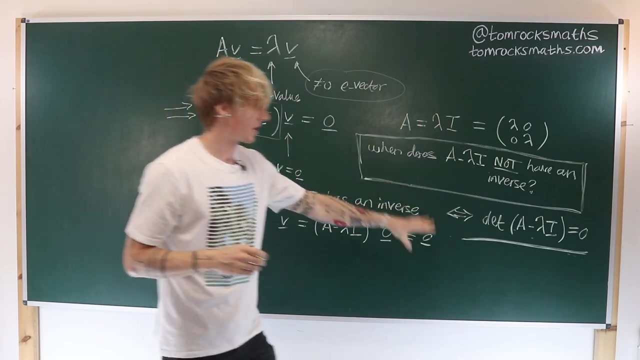 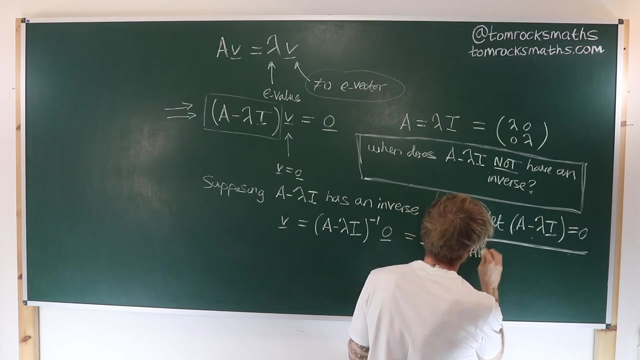 in the Oxford linear algebra series and we actually saw the condition to not have an inverse is exactly when the determinant of a minus lambda i is equal to zero. So this is the equation that we actually solve to find the eigenvalues lambda, and this is called the characteristic equation. So just to 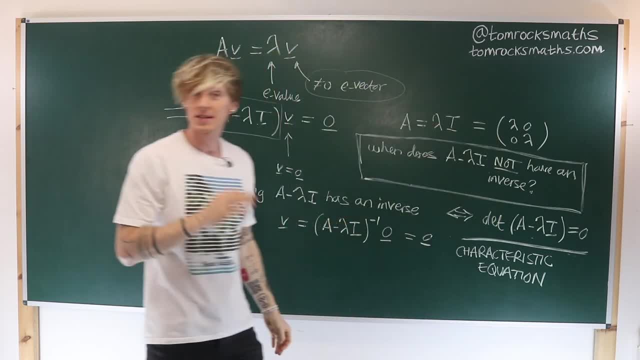 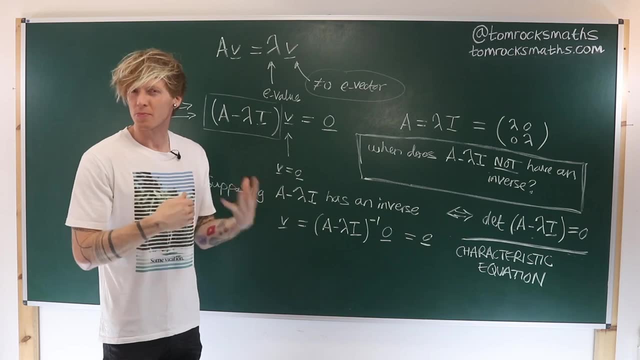 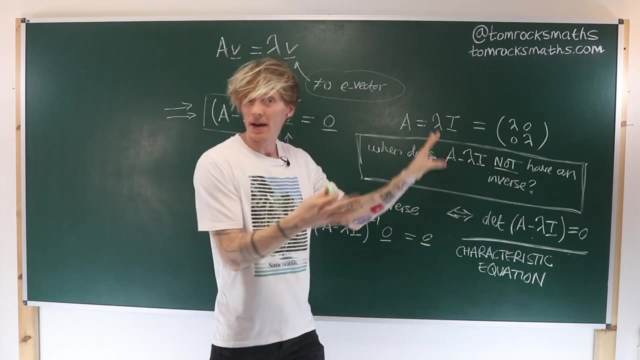 recap: we solve the determinant of a minus lambda i equal to zero. That will give us an algebraic equation for lambda. it will give us a polynomial in lambda. we solve: find those roots to get lambda, the different possible eigenvalues. So this: 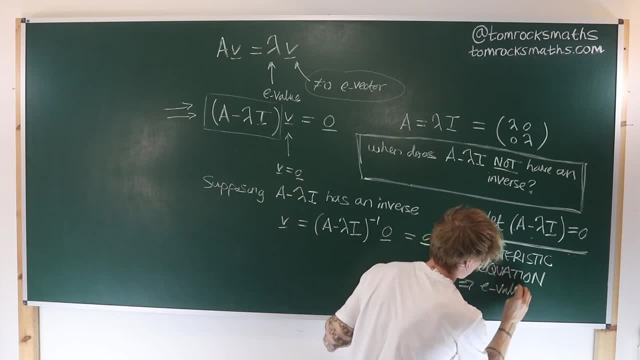 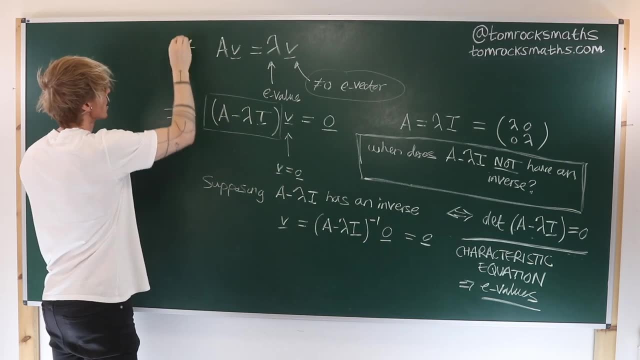 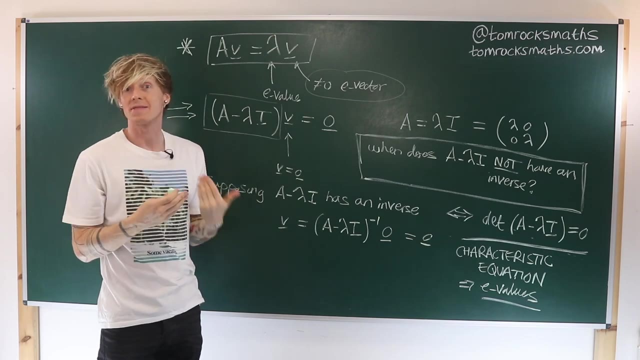 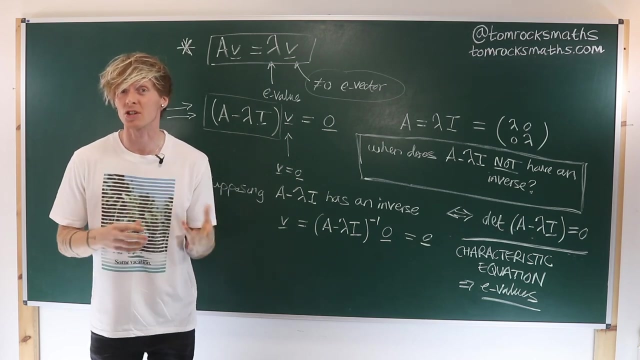 gives us the eigenvalues, and once we have the eigenvalues lambda, we go back to our equation at the top. here we substitute in for lambda and then we can solve for our eigenvector v. Now, before we go through some examples together, I do recommend checking out the video lectures on this topic from: 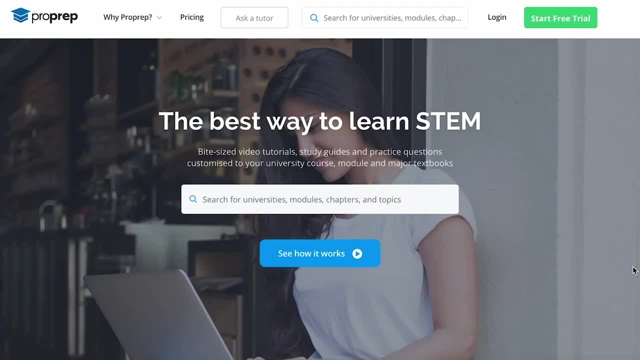 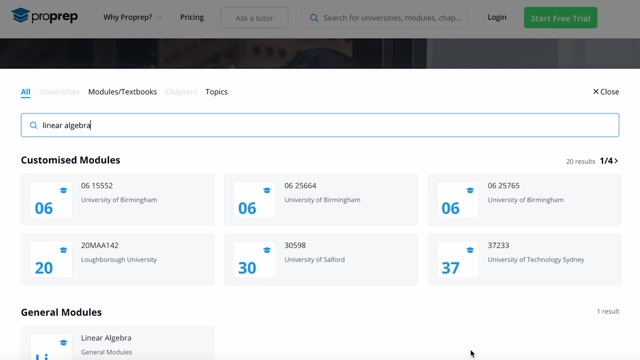 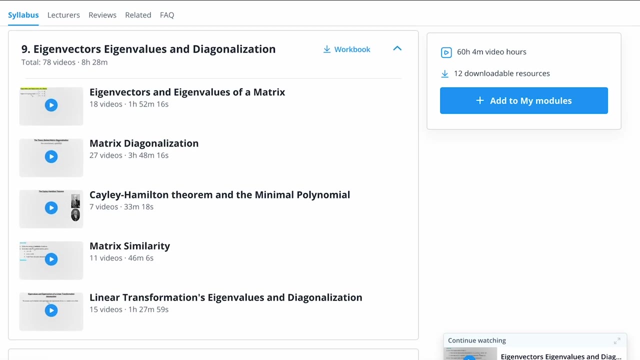 ProPrep, which are linked in the video description. ProPrep is an online resource that provides customized tutorials for students looking to improve their skills in stem-based subjects. There is almost two hours of content looking at eigenvalues and eigenvectors, which will really help you. 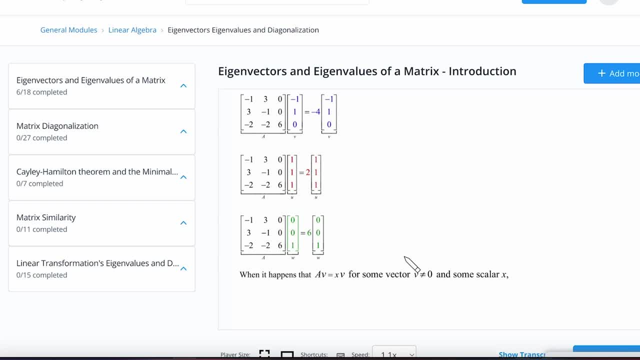 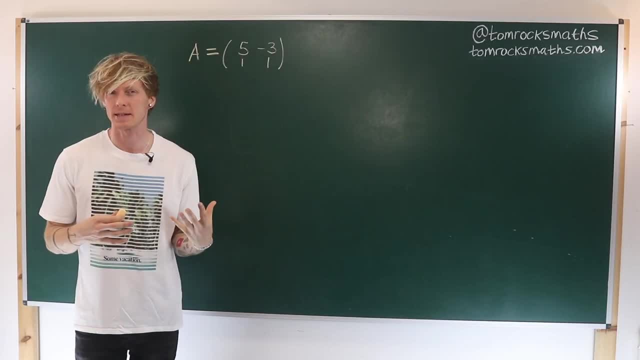 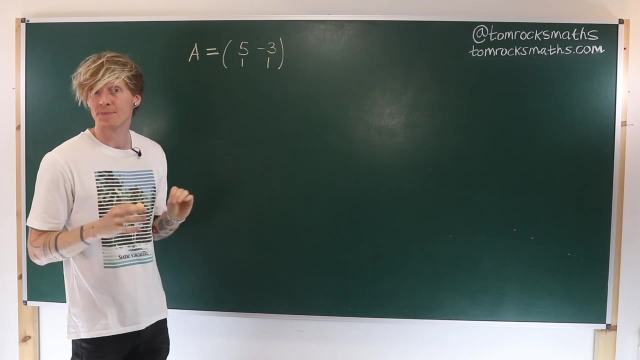 to understand the topic. You can access the videos by signing up for a free trial using the link below. Let's look at an example to see how this works in practice. Suppose I want to find the eigenvalues and eigenvectors of this two-by-two matrix A, So we want to solve the equation. 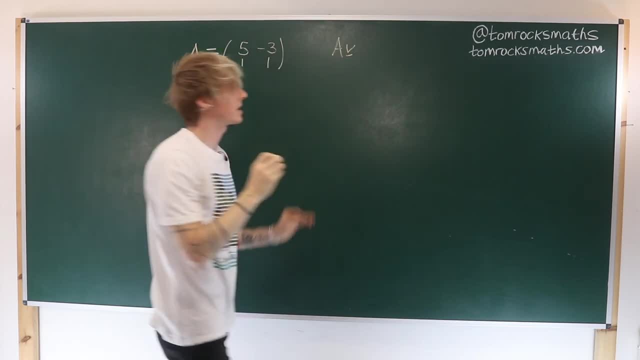 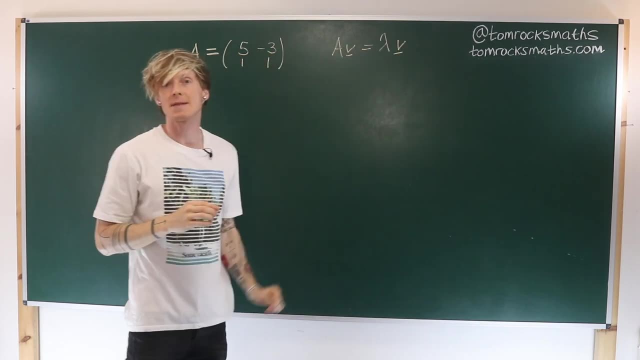 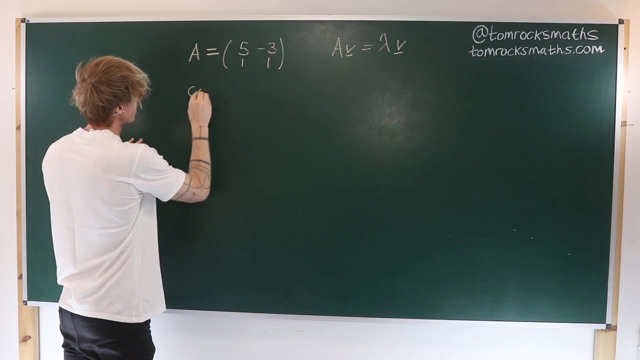 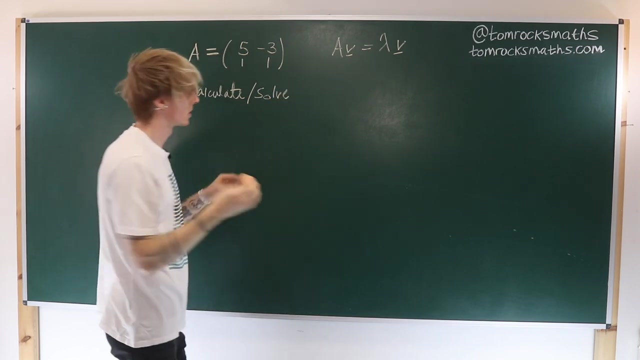 A times a non-zero vector. v is equal to a scalar lambda, which is the eigenvalue times the same non-zero vector. Now our approach, as we've just seen, is to calculate or solve the characteristic polynomial which is the determinant of. 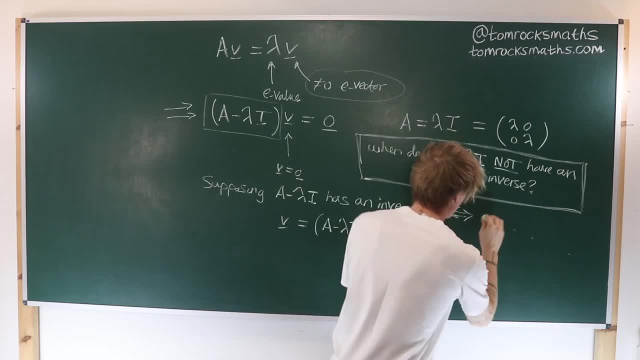 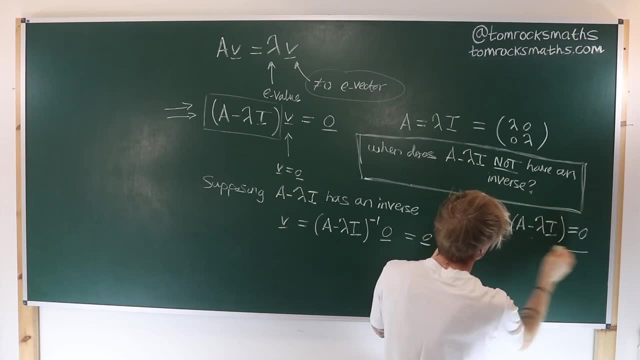 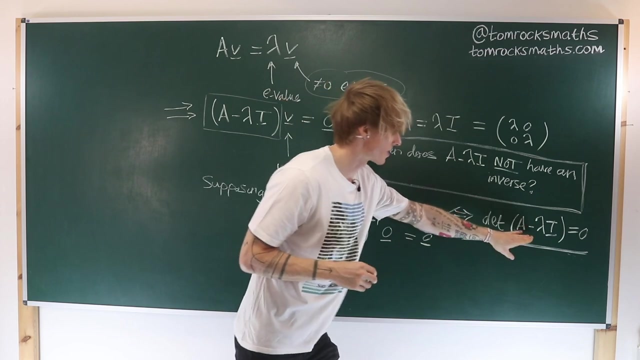 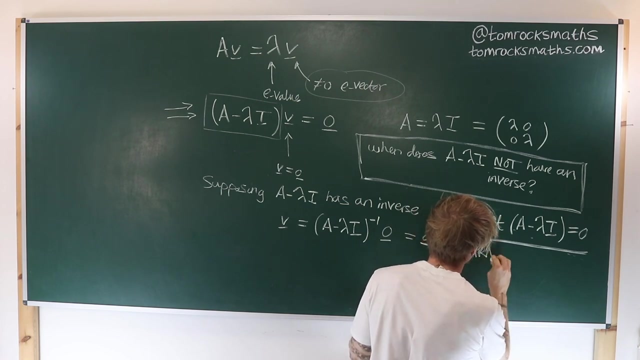 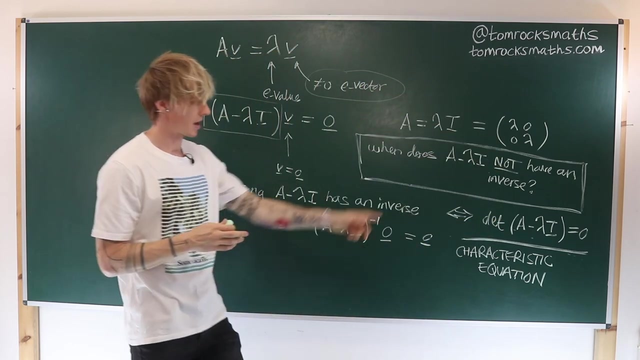 is exactly when the determinant of A minus lambda I is equal to zero. So this is the equation that we actually solve to find the eigenvalues lambda, And this is called the characteristic equation. So, just to recap, we solve the determinant of a minus lambda I. 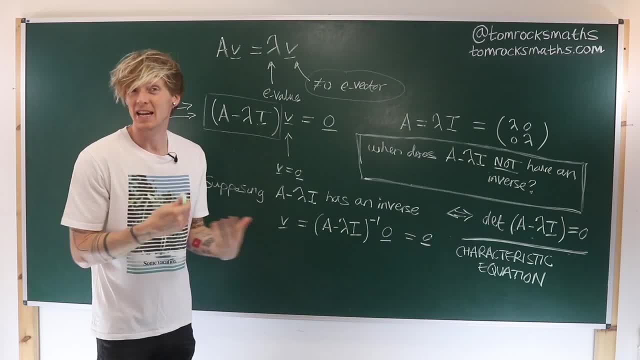 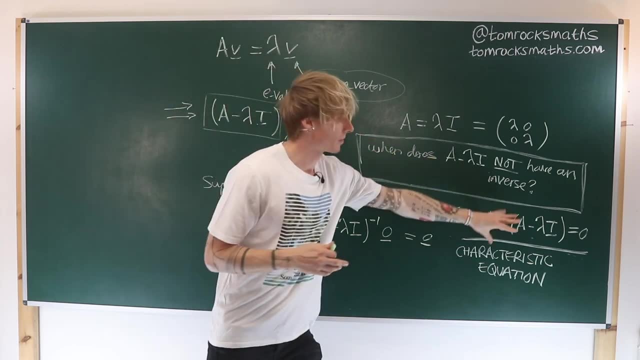 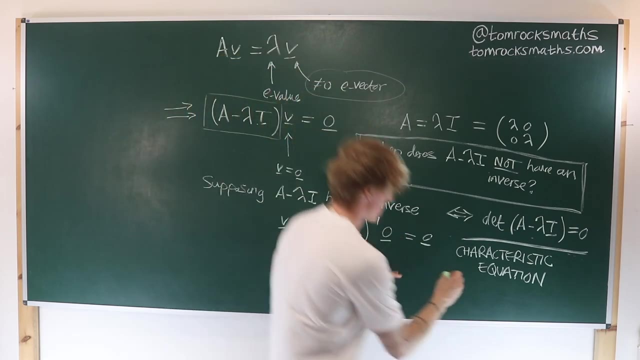 equal to zero. That will give us an algebraic equation for lambda. It will give us a polynomial in lambda. That will give us a polynomial in lambda We solve, find those roots to get lambda the different possible eigenvalues. So this gives us the eigenvalues. 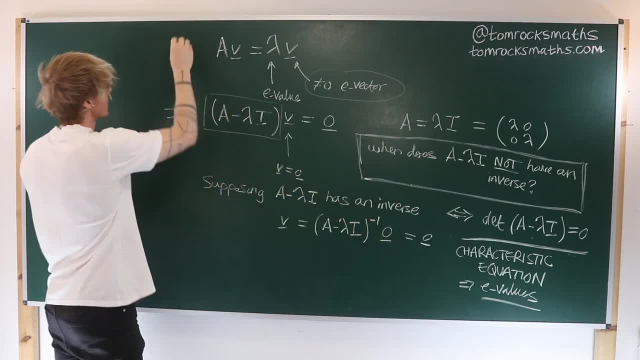 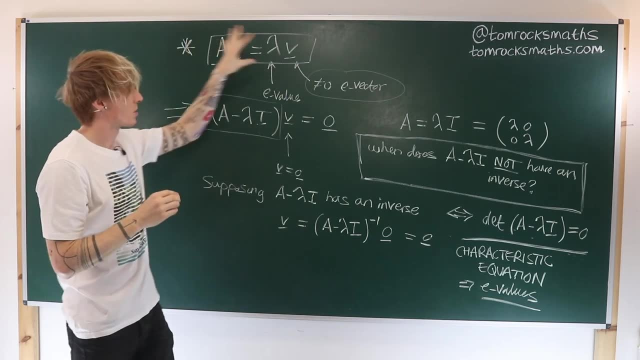 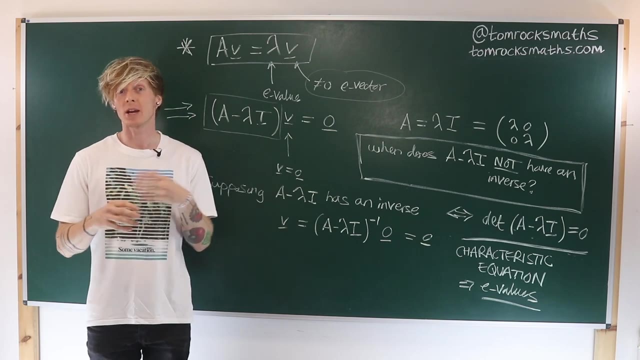 and once we have the eigenvalues lambda, we go back to our equation at the top. here we substitute in for lambda and then we can solve for our eigenvector v. Now, before we go through some examples together, I do recommend checking out the video lectures. 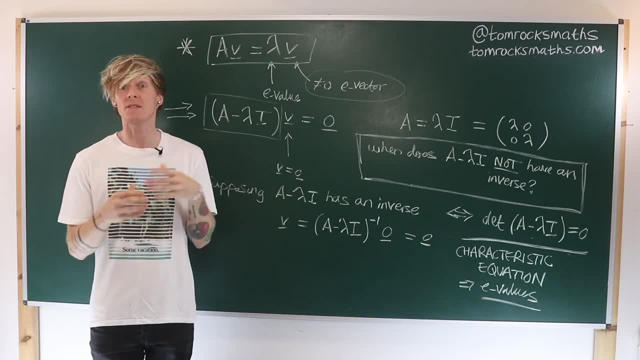 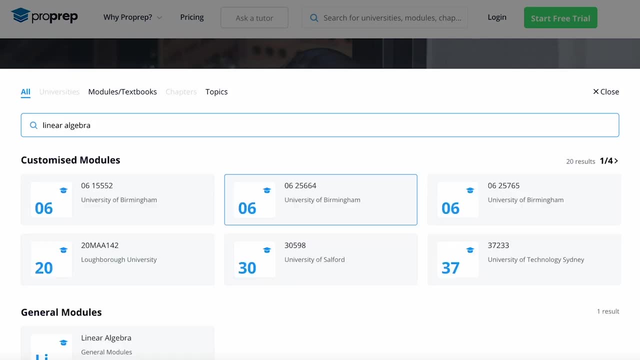 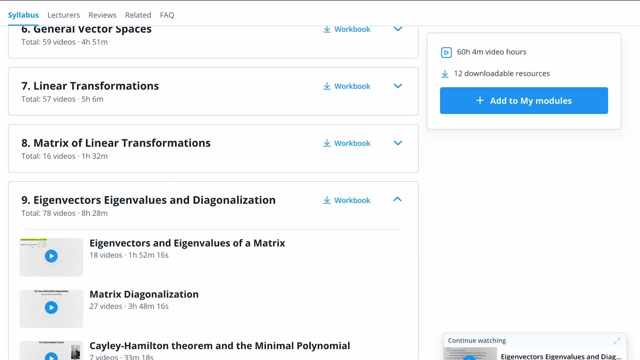 on this topic from ProPrep, which are linked in the video description. ProPrep is an online resource that provides customised tutorials for students looking to improve their skills in STEM-based subjects. There is almost two hours of content looking at eigenvalues and eigenvectors. 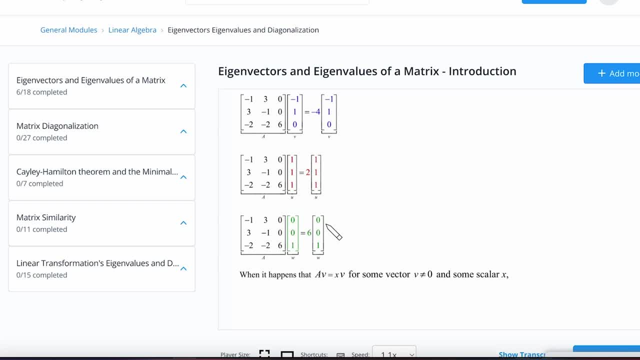 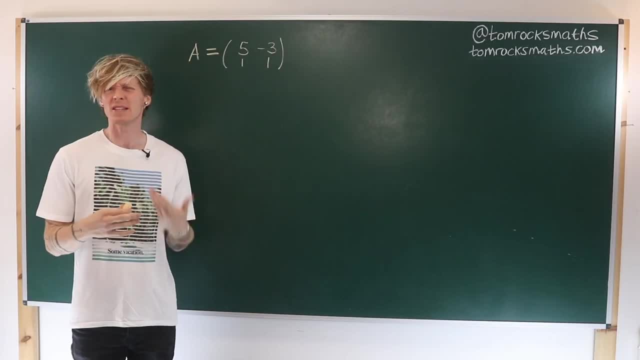 which will really help you to understand the topic. You can access the videos by signing up for a free video on the ProPrep website, which is linked in the video description Trial, using the link below. Let's look at an example to see how this works in practice. 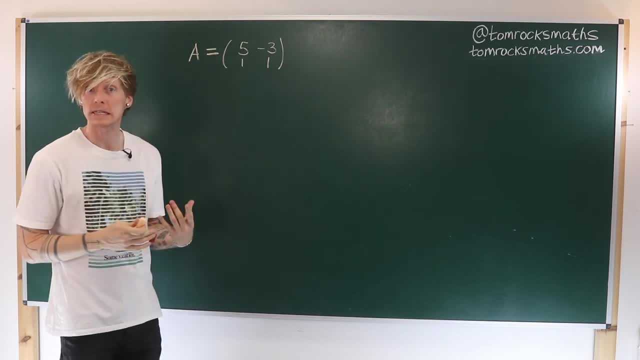 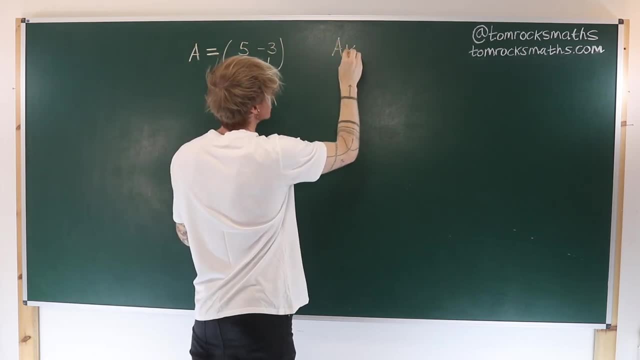 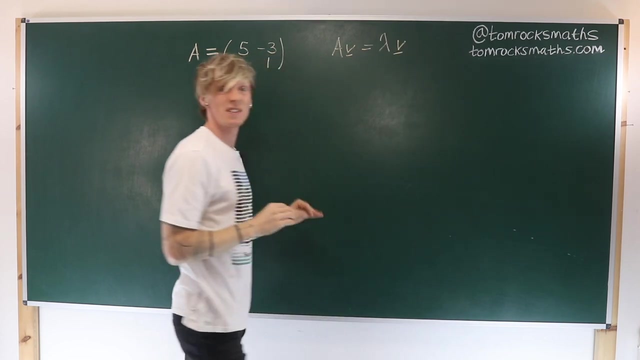 Suppose I want to find the eigenvalues and eigenvectors of this 2x2 matrix A. So we want to solve the equation: A times a non-zero vector, v is equal to a scalar lambda, which is the eigenvalue times the same non-zero vector. 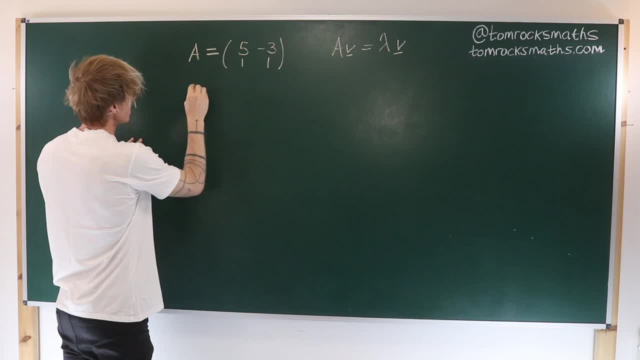 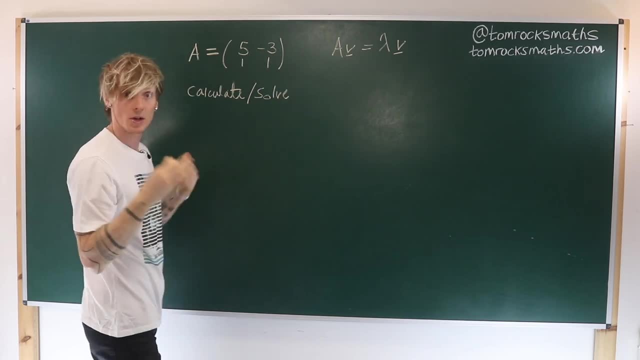 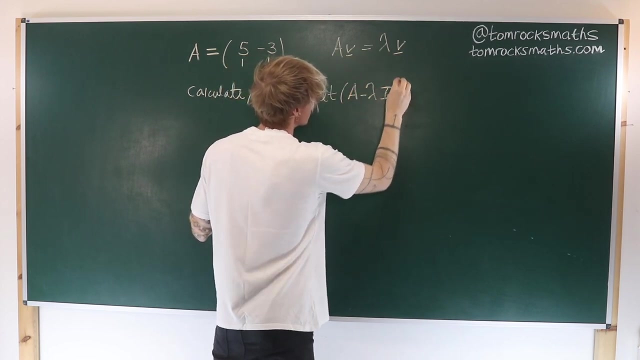 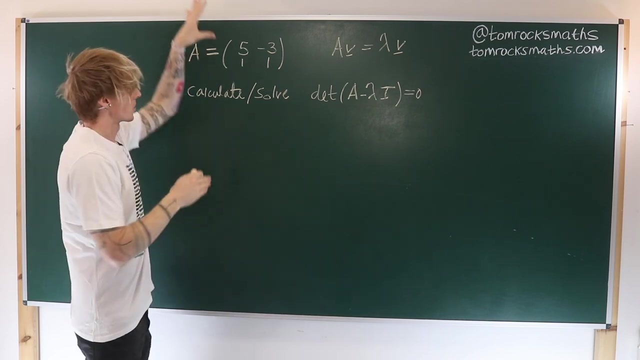 Now our approach, as we've just seen, is to calculate or solve the characteristic polynomial which is the determinant of A minus lambda i is equal to zero. So here we have a 2x2 matrix. so lambda times the 2x2 identity will give me. 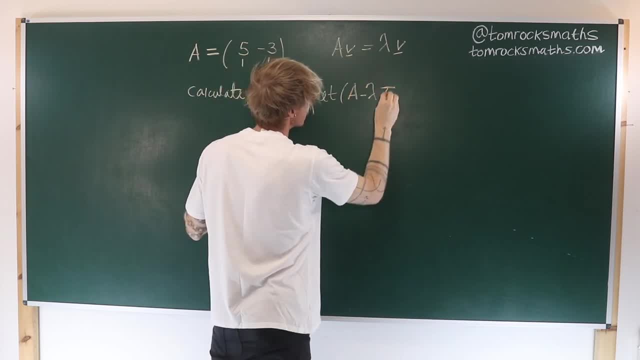 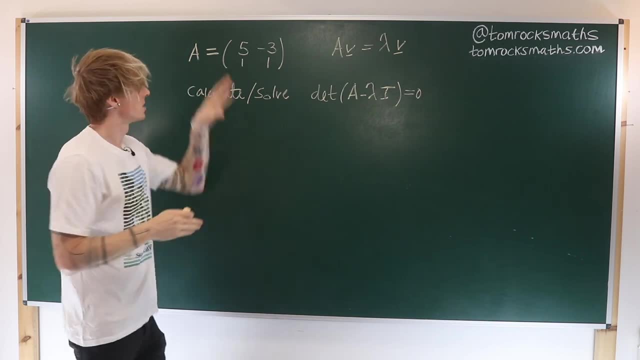 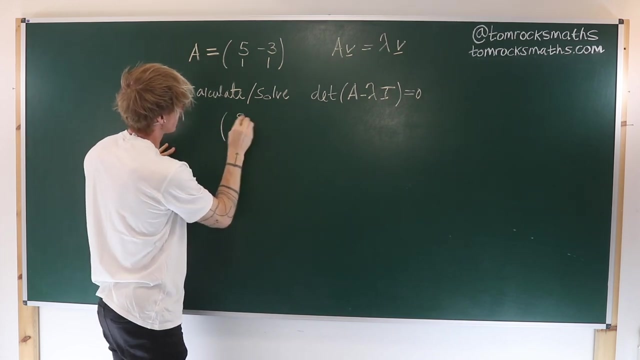 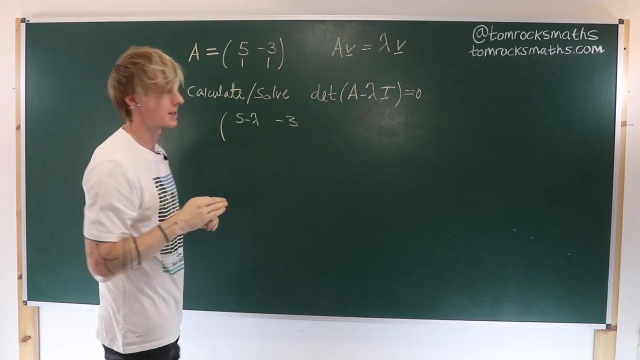 A minus lambda, i is equal to zero. So here we have a two-by-two matrix. So lambda times the two-by-two identity will give me five minus lambda in that first entry, minus three because there's a zero in the identity matrix there. That stays as one. 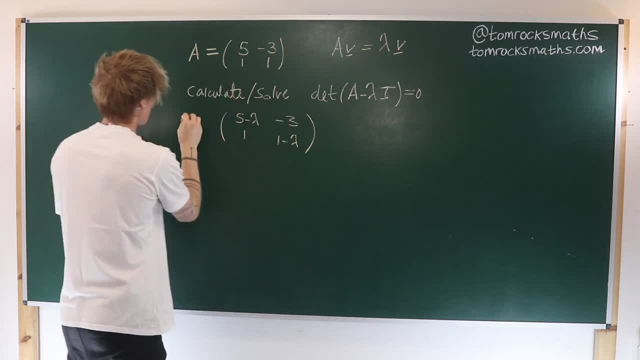 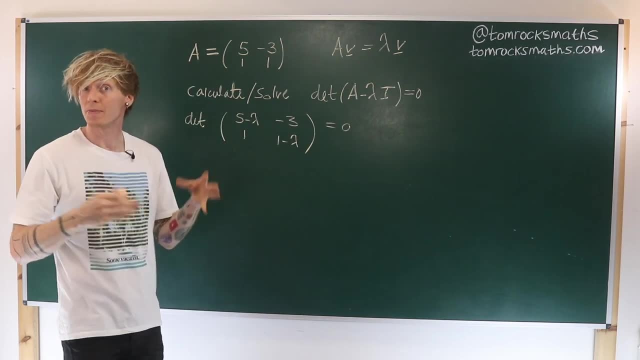 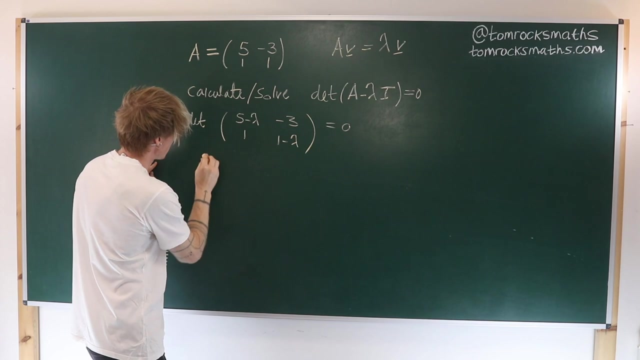 and then this becomes one minus lambda, and we want the determinant of this to be to be equal to zero. Now, this is a two-by-two matrix. The determinant is just the diagonal ones minus the off-diagonal product. So we can say that's equivalent to 5 minus lambda times 1 minus lambda minus minus. 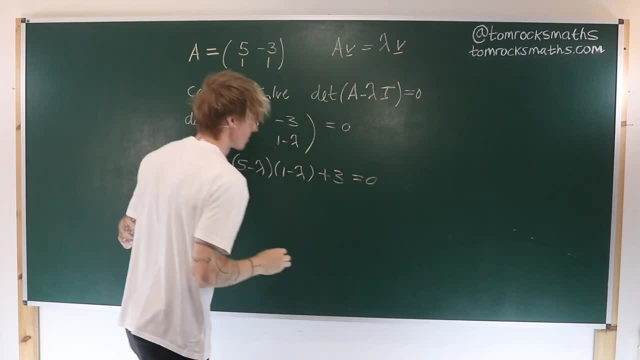 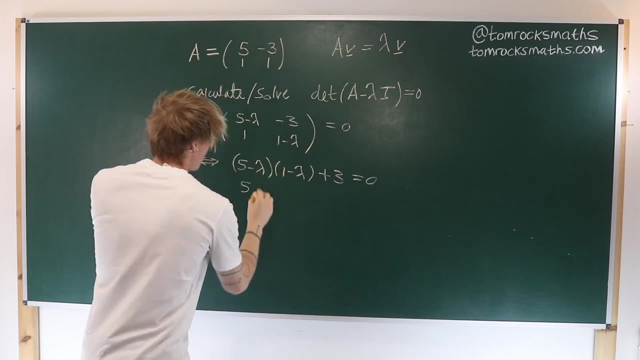 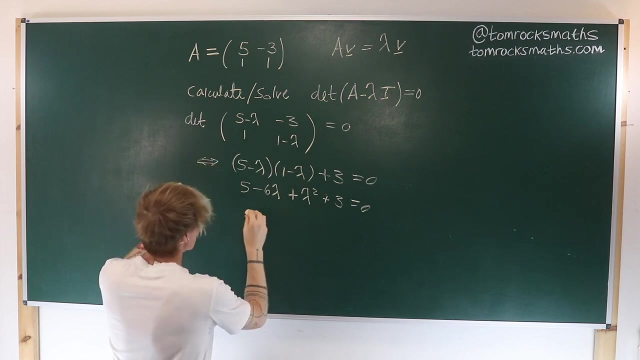 three. so plus three equal to zero. So gonna need to expand this bracket which gives us 5 minus lambda, minus another five lambda minus six lambda. so five lambda lambda plus lambda squared plus three equals zero, so that becomes lambda squared minus six lambda. 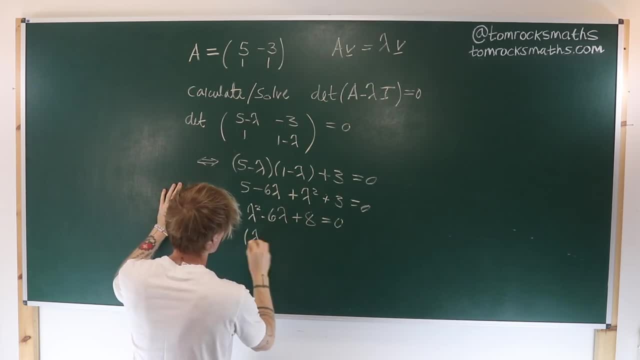 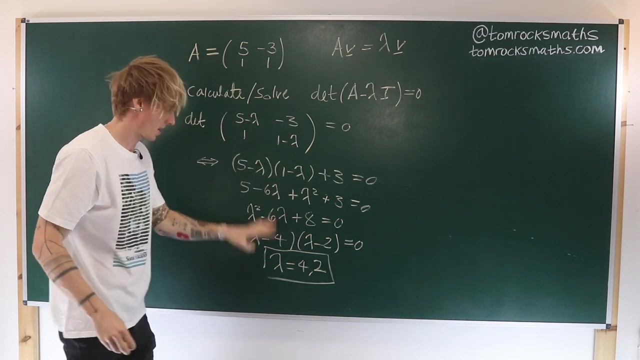 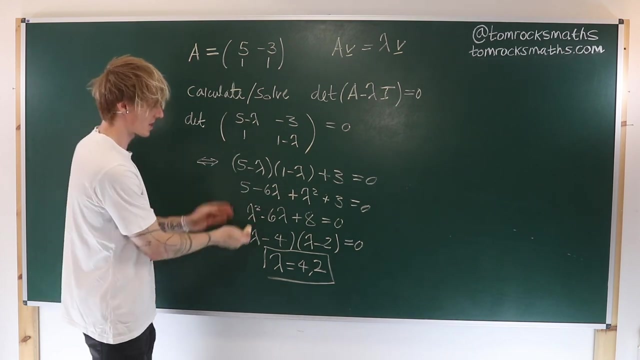 plus eight is zero, and that factorizes really nicely into lambda minus four. lambda minus two equals zero, so lambda is four or two. So our eigenvalues here are lambda equals four and lambda equals two. Now just to say for this step here I was able to spot that this factorizes: 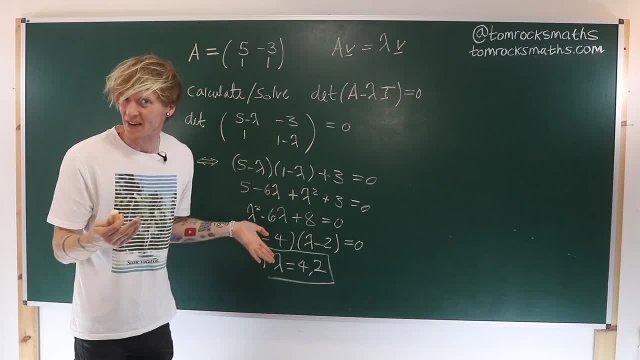 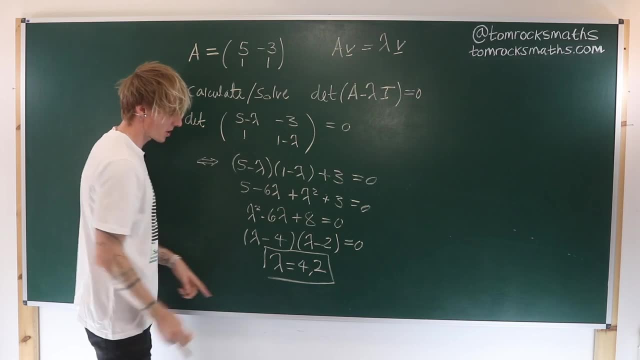 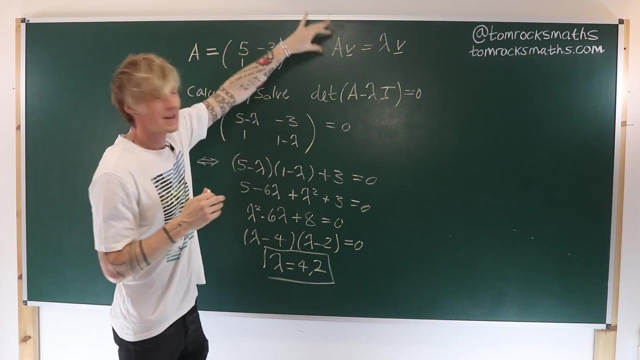 really nicely. Of course they won't always factorize and you can use the quadratic equation here to solve for your roots. lambda, We now know the eigenvalues are four and two, so, following our method, we now have to plug them in to our equation to actually find the eigenvector. v And that is theнаружive1 أところ. so jetzt elevated yところ and I get some room before I get to the 취 shrimpneam times that. So we now know the eigenvalues are four and two. So, following our method, we now have to plug them in to our equation to actually find the eigenvector v and 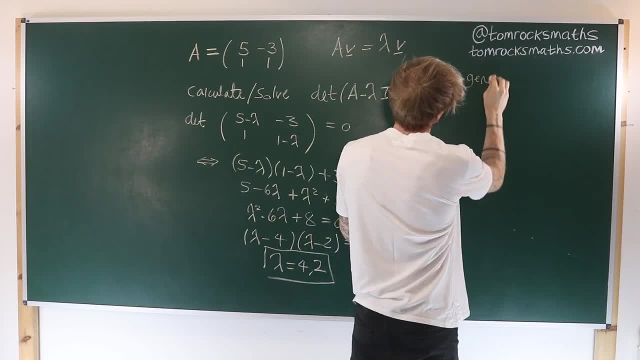 So, following our method, we now have to plug them in to our equation to actually find the eigenvector v, and- And here we're considering a general v, which has to be 2d, so v here is going to be x, y. 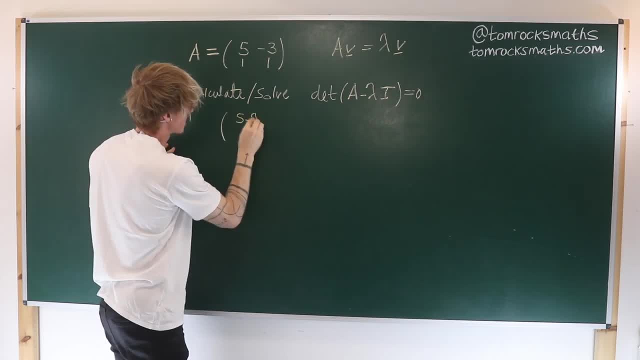 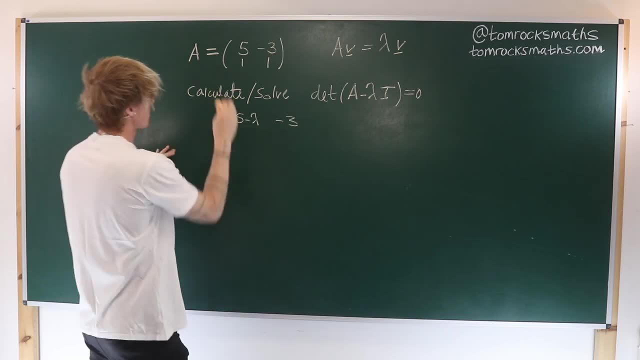 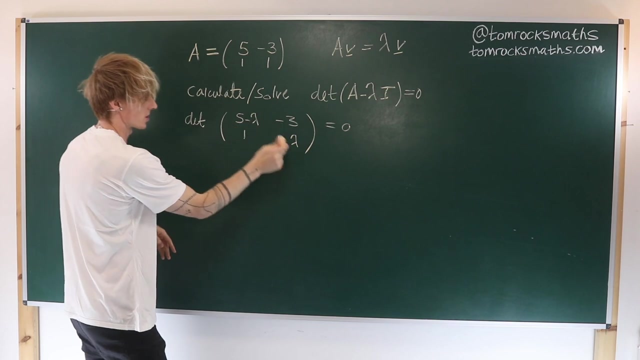 5 minus lambda in that first entry, minus 3, because there's a zero in the identity matrix there. that stays as 1, and then this becomes 1 minus lambda and we want the determinant of this to be equal to zero. Now this is a 2x2 matrix. the determinant is just the diagonal ones minus. 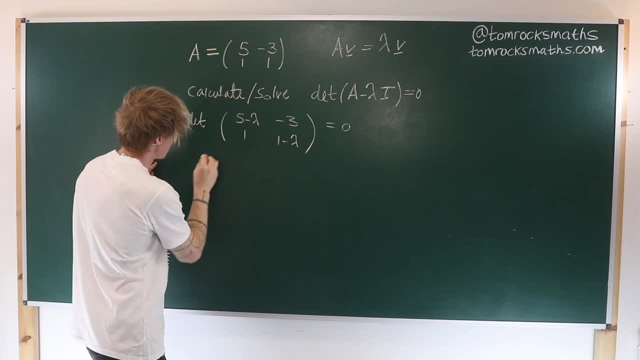 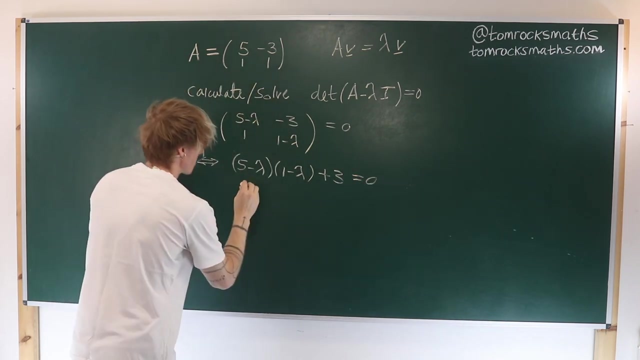 the off-diagonal product. so we can say that's equivalent to 5 minus lambda times 1 minus lambda minus minus 3, so plus 3, equal to zero. So we're going to need to expand this bracket which gives us 5 minus lambda minus another 5. 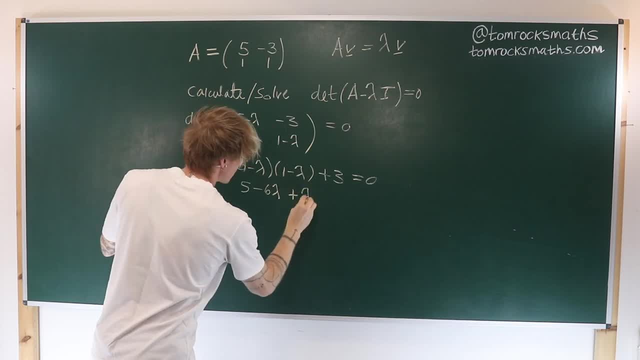 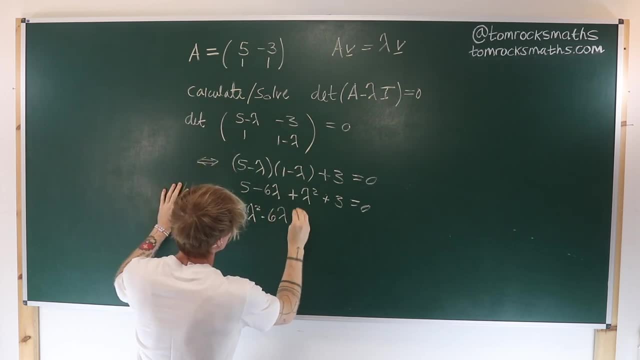 lambda minus 6. lambda plus lambda squared plus 3, plus zero, so that becomes lambda squared minus 6. lambda plus 8, is zero and that factorizes really nicely into lambda minus 4,. lambda minus 2,. 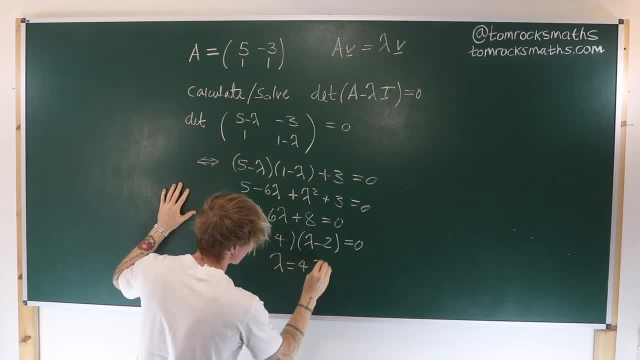 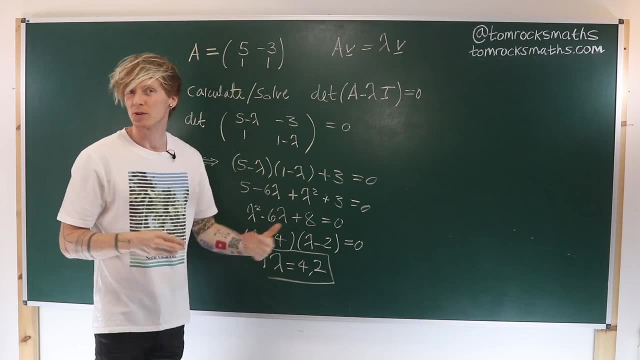 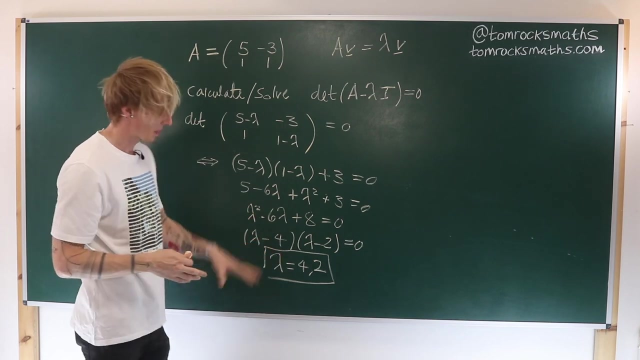 equals zero, so lambda is 4, or 2.. So our eigenvalues here are lambda equals 4, and lambda equals 2.. Now just to say for this step here I was able to spot that this factorizes really nicely. Of course they won't always factorize and you can use the quadratic equation. 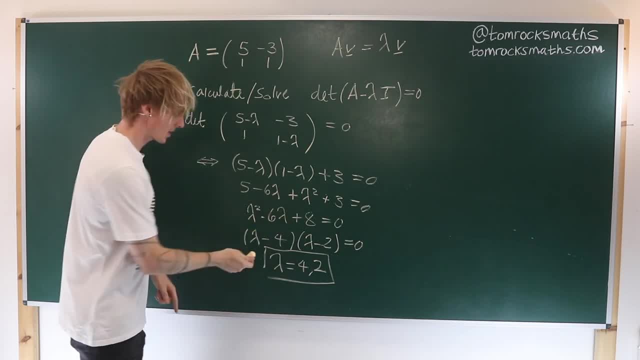 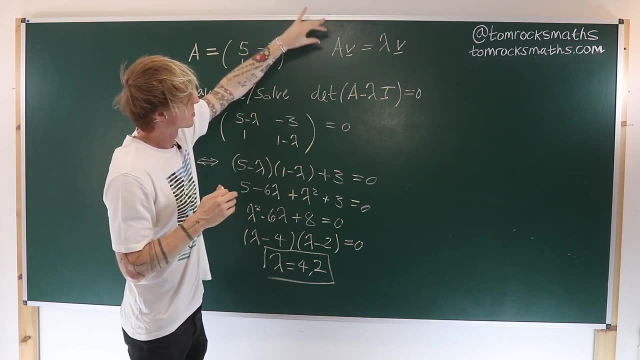 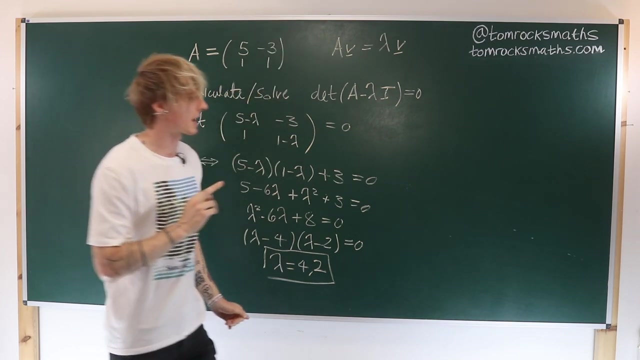 and you can use the quadratic equation here to solve for your roots, lambda. So we now know the eigenvalues are 4 and 2.. So, following our method, we now have to plug them in to our equation to actually find the eigenvector v, And here we're considering a general v. 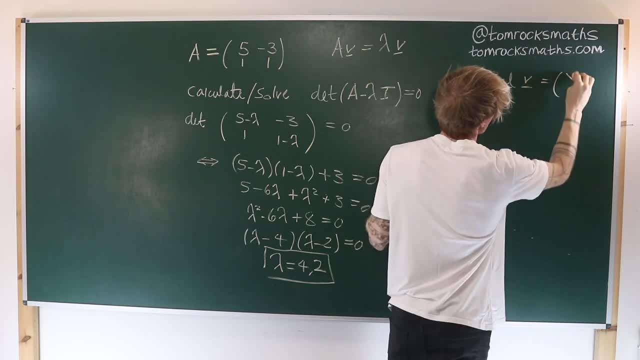 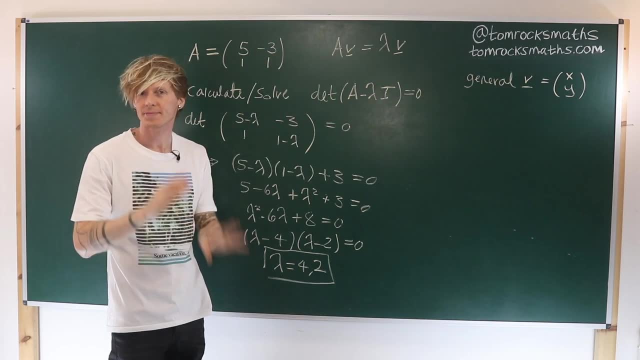 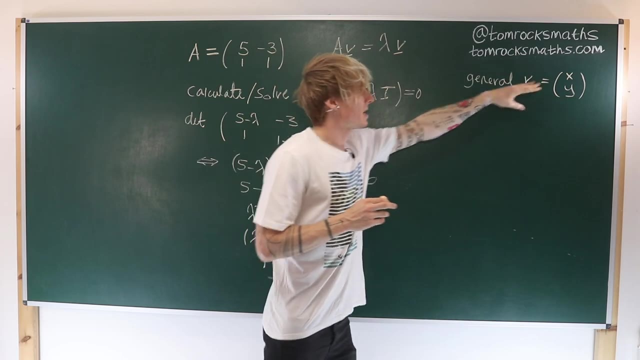 which has to be 2d. so v here is going to be xy and we need to find the direction of this vector. Now there's an important thing to spot at this point in the calculation, which is to say if v, some vector, satisfies this equation once we've fixed lambda. 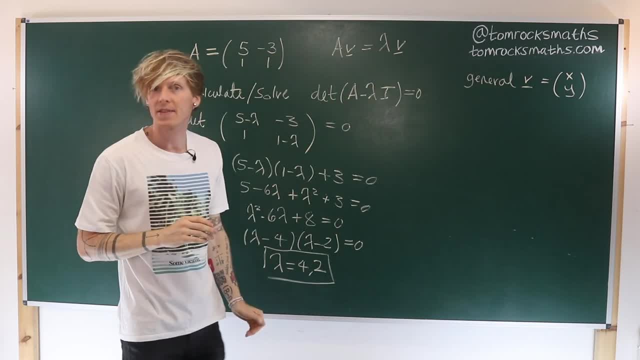 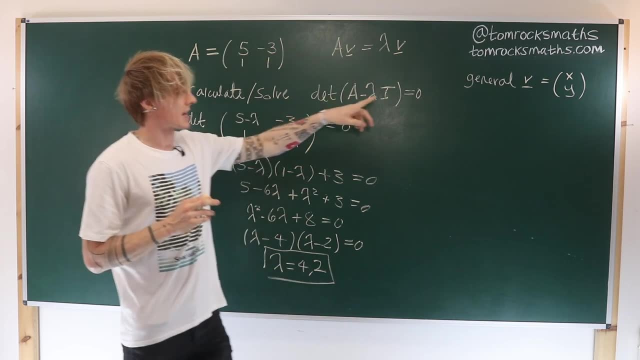 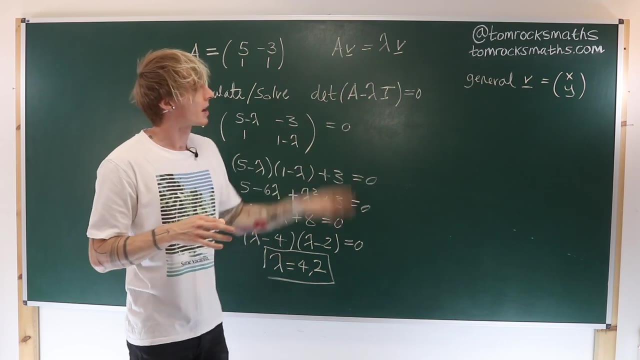 And we need to find the direction of this vector. Now there's an important thing to spot at this point in the calculation, which is to say, if v, some vector satisfies this equation, once we've fixed lambda, then in fact any multiple of v will also satisfy this equation. 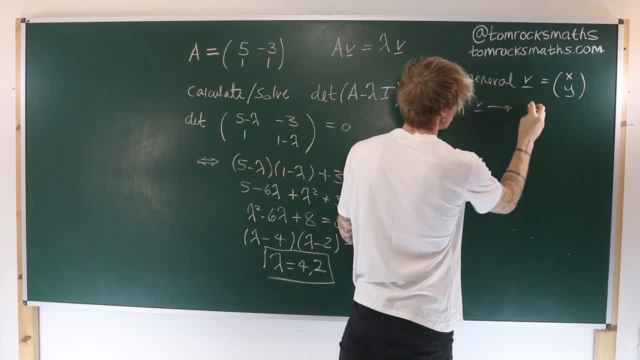 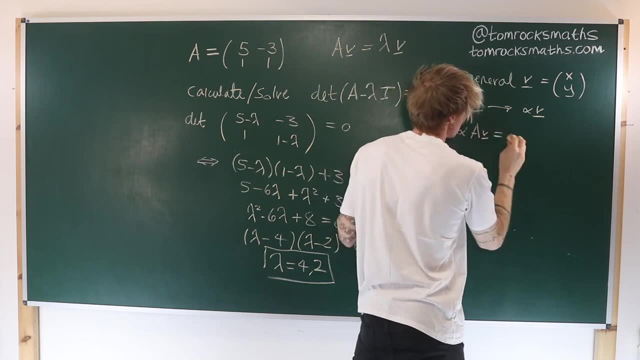 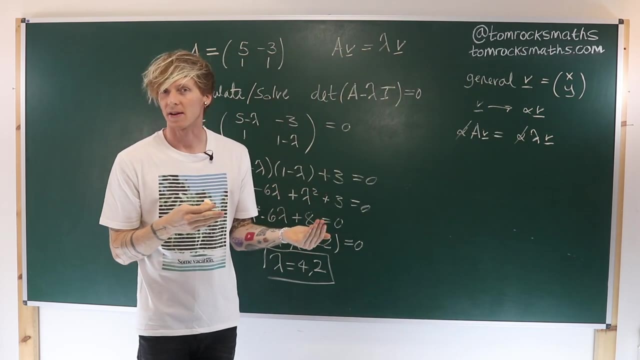 Because if I simply replace v by alpha times v, then my equation up here just becomes: alpha av equals alpha under v, so I cancel the alpha and the same equation is satisfied. So when we're looking for a general v, we have some freedom in multiplying lambda. 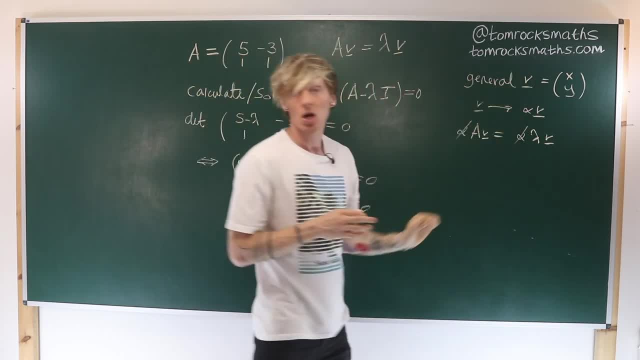 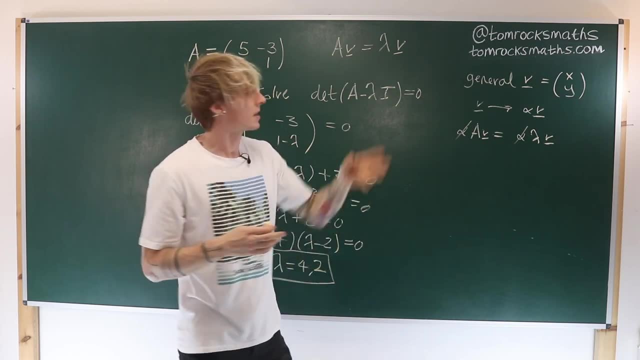 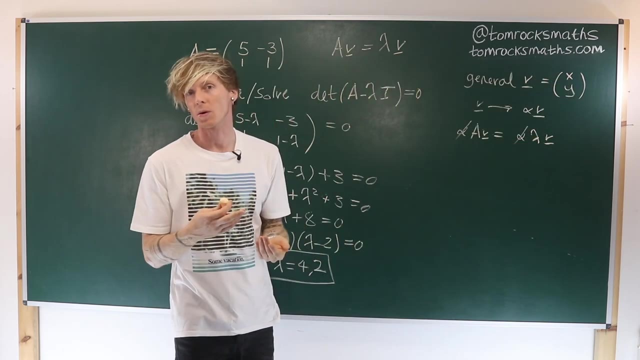 The whole thing, both x and y, by the same constant number, And that's important to remember. We're actually just interested in the direction of this vector. So if you were to plot this like a triangle, you would have a fixed angle, because it would be the ratio of these that would be equal to tan theta. 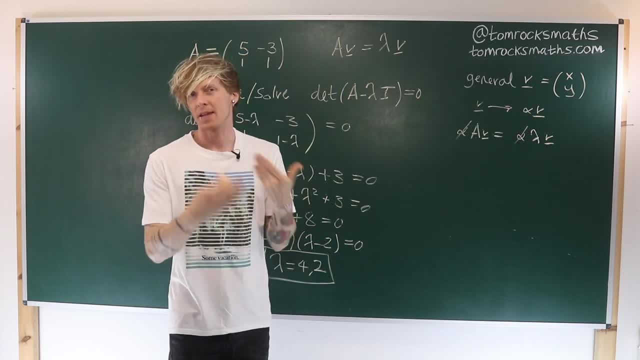 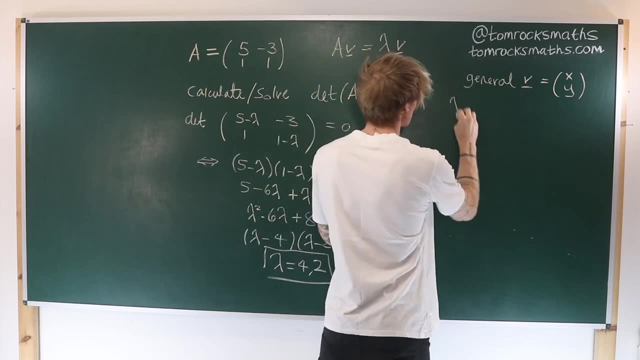 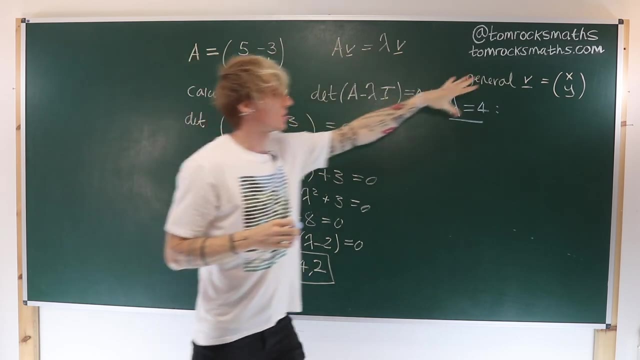 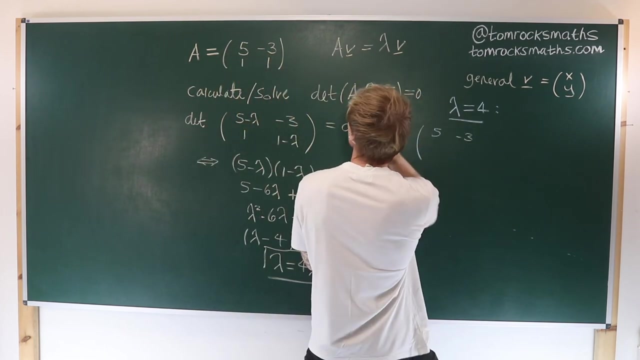 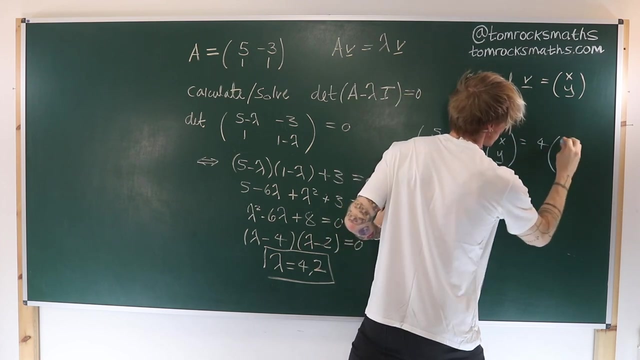 and so multiplying by this constant alpha wouldn't affect that angle, and so the direction would be the same. If we start with lambda equals 4, and we sum Substitute lambda equals 4 into our eigenvalue equation for this general v, Then what we have is 5 minus 3, 1, 1, times x. y has to be equal to 4 times x- y. 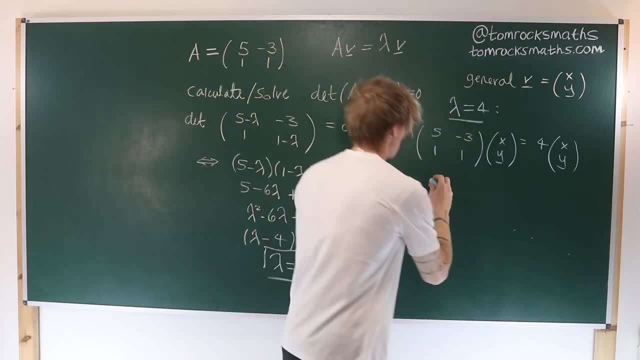 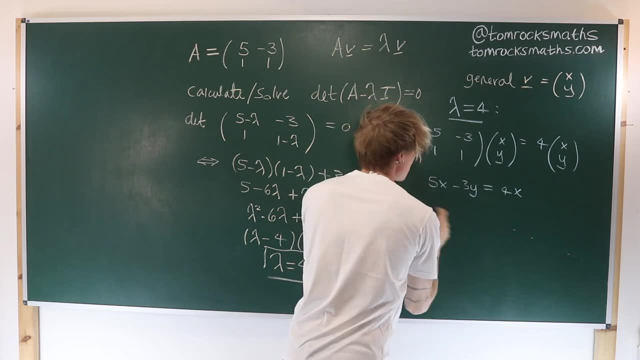 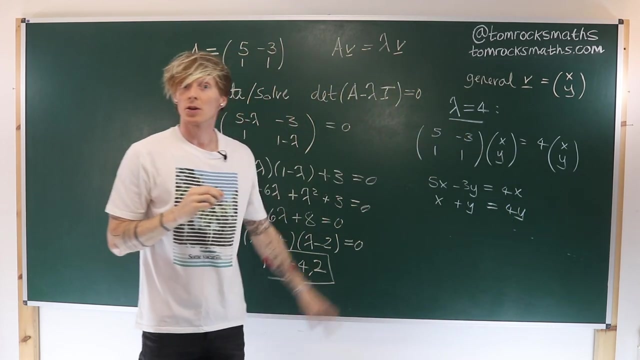 So now we can expand this out. So the first row is going to give me x minus 3, y has to be equal to 4x and the bottom row says x plus y is equal to 4y. So, rearranging the second one, this tells me here that I can say: x, therefore is 3y. 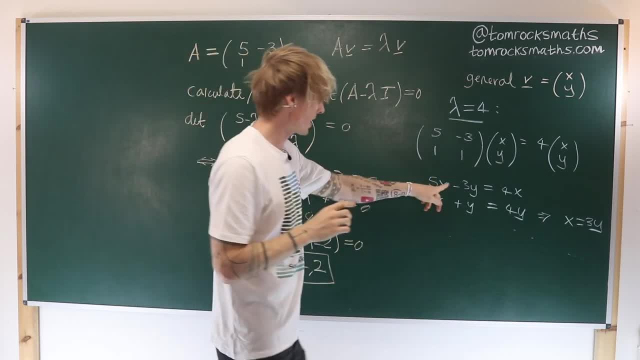 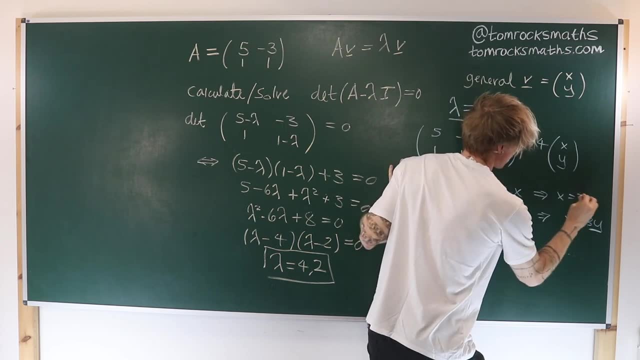 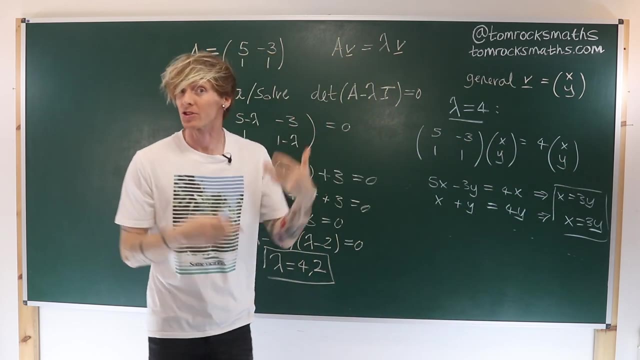 and then in this top equation I can also take the 3y across, subtract the 4x and that also gives me x equals 3y, And the reason we have the same equation is what I was just talking about regarding we can multiply v by some constant alpha. 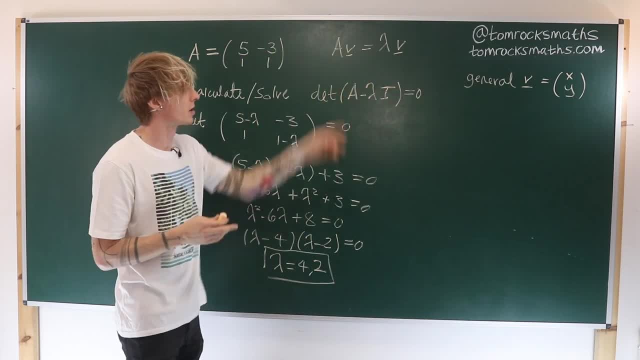 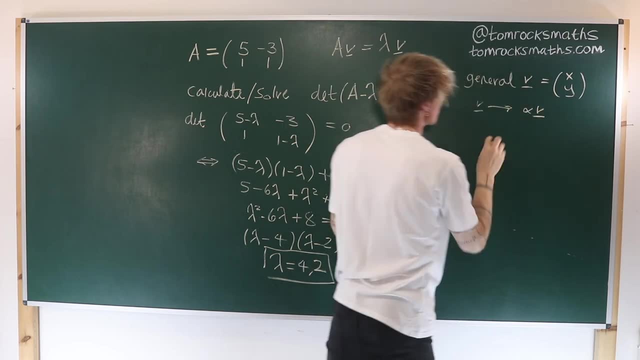 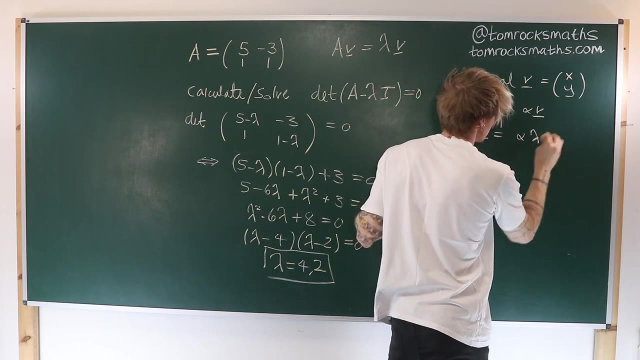 then in fact any multiple of v will also satisfy this equation. Because if I simply replace v by alpha times v, then my equation up here just becomes alpha. a v equals alpha and a v, so I cancel the alpha and the same equation is satisfied. 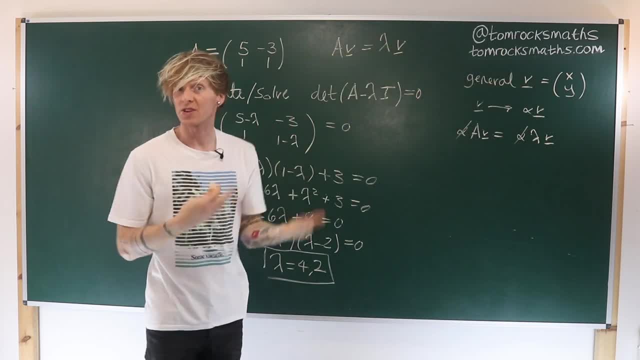 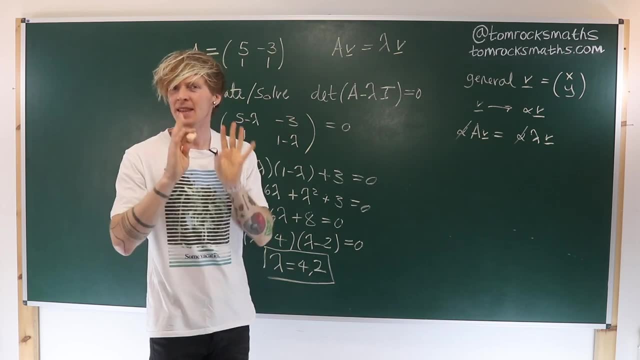 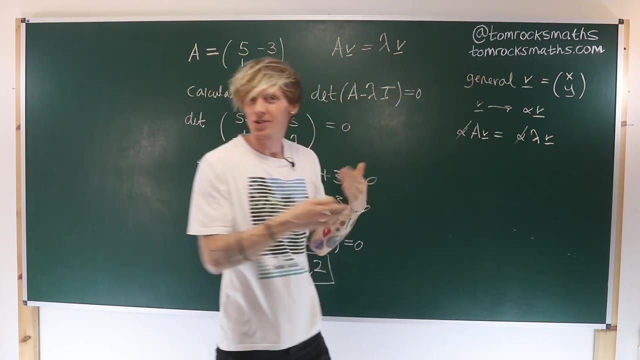 So when we're looking for a general v, we have some freedom in multiplying the whole thing- both x and y, by the same constant number, And that's important to remember. We're actually just interested in the direction of this vector. So if you were to plot this like a triangle, 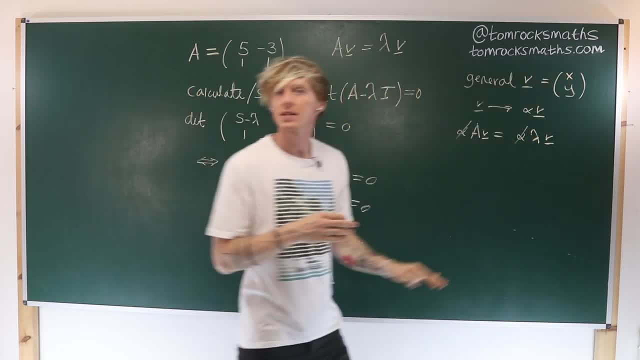 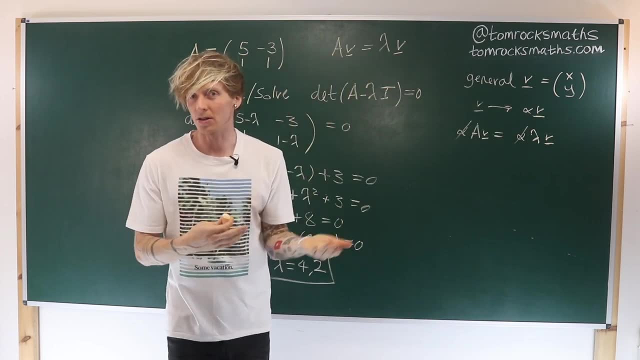 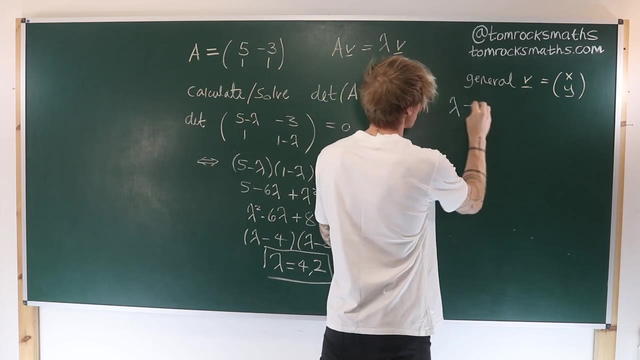 you would have a fixed angle, because it would be the ratio of these that would be equal to tan theta, And so multiplying by this constant alpha wouldn't affect that angle, and so the direction would be the same. If we start with lambda equals 4, and we substitute lambda equals 4, 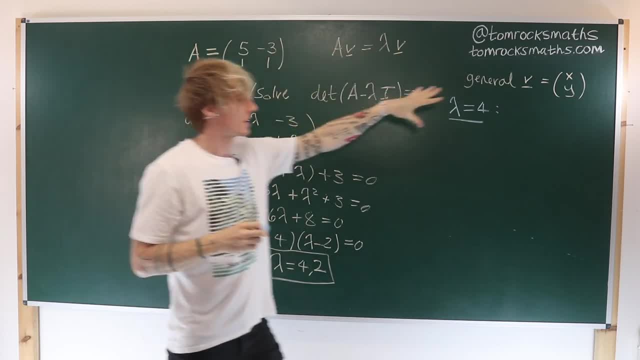 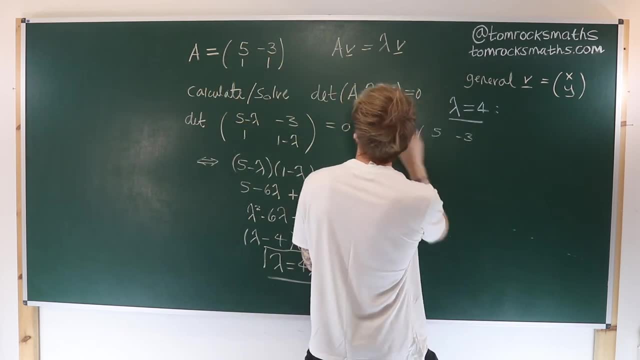 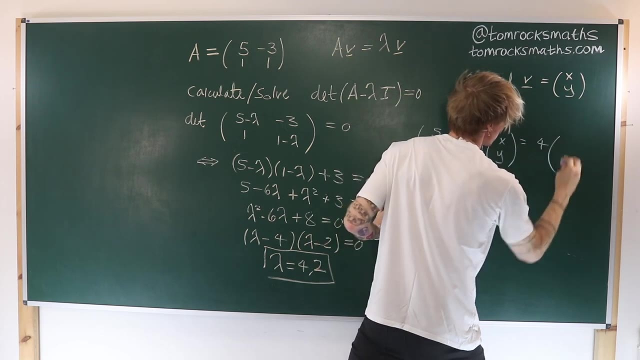 into our eigenvalue equation for this general v. then what we have is 5 minus 3, 1, 1, times x. y has to be equal to 4 times x- y. So now we can expand this out. So the first row. 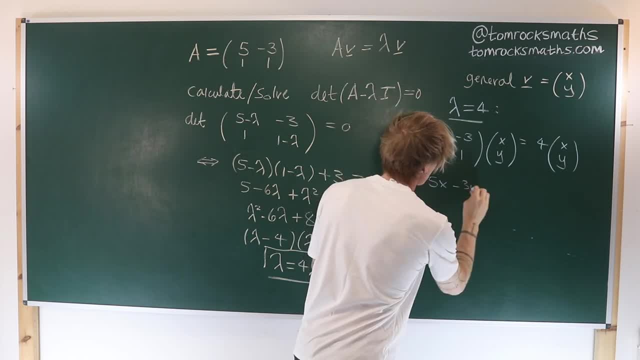 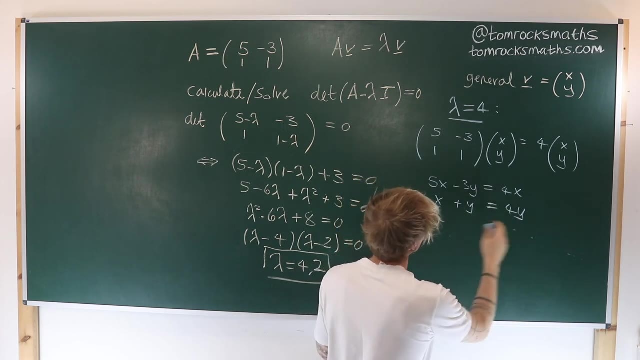 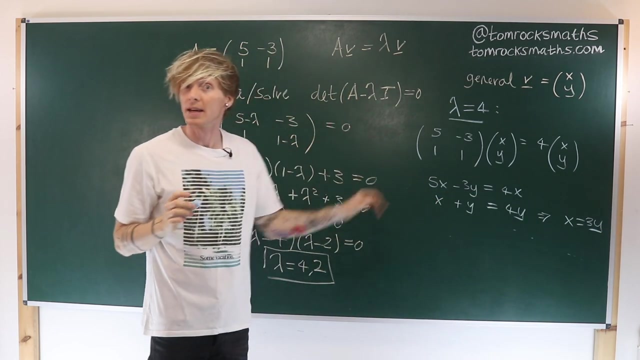 is going to give me 5x minus 3y has to be equal to 4x, and the bottom row says x plus y is equal to 4y. So rearranging the second one, this tells me here that I can say x, therefore is 3y, and then in this top equation I can also take the 3y across. 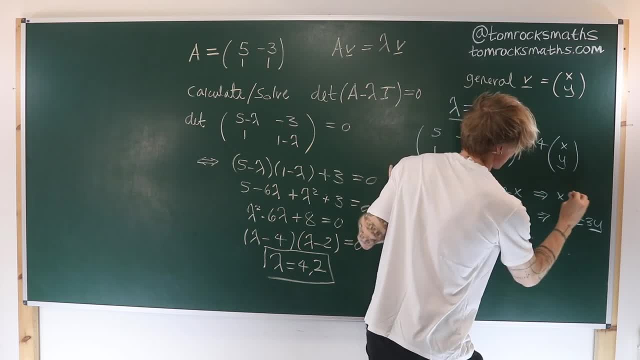 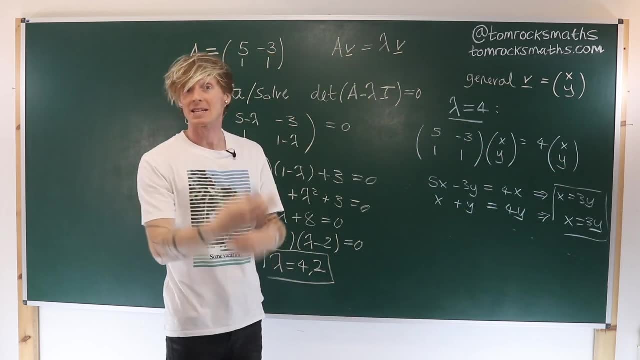 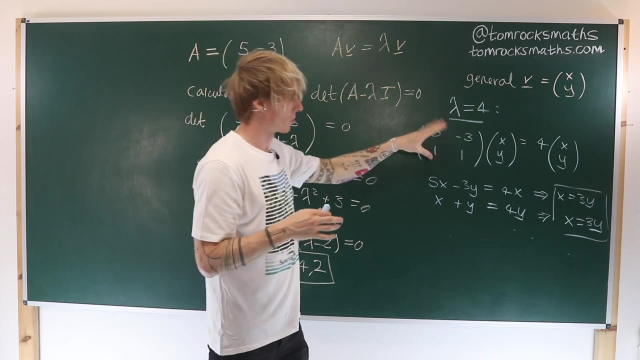 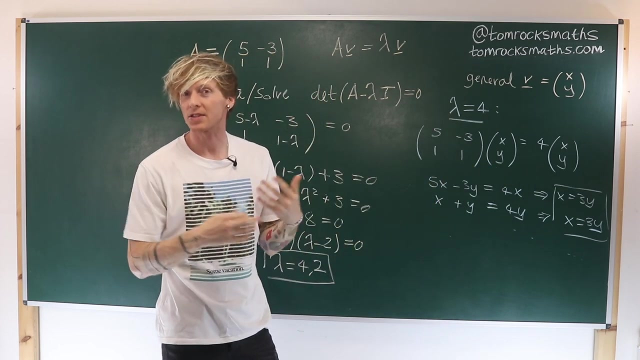 subtract the 4x and that also gives me x equals 3y, And the reason we have the same equation is what I was just talking about regarding we can multiply v by some constant alpha, So you'll find that the values in your eigenvector equation will actually be multiples of one another in a lot of. 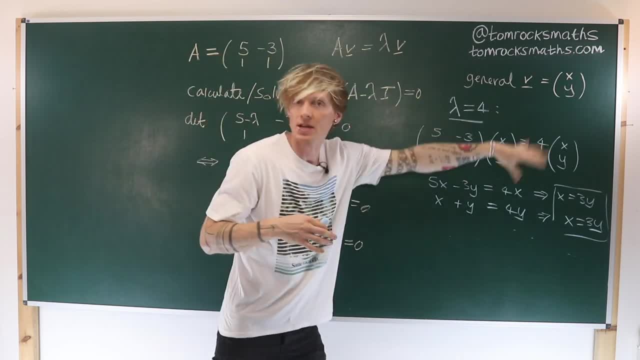 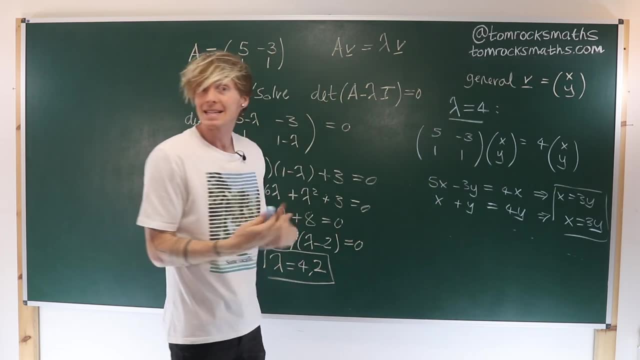 So you'll find that your rows in your eigenvector equation will actually be multiples of one another in a lot of cases, So we're free to pick one of the values for x or y. So, to make things easy for ourselves, I'm going to let 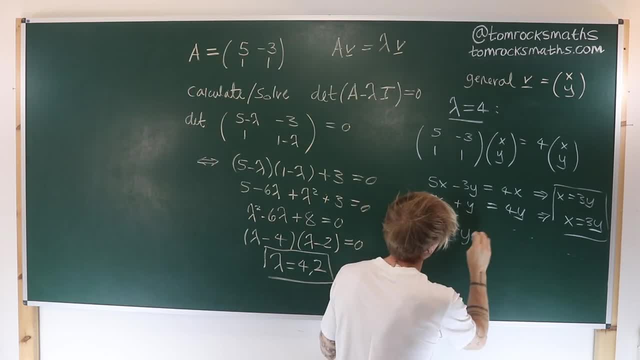 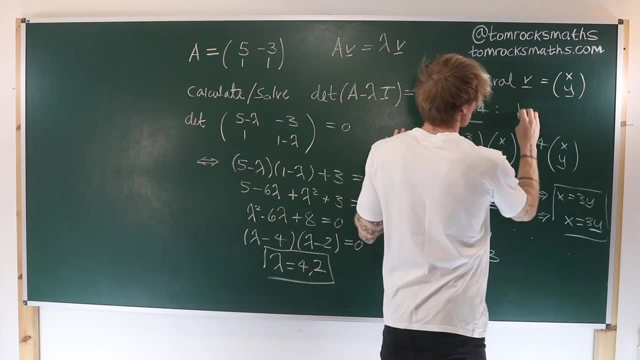 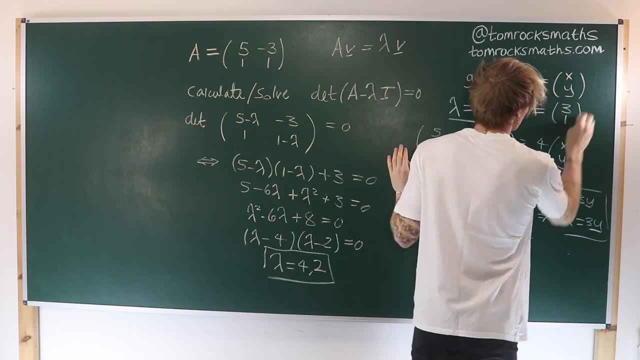 y be equal to 1,, and then, in order to satisfy this equation, I need x to be equal to 3.. So this gives me my eigenvector for the eigenvalue of 4 to be given by 3, 1.. 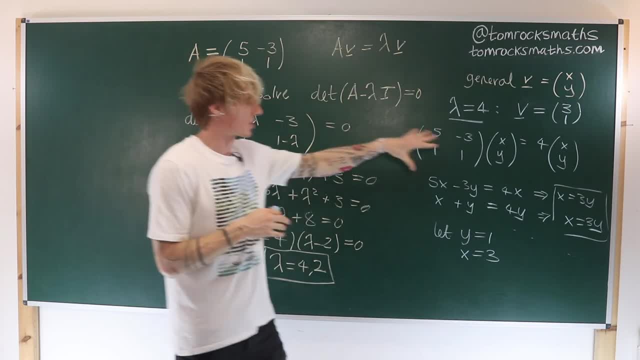 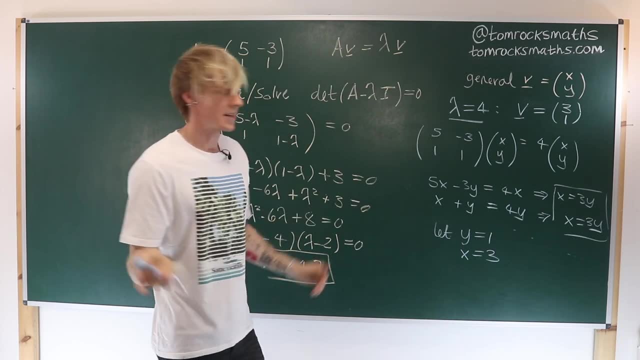 Now, of course, it's always worth checking your answer. You want to make sure that these values of x and y satisfy the simultaneous equations. Unfortunately, we can see that they do, because 5 times x gives me 15, minus 3 equals 4 times 3, which is 12.. 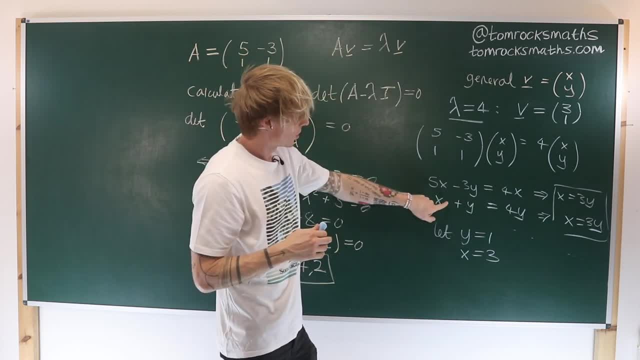 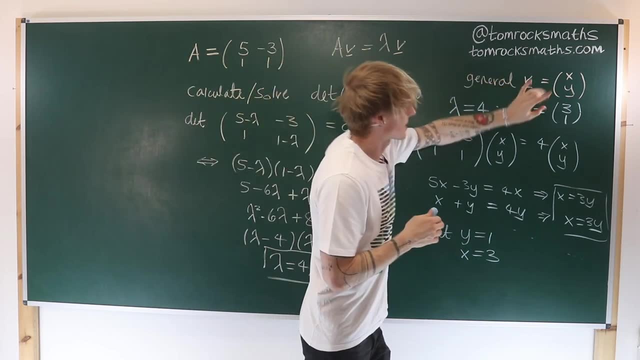 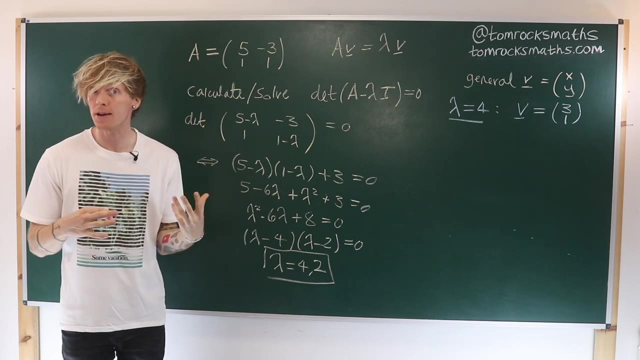 And similarly x plus y, that's 4, equals 4 lots of 1, which is also 4.. So for the eigenvalue of 4, we have an eigenvector given by 3, 1.. The calculation for our second eigenvalue is very similar. 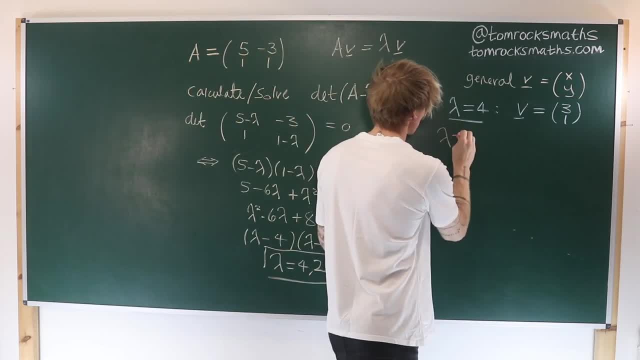 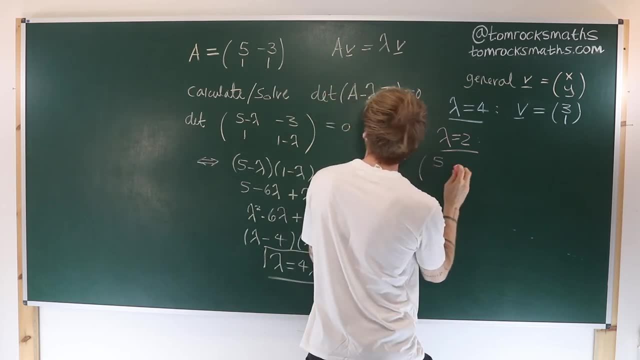 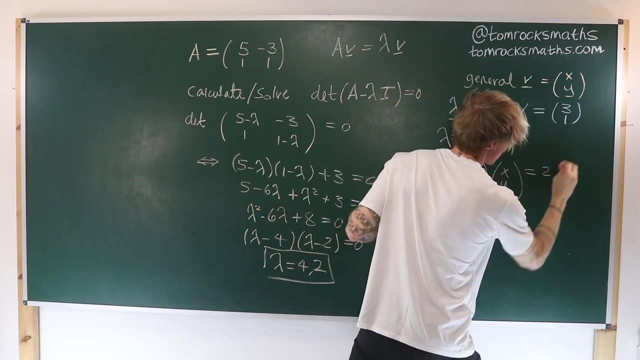 So we begin by saying: when lambda is 2,, we want to satisfy this equation. So that says 5 minus 3, 1, 1 times x y needs to be equal to 2, lots of x, y. As before we expand this out. 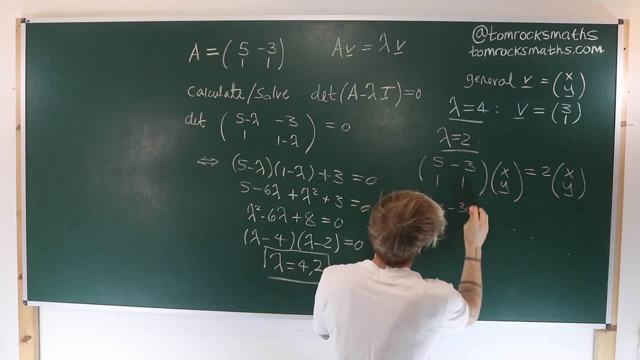 So we get our simultaneous equations: 5x minus 3y has to equal 2x. So I can immediately see that's going to tell me that x is equal to y, And the second one tells me that x plus y has to be equal to 2y. 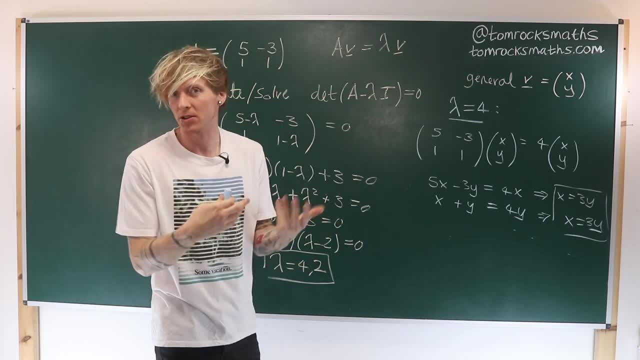 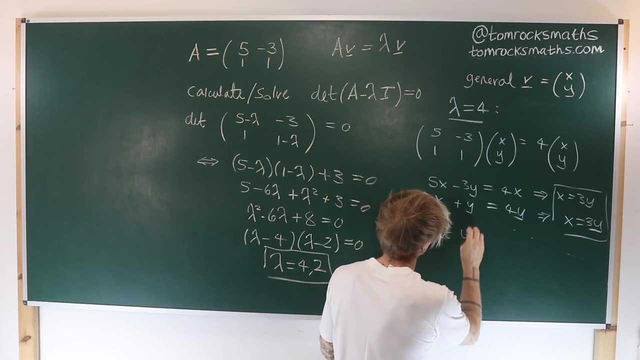 cases. So we're free to pick one of the values for x or y. So, to make things easy for ourselves, I'm going to let y be equal to 1, and then, in order to satisfy this equation, I need x to be. 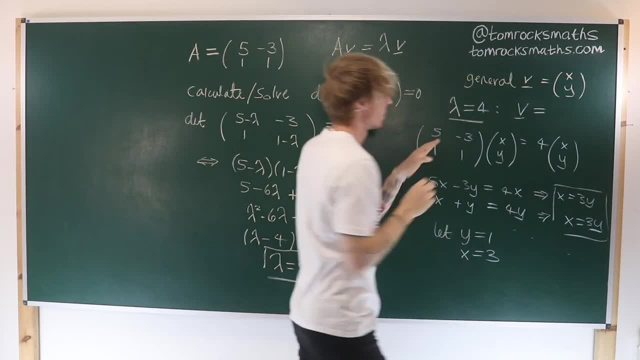 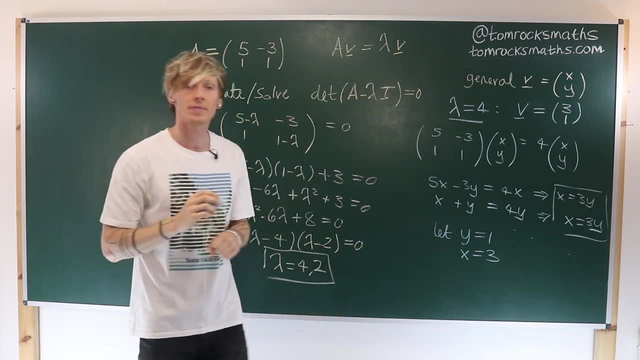 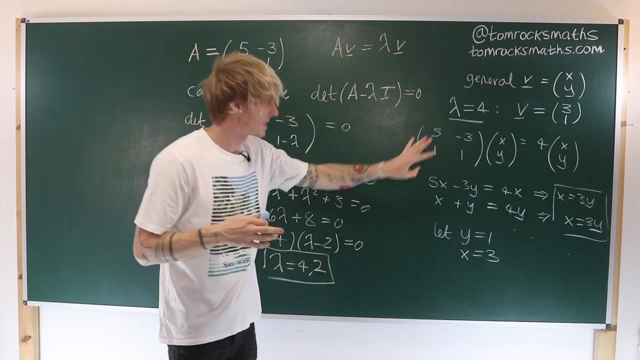 equal to 3.. So this gives me my eigenvector for the eigenvalue of 4, to be given by 3, 1.. Now, of course, it's always worth checking your answer. You want to make sure that these values of x and y satisfy the simultaneous equations. Unfortunately, 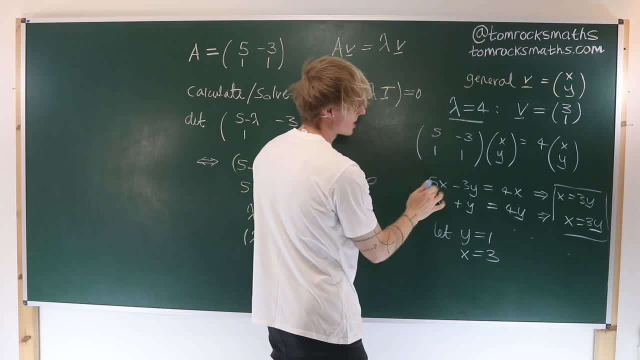 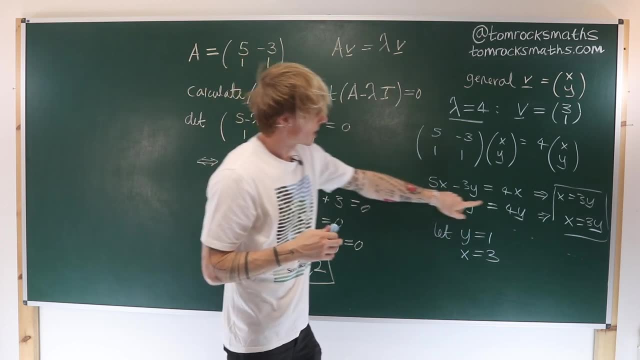 we can see that they do, because 5 times x gives me 15, minus 3 equals 4 times 3,, which is 12.. And similarly, x plus y, that's 4, equals 4, lots of 1, which is also 4.. 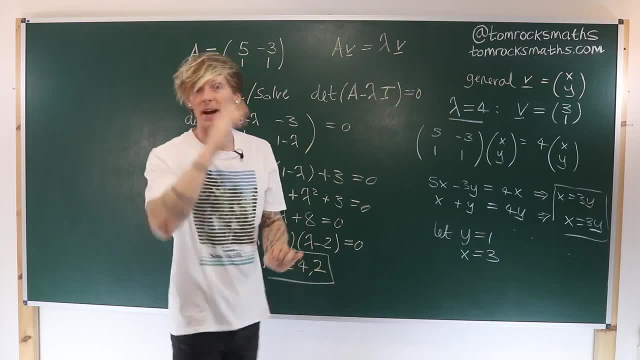 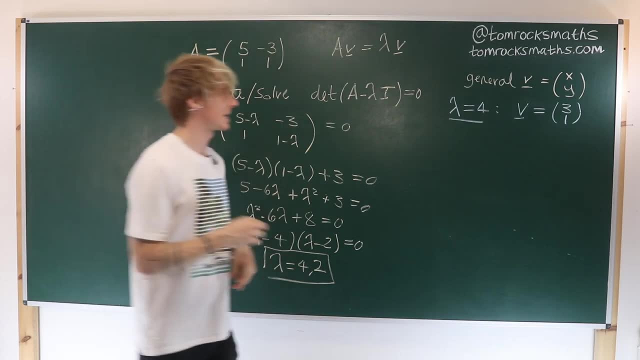 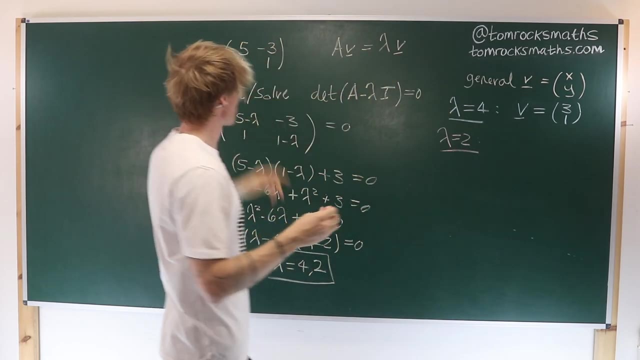 So for the eigenvalue of 4, we have an eigenvector given by 3, 1.. The calculation for our second eigenvalue is very similar. So we begin by saying: when lambda is 2, we want to satisfy this equation. So that says: 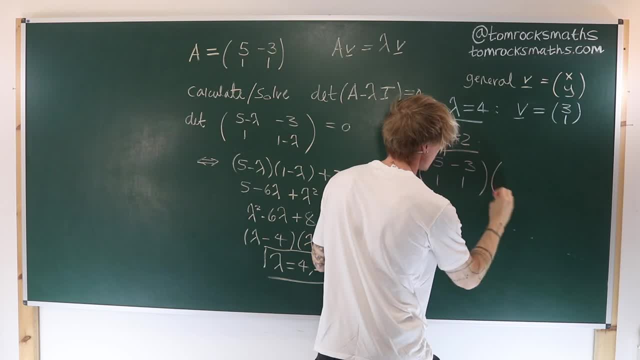 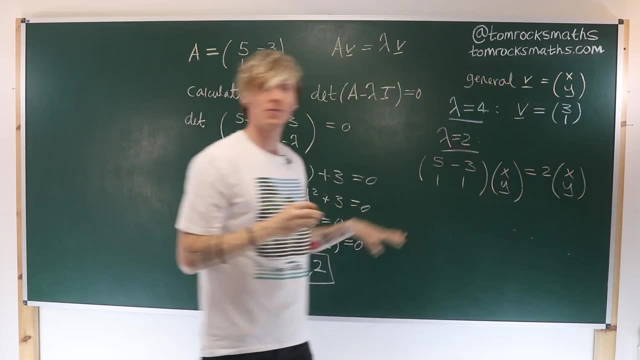 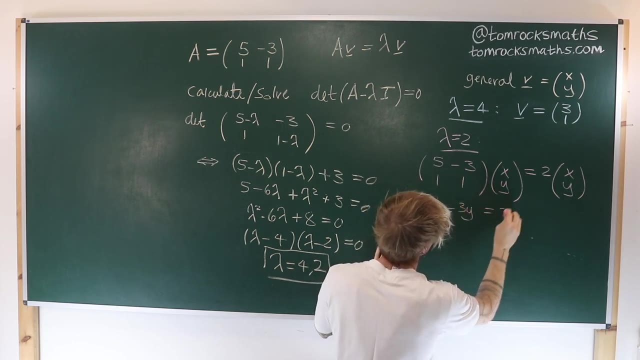 5 minus 3, 1, 1 times x y needs to be equal to 2. lots of x y. Before we expand this out, so we get our simultaneous equations: 5x minus 3y has to equal to. 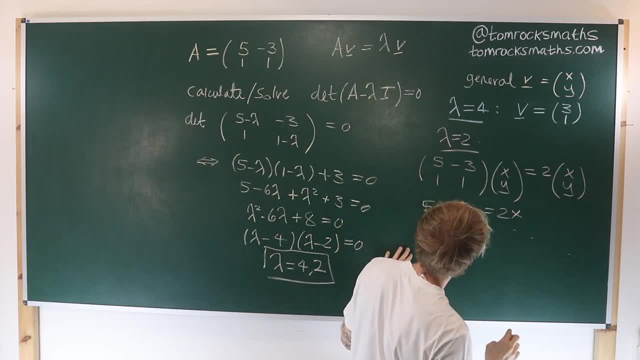 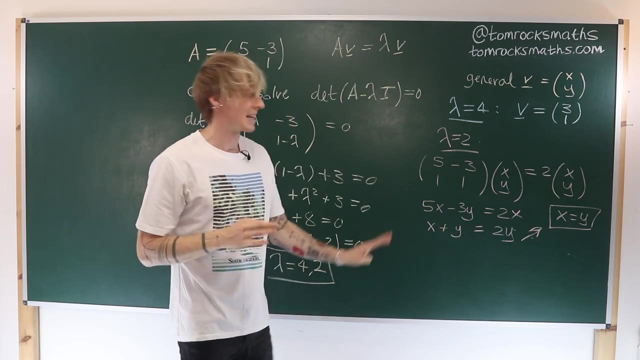 x. So I can immediately see that's going to tell me that x is equal to y. And the second one tells me that x plus y has to be equal to 2y, which also, when you subtract y from both sides, gives me that x is equal to y. So we can pick any value. 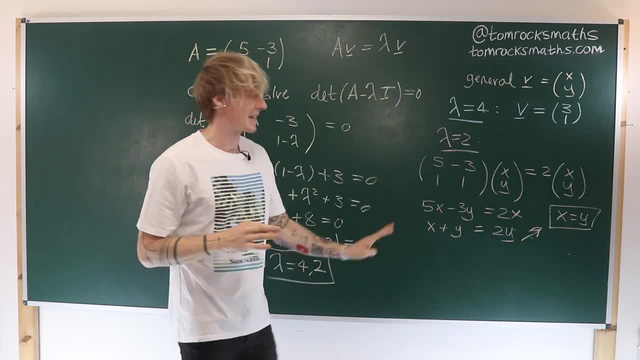 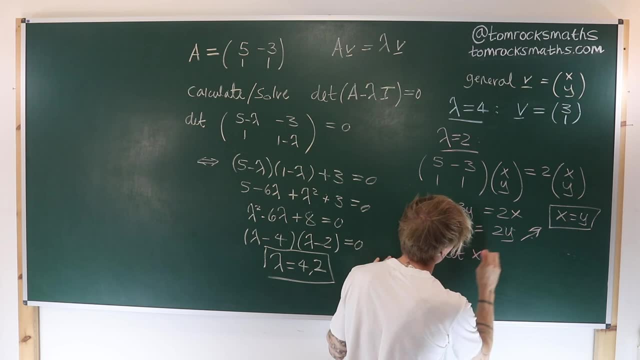 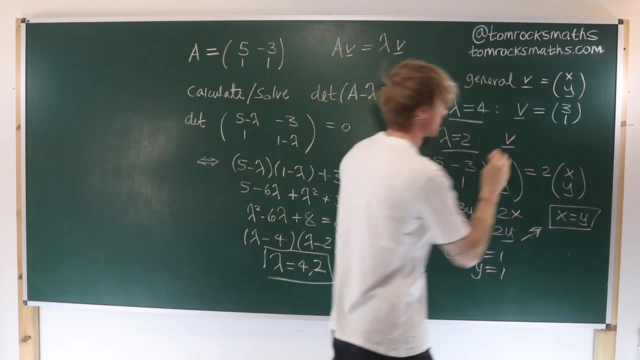 which also, when you subtract y from both sides, gives me that x is equal to y. So we can pick any value. We keep things simple. We say: let x equal 1, then y is also 1.. So our eigenvector for the eigenvalue of 2 is given by 1, 1.. 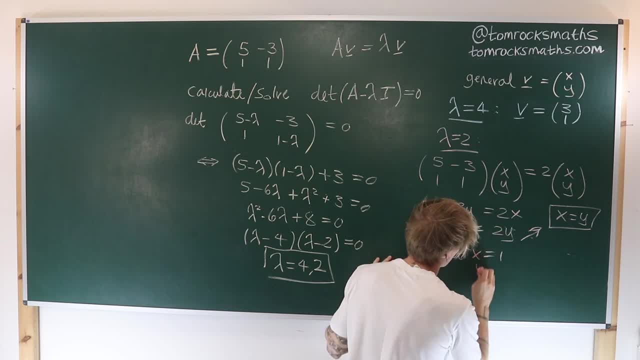 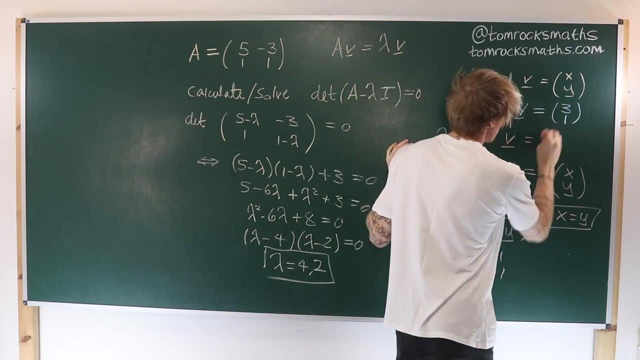 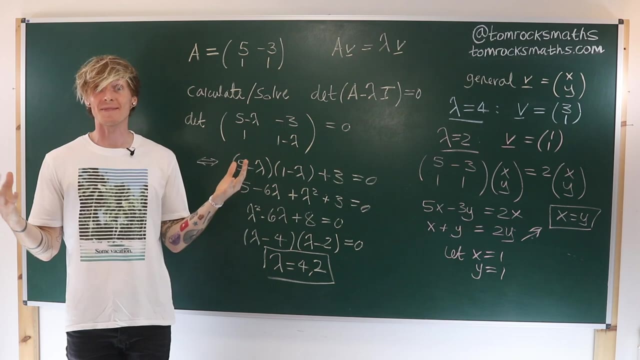 we keep things simple. we say: let x equal 1, then y is also 1.. So our eigenvector for the eigenvalue of 2 is given by 1, 1.. So it's a line with a 45 degree angle, And that's it. We found both. 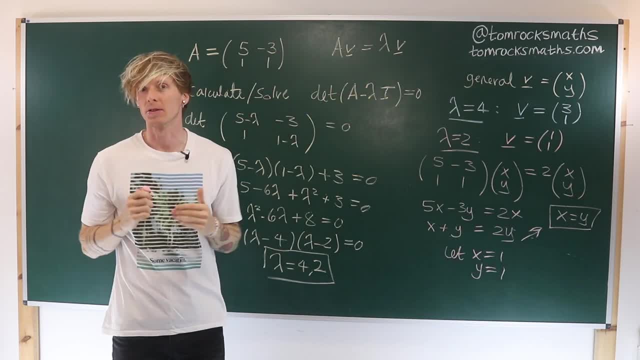 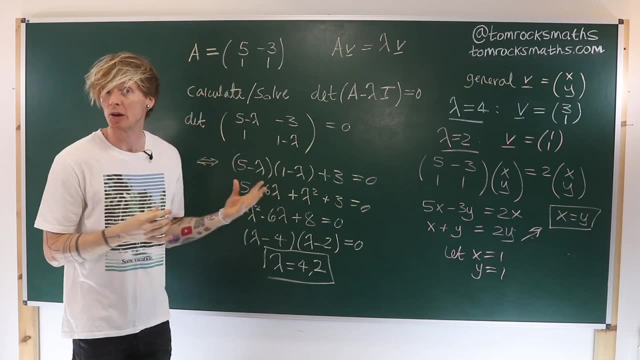 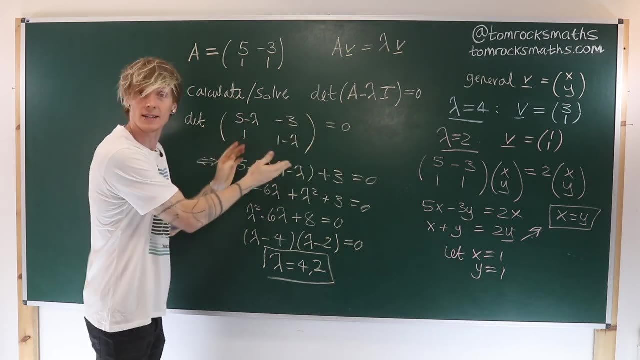 So it's a line with a 45 degree angle, And that's it. We found both eigenvalues by solving our characteristic polynomial, The determinant of a minus lambda times the identity had to be 0. This gave us a quadratic equation. We could factorize it here or use the quadratic formula. 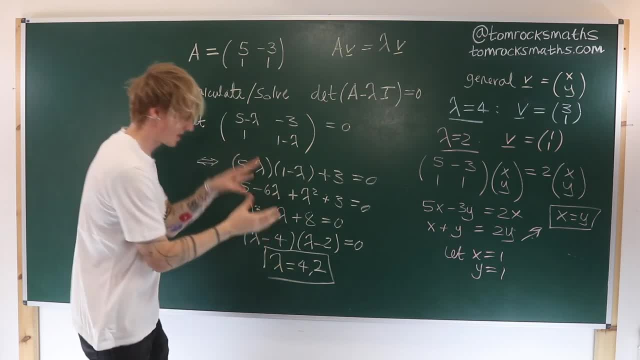 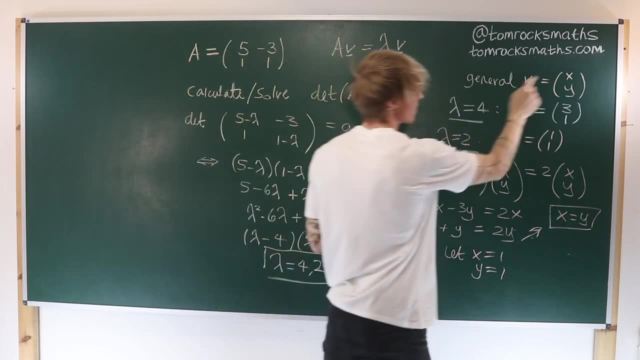 to get the solutions that lambda must be 4 or 2.. These are our eigenvalues. We then substitute those in One at a time And solve for a general vector- x, y, to find when we have an eigenvalue of 4,. 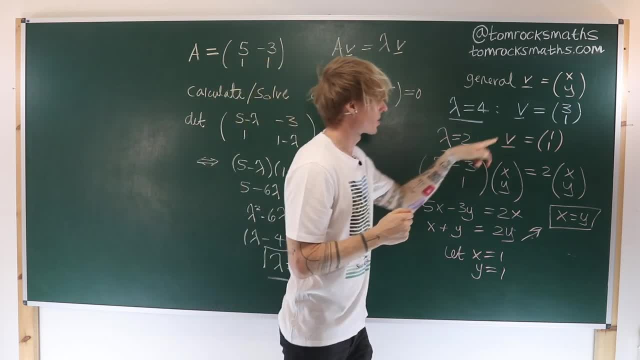 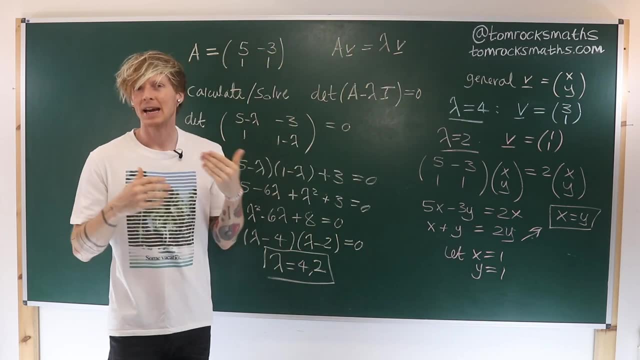 the vector is 3, 1.. And when we have an eigenvalue of 2,, v is given by 1, 1.. And, of course, both of these are non-zero, so therefore they are valid eigenvectors. Now let's look at an example with a 3x3 matrix. 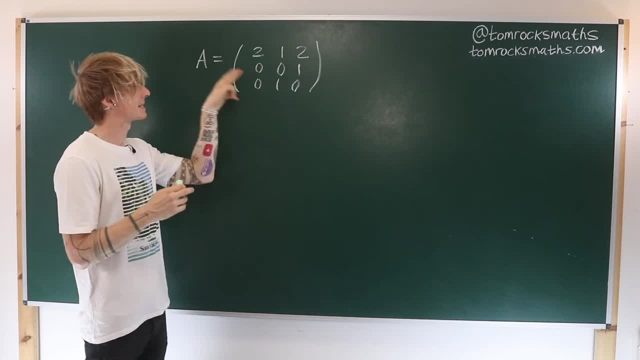 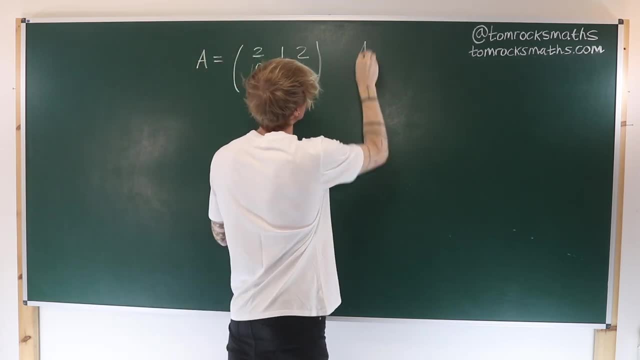 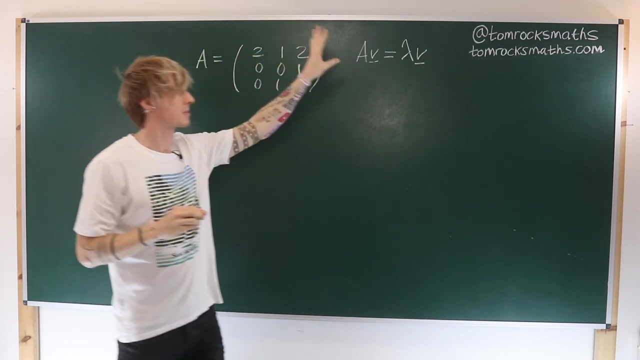 given by a is equal to 2, 1, 2, 0, 0, 1, 0, 1, 0.. As before, we start by saying we want to find non-zero v and lambda, such that a times the vector v equals lambda times the same vector v. 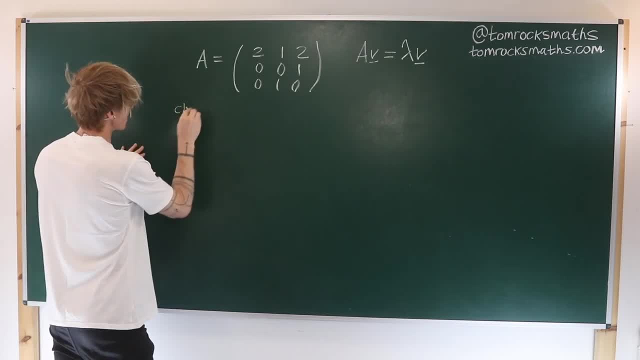 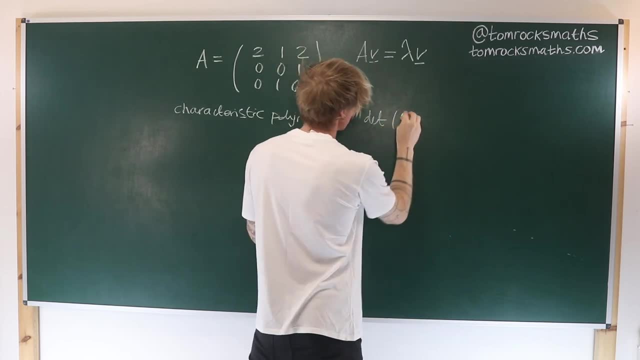 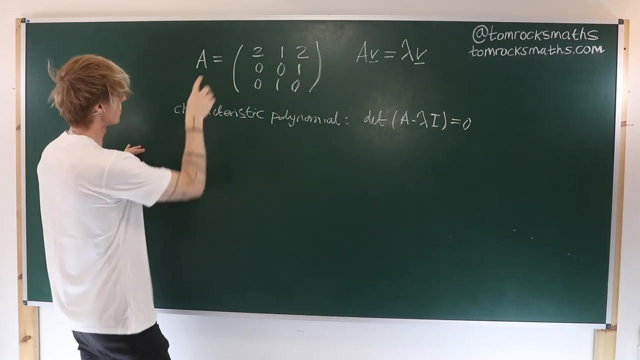 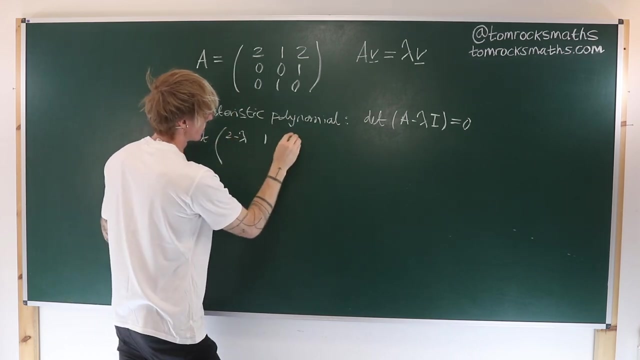 And again we need to solve the characteristic polynomial which still says that the determinant of a minus lambda i has to be equal to 0. So our matrix now becomes 2 minus lambda 1, 2.. Then we get 0. 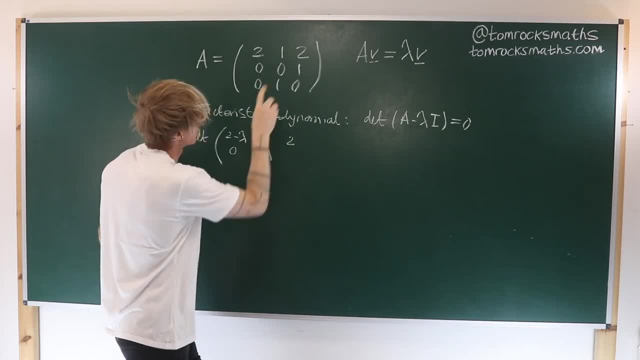 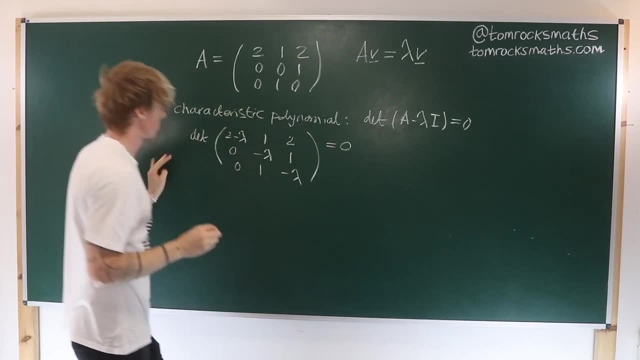 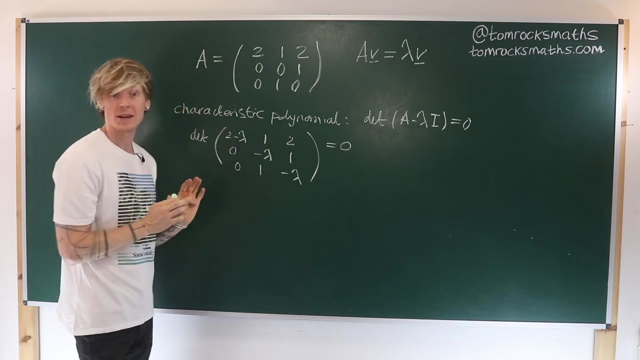 This one now has a minus lambda and a 1. And on the bottom, 0, 1 minus lambda And we need to solve this 3x3 determinant equal to 0.. Now, looking at the matrix, the form of the matrix that we have, 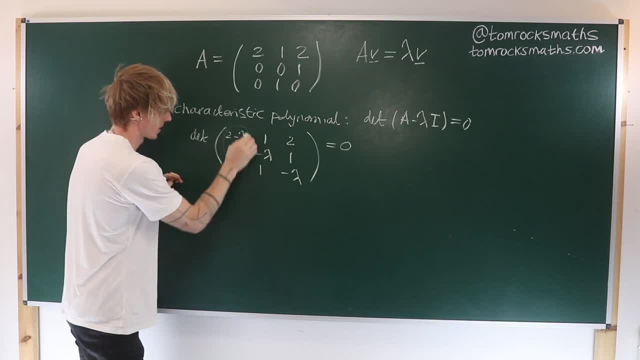 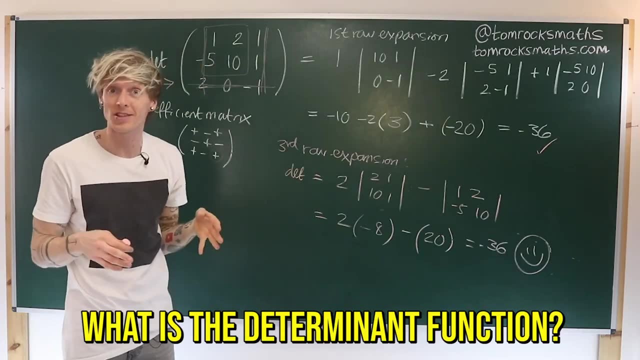 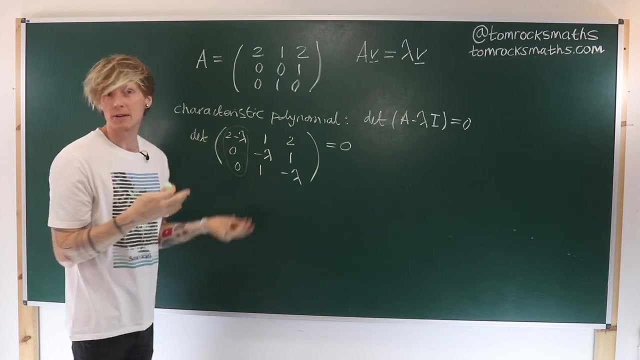 we can see that this first column contains a lot of zeros, And we talked about this in the earlier determinants video. I think this was video 2 or 3 in the Oxford Linear Algebra series- And we said that when you have lots of zeros in a row or column- 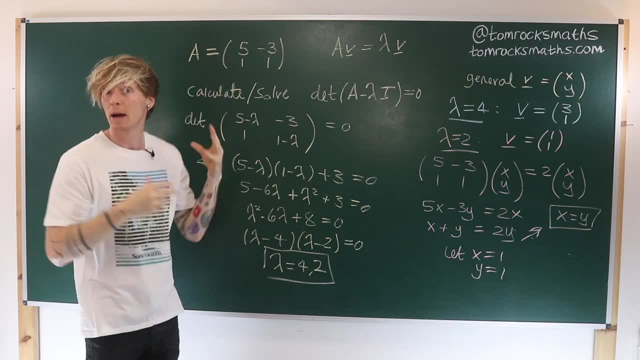 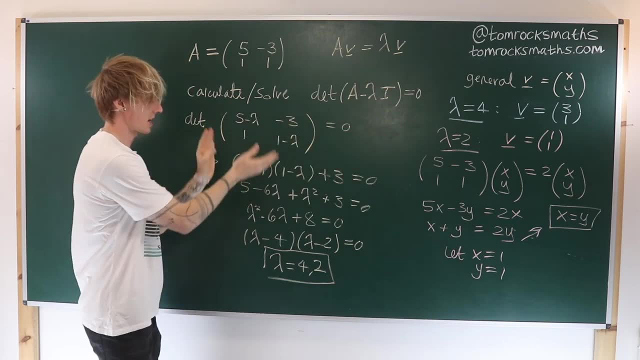 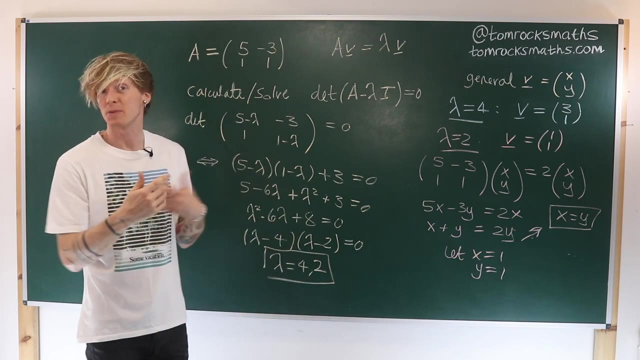 eigenvalues by solving our characteristic polynomial. the determinant of a minus lambda times the identity had to be 0. This gave us a quadratic equation. We could factorize it here or use the quadratic formula to get the solutions that lambda must be 4 or 2.. 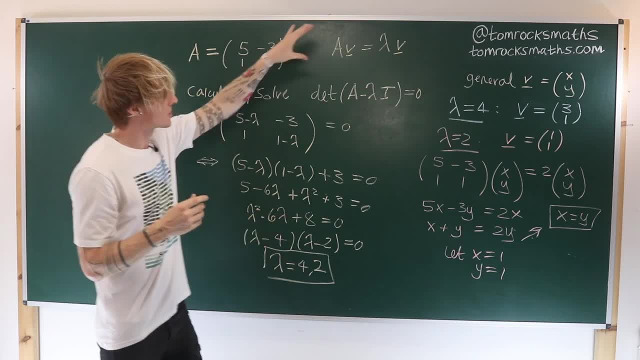 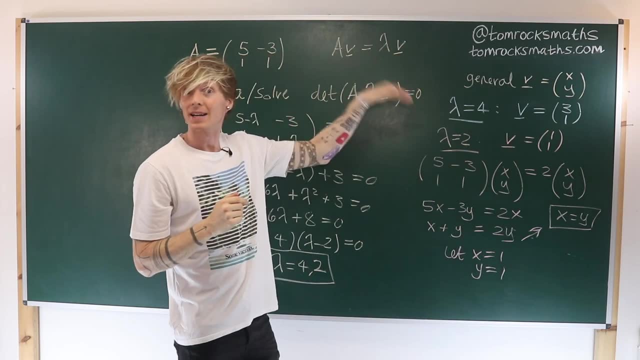 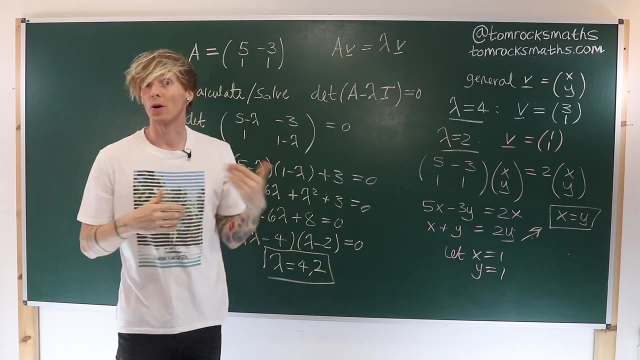 These are our eigenvalues. We then substitute those in one at a time and solve for a general vector xy to find. when we have an eigenvalue of 4, the vector is 3, 1, and when we have an eigenvalue of 2, v is given by 1, 1 and, of course, 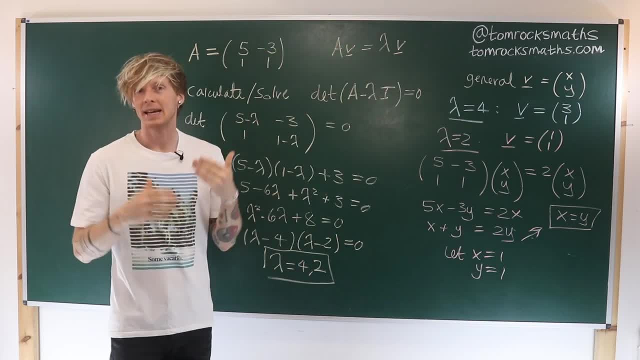 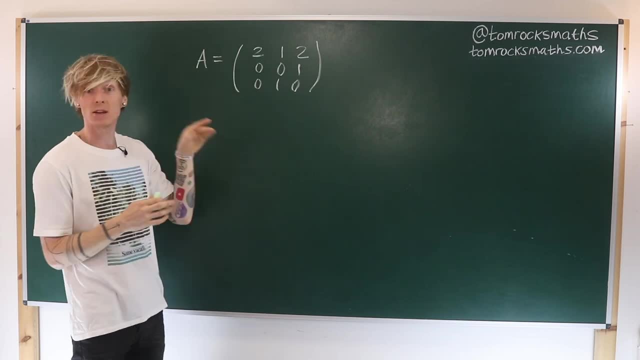 both of these are nonzero, so therefore they are valid eigenvectors. Now let's look at an example. with a 3 by 3, matrix given by a is equal to 2, 1, 2, 0, 0, 1 0, 1, 0.. 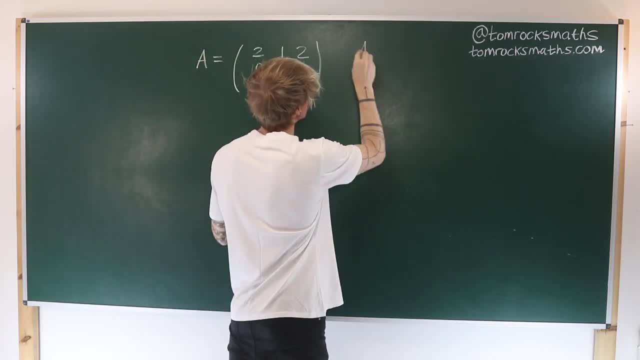 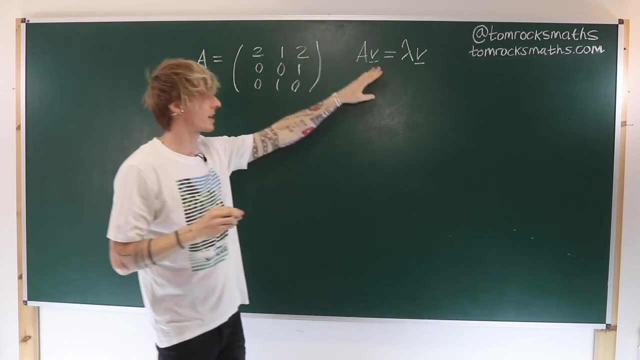 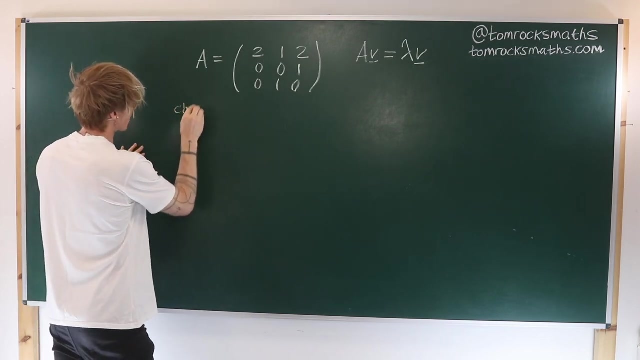 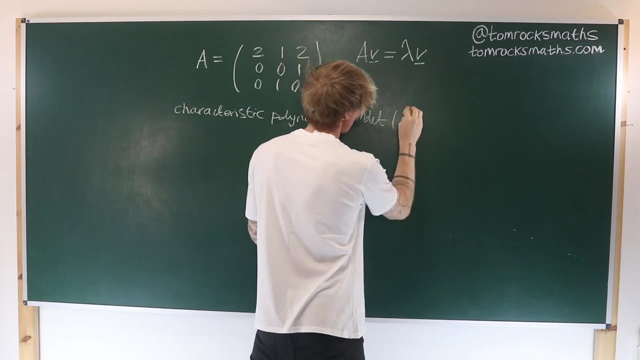 As before, we start by saying: we want to find nonzero v and lambda such that a times the vector v equals lambda times the same vector v. And again we need to solve the characteristic polynomial, which still says that the determinant of a minus lambda i. 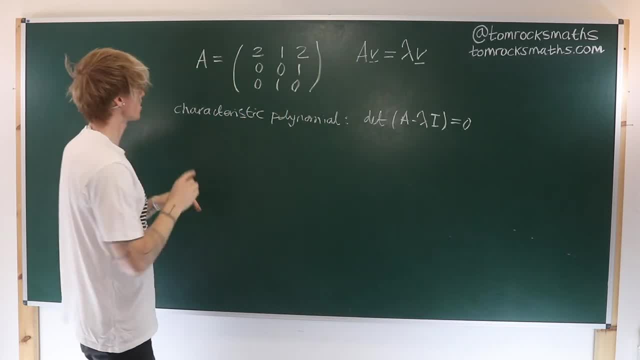 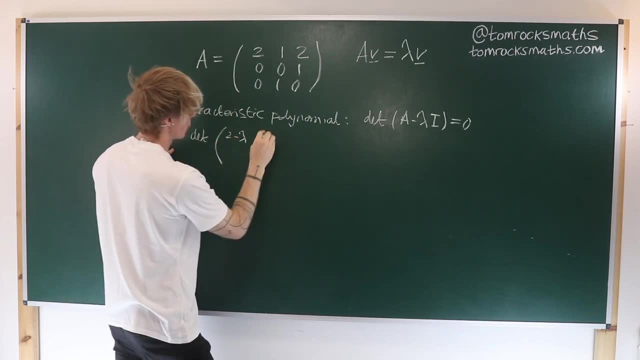 has to be equal to 0. So our matrix now becomes 2 minus lambda, 1, 2.. Then we get 0. This one now has a minus lambda And a 1. And on the bottom, 0, 1.. 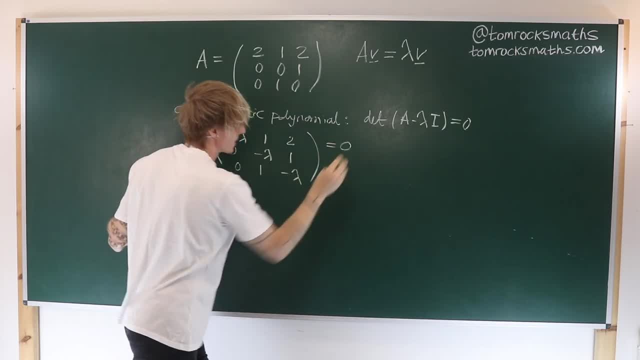 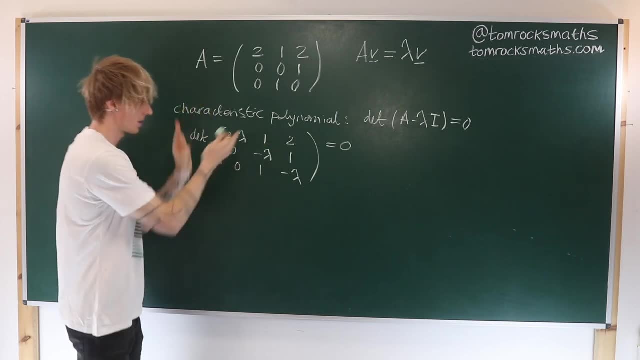 Minus lambda And we need to solve this 3 by 3 determinant equal to 0.. Now, looking at the matrix- the form of the matrix that we have- we can see that this first column contains a lot of zeros, And we talked about this in the earlier determinants video. 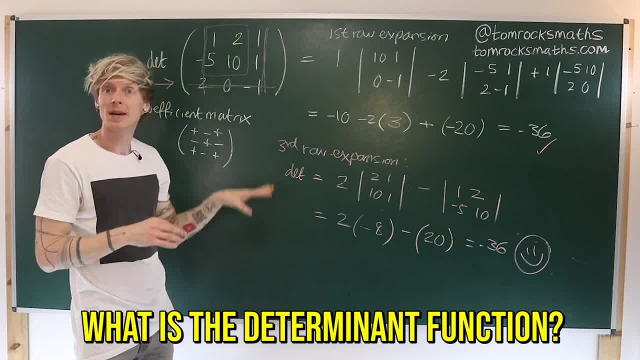 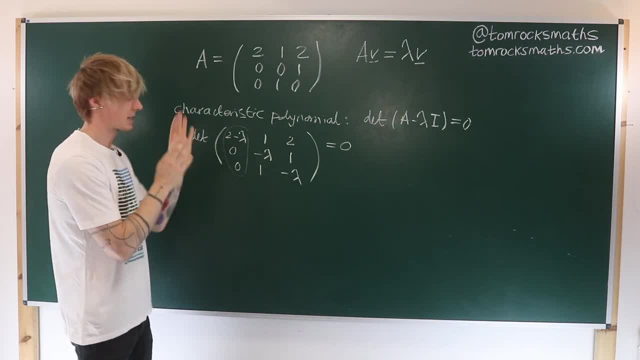 I think this was video 2 or 3.. In the Oxford Linear Algebra series And we said that when you have lots of zeros in a row or column, it's a good idea to expand in that row or column because it simplifies the computation. 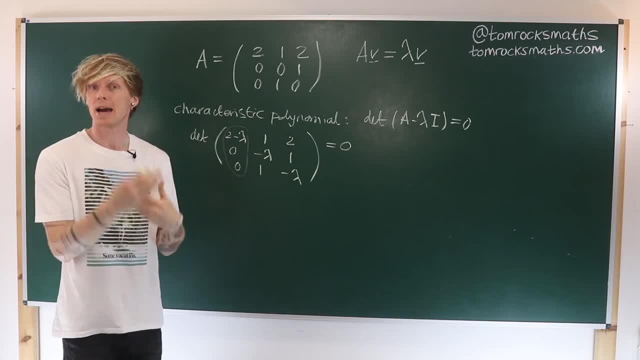 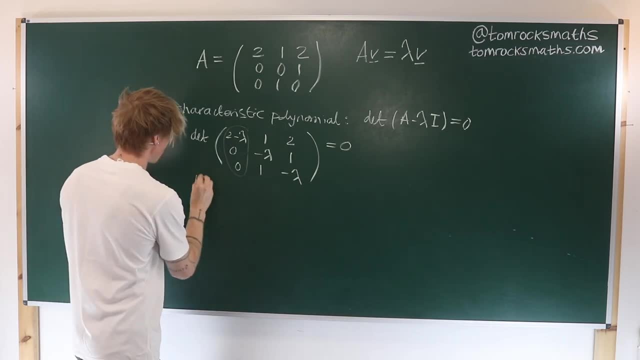 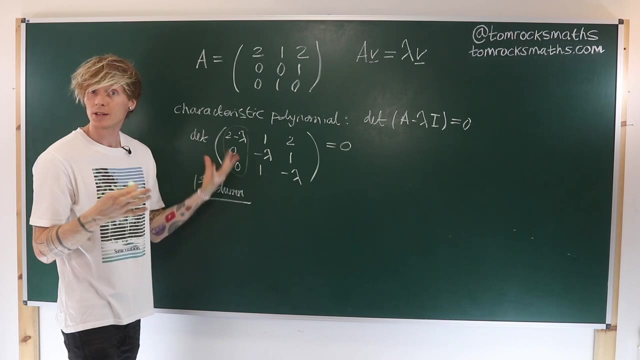 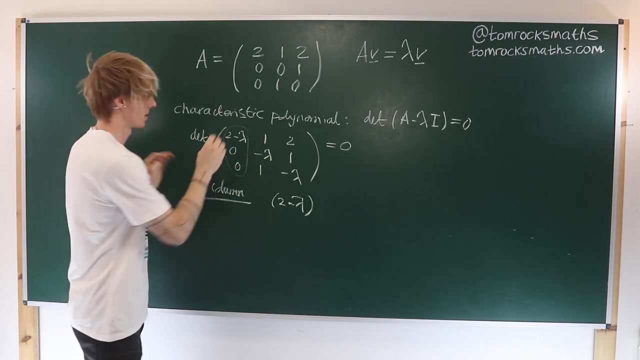 it's a good idea to expand in that row or column because it simplifies the computation. So if we expand in the first column, then we only actually have one non-zero term And that's 2 minus lambda, which is then multiplied, crossing those off. 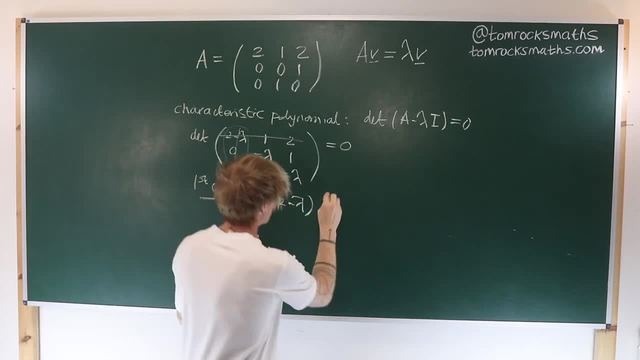 by the remaining 2x2 determinant. So, multiplied by the 2x2, which is minus lambda, 1,, 1, and minus lambda, And we need that to be equal to 0. So, expanding this out, we've got 2 minus lambda. 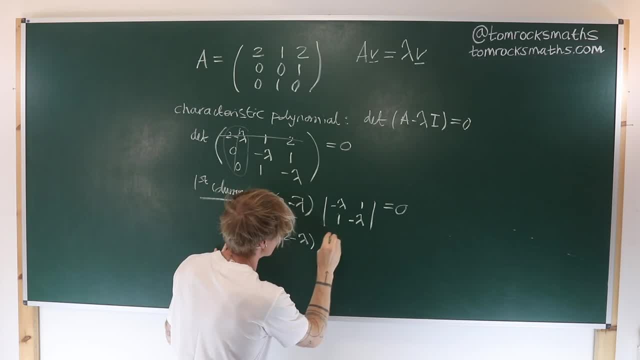 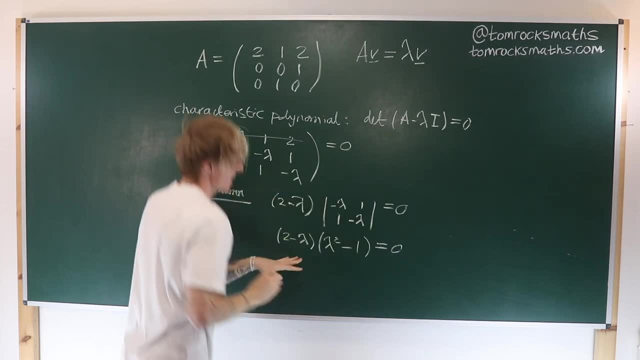 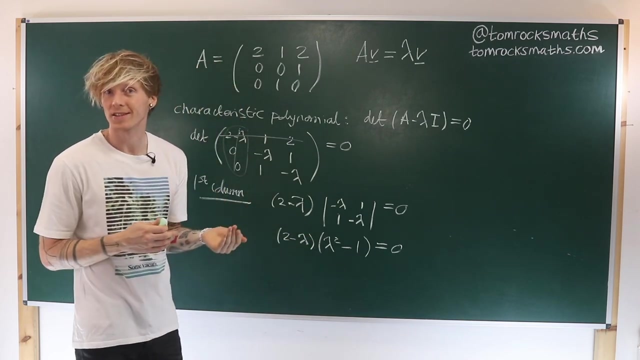 We've then got minus lambda times minus lambda. So that's going to give me a lambda squared minus 1 times 1.. So minus 1.. So this is now our characteristic equation, our characteristic polynomial for this particular matrix. Now we can actually see what these solutions are immediately. 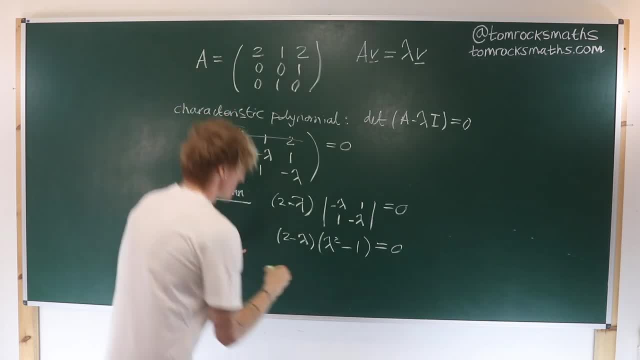 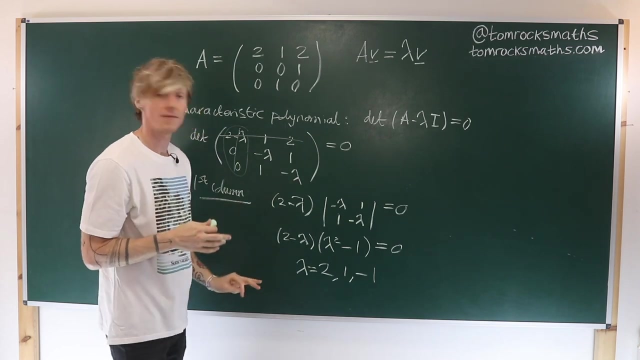 because the equation has already been factorized. So this tells us that lambda is equal to 2, and then we can have plus 1 or minus 1.. So we get three eigenvalues because we have a 3x3 matrix: Three eigenvalues, and exactly as in the previous example, 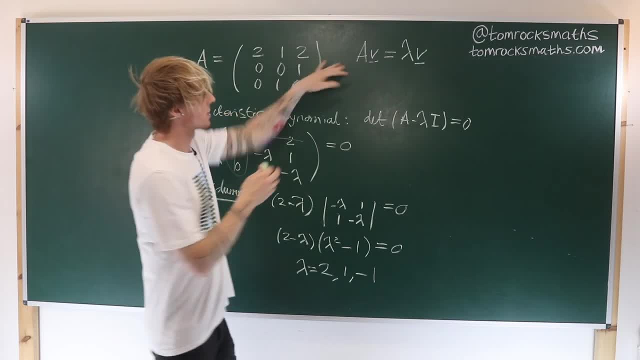 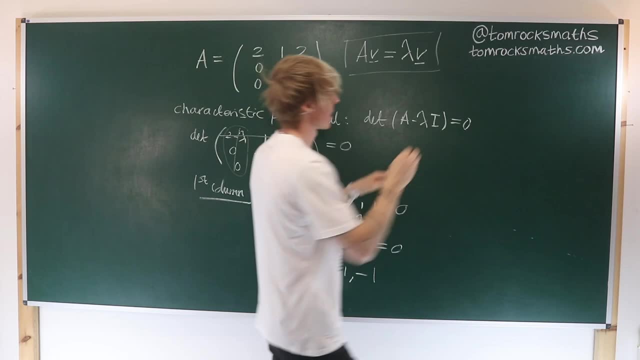 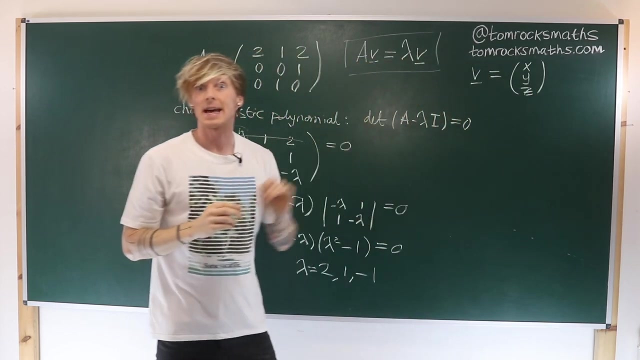 we now take these in turn, substitute them into our original equation and solve for the eigenvector v where, remember, now v will be a general 3 vector, So it will be x, y and z, Starting with lambda, equals 2,. 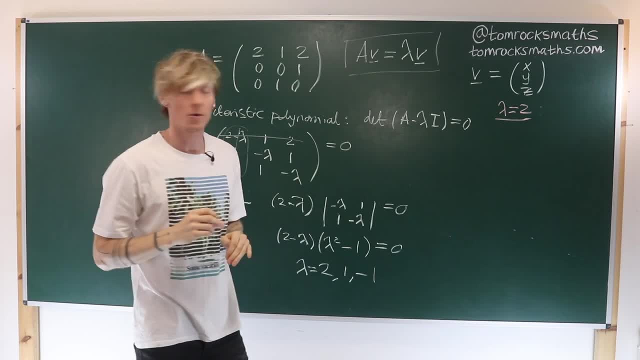 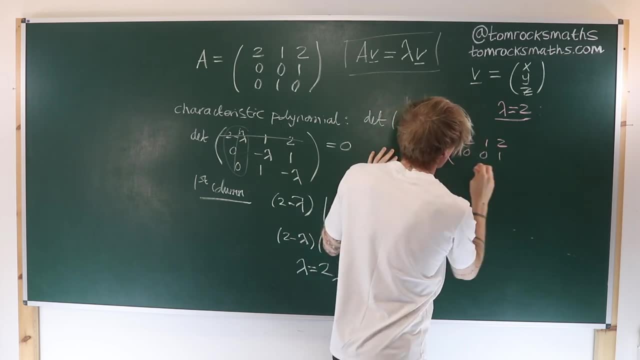 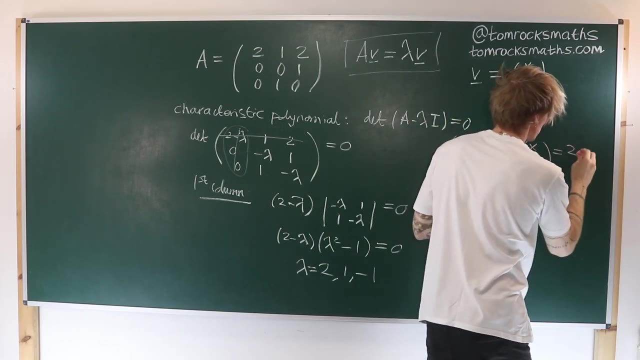 we now substitute into our equation and we have to solve 2, 1,, 2, 0, 0, 1, 0, 1, 0, times x, y, z has to be equal to 2, lots of. 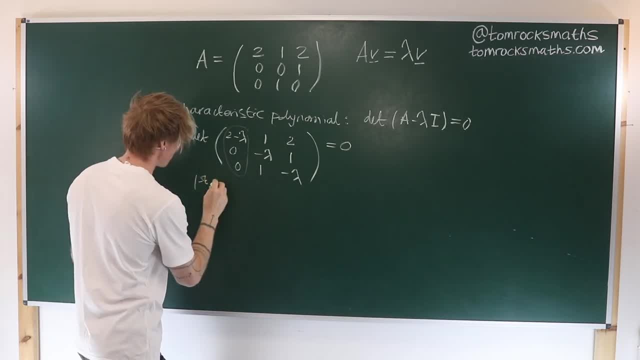 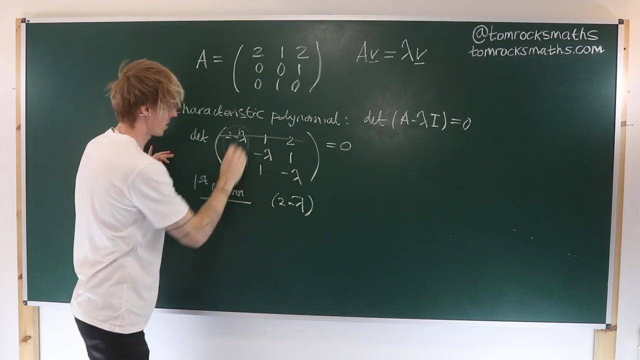 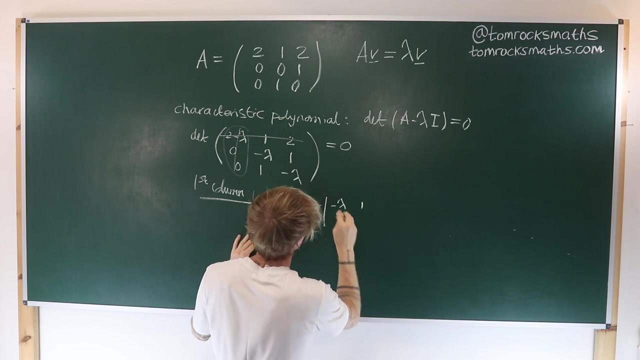 So if we expand in the first column, then we only actually have one nonzero term, And that's 2 minus lambda, which is then multiplied, crossing those off, by the remaining 2 by 2 determinant. So multiplied by the 2 by 2, which is minus lambda, 1, 1, and minus lambda. 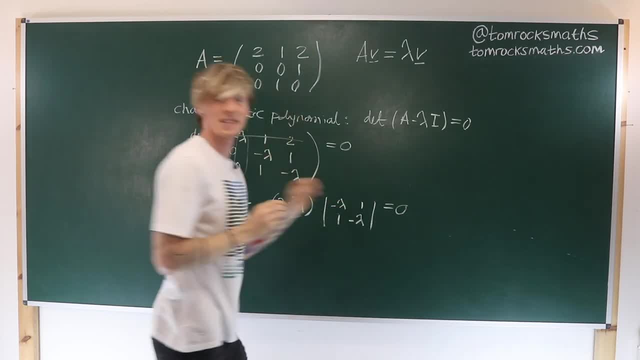 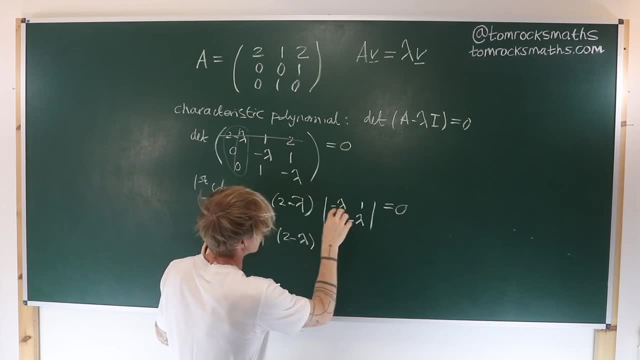 And we need that to be equal to 0.. So, expanding this out, we've got 2 minus lambda. We've then got minus lambda times minus lambda, So that's going to give me a lambda squared minus 1 times 1.. 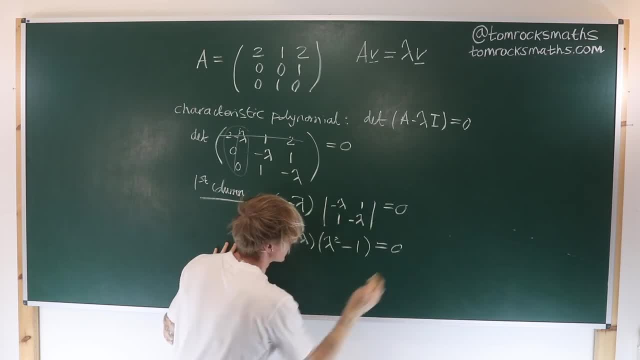 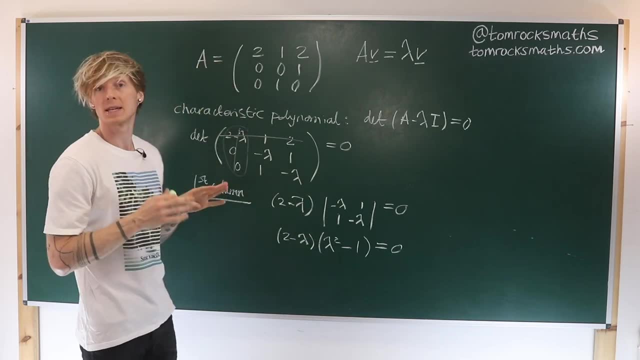 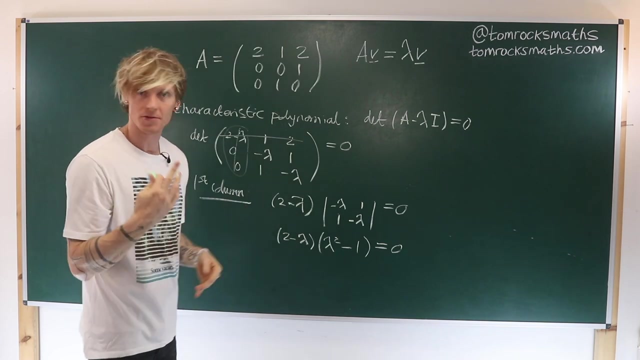 So minus lambda Plus 1.. So this is now our characteristic equation, our characteristic polynomial for this particular matrix. Now we can actually see what these solutions are immediately, because the equation has already been factorised. So this tells us that lambda is equal to 2. 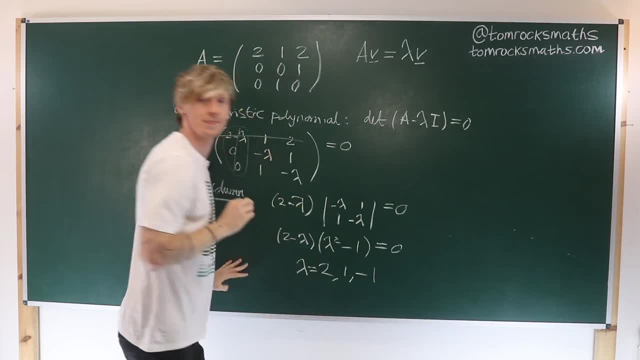 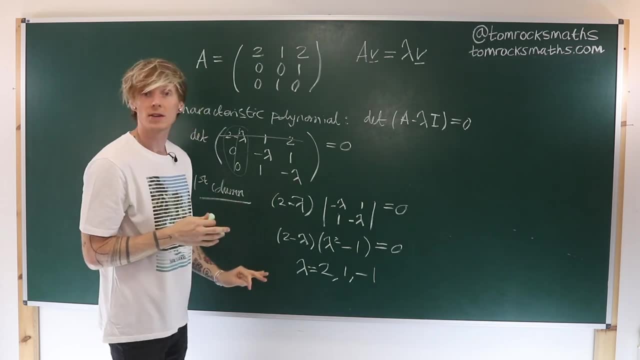 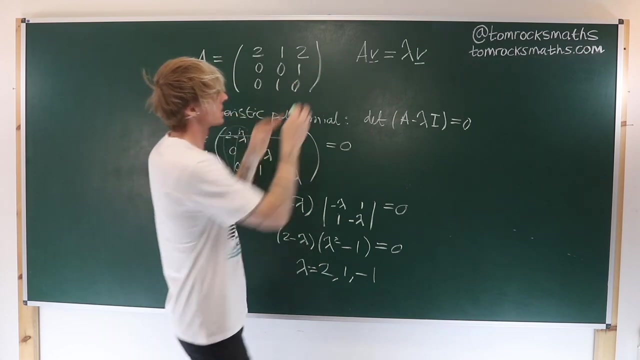 and then we can have plus 1 or minus 1.. So we get 3 eigenvalues, because we have a 3 by 3 matrix, 3 eigenvalues and, exactly as in the previous example, we now take these in turn, substitute them into. 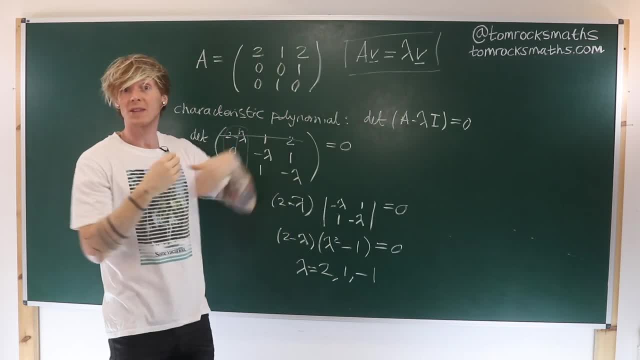 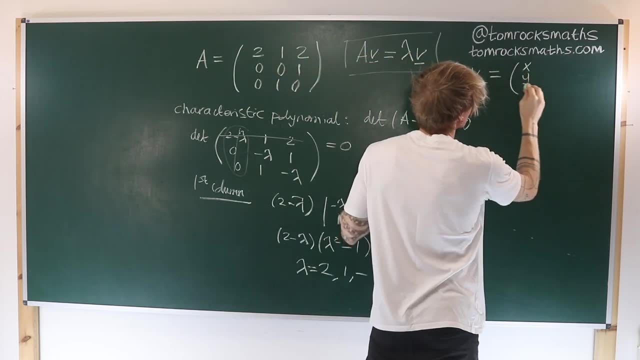 our original equation and solve for the eigenvector v where, remember, now v will be a general 3 vector, So it will be x, y and z, Starting with lambda equals 2,. we now substitute into our equation And we have to solve. 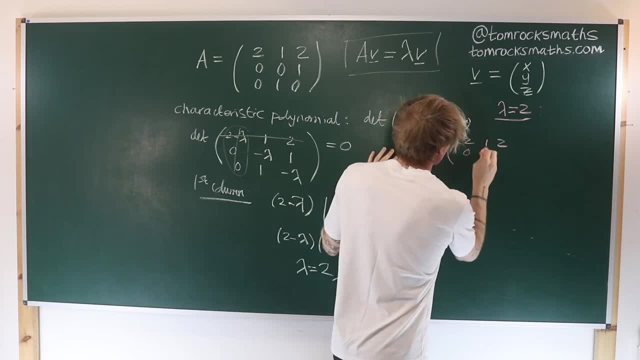 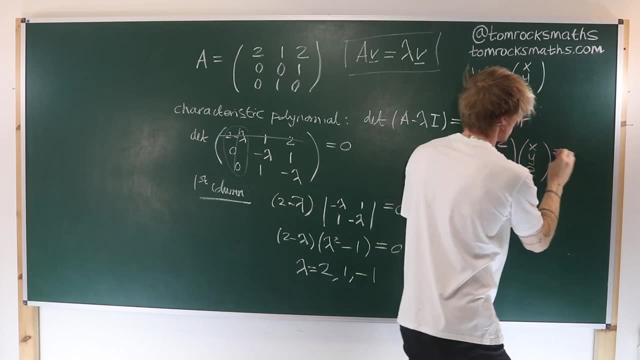 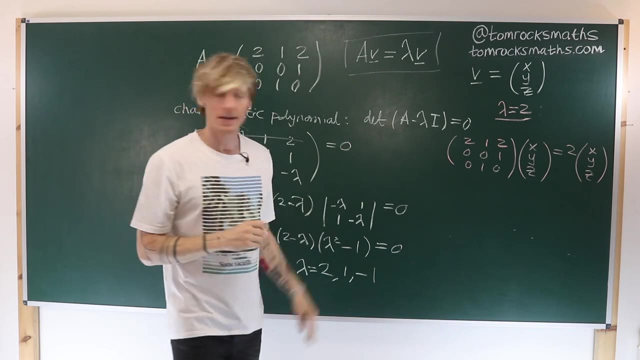 2, 1, 2, 0, 0, 1, 0, 1, 0 times x y z has to be equal to 2 lots of x y z Again. we now expand row by row. 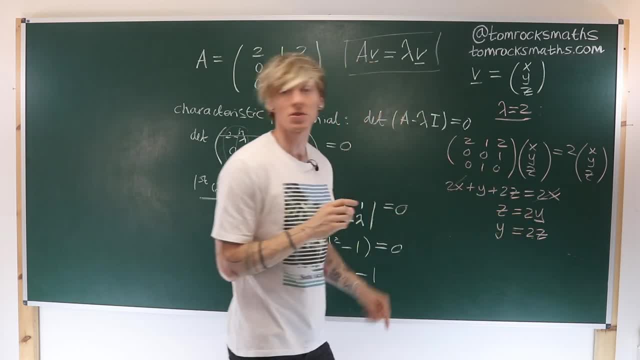 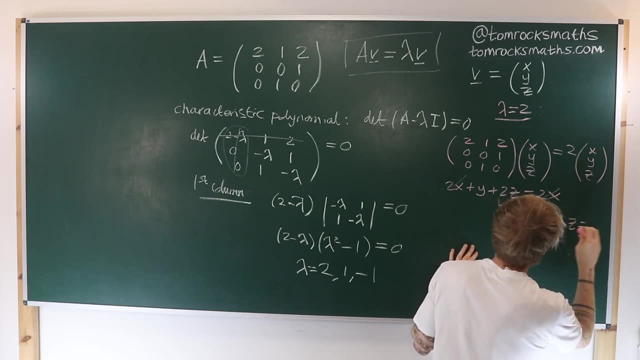 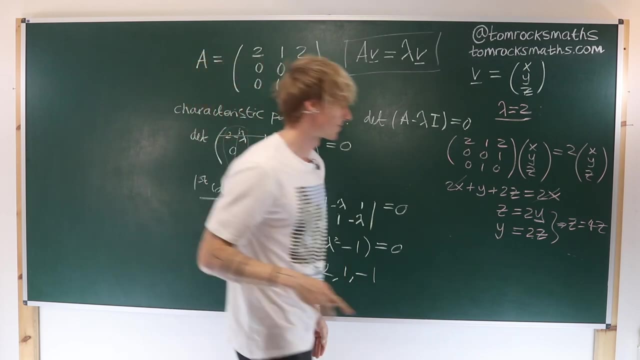 Now, if we take the third equation- y equals 2z- and substitute into the equation above, this will actually tell us that z has to equal 4z. So the only way that can be true is if z is 0.. So this tells us that z is 0. 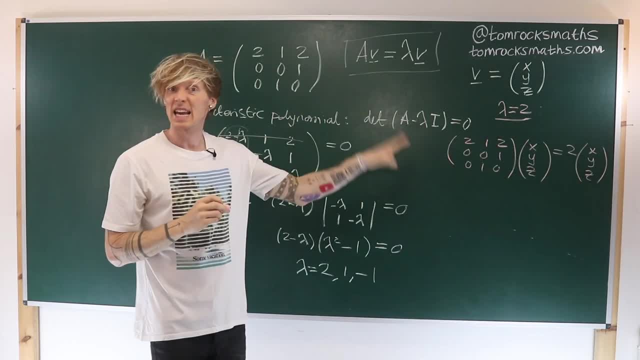 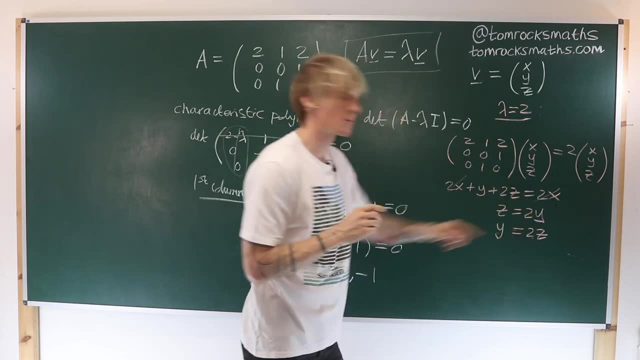 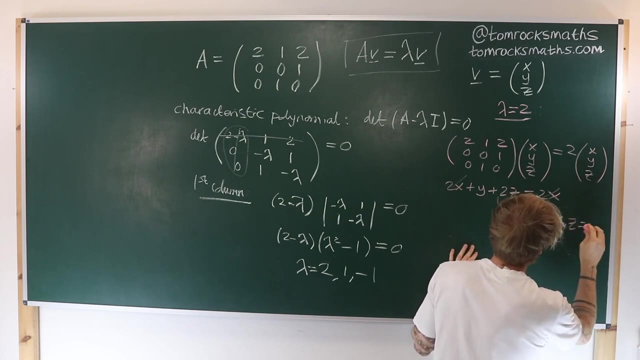 x, y, z. Again, we now expand row by row. Now, if we take the third equation- y equals 2z- and substitute into the equation above, this will actually tell us that z has to equal 4z, So the only way that can be true. 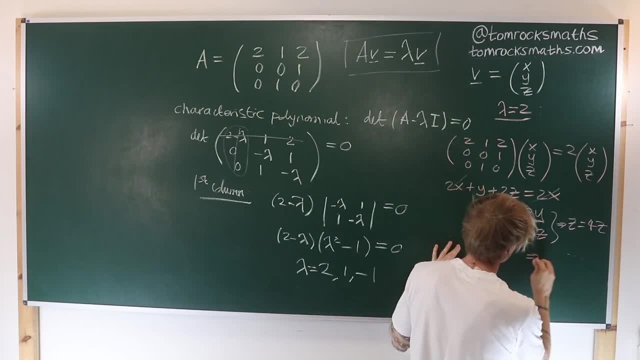 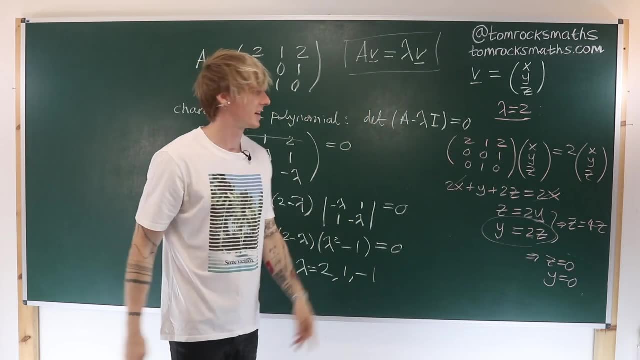 is if z is 0. So this tells us that z is 0, but then y is 2, lots of that. so y is also 0. And then, going back to our original equation, y plus 2z is also 0. 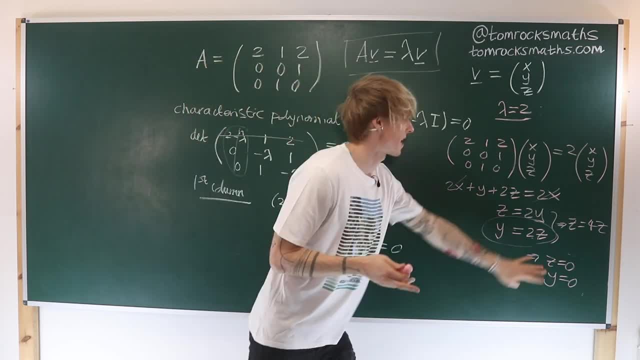 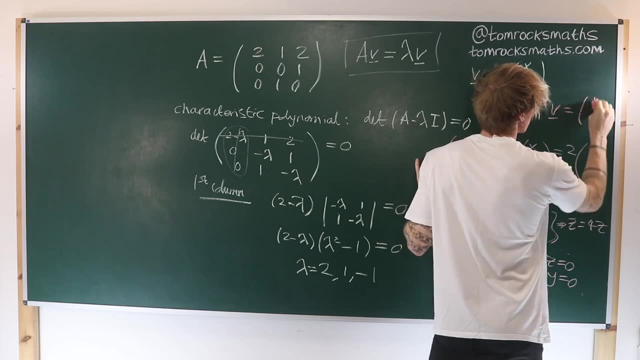 So x is undetermined, y and z both have to be 0. So our eigenvector, writing it as simply as possible, is going to be 1, 0, 0. We have to have y and z being 0,. 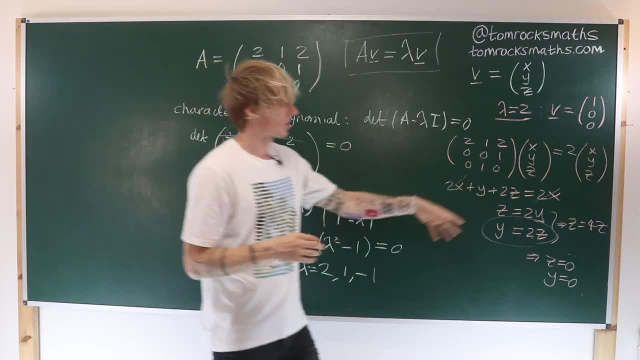 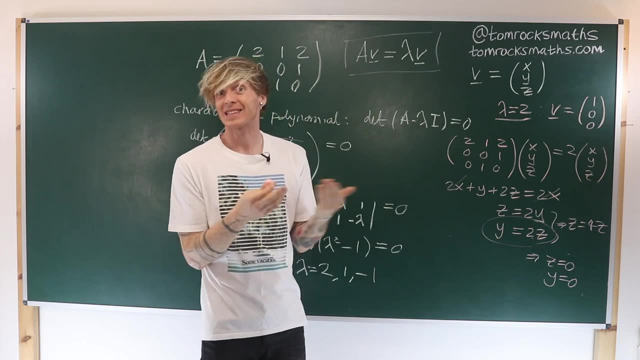 otherwise the equations are contradictory and we can't have that. So they have to be 0.. x can be anything. Let's just pick it to be 1 to make it nice and easy, and so we actually get the unit vector along the x-axis. 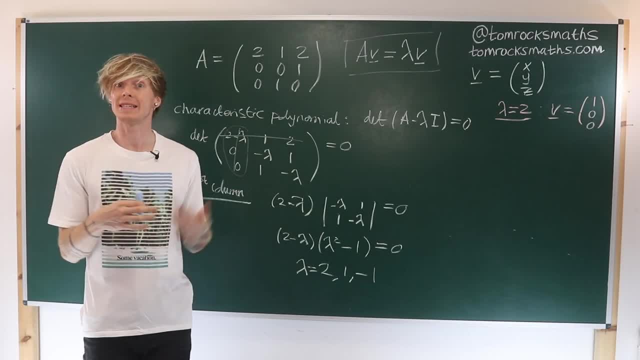 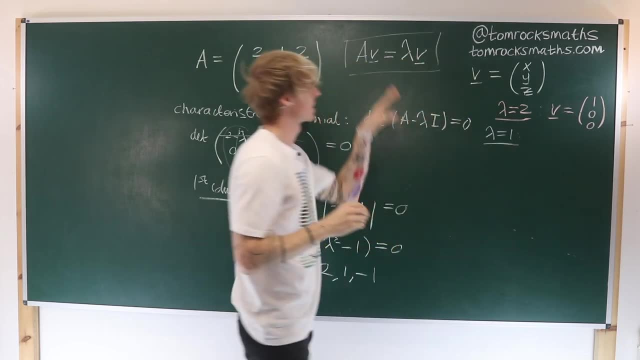 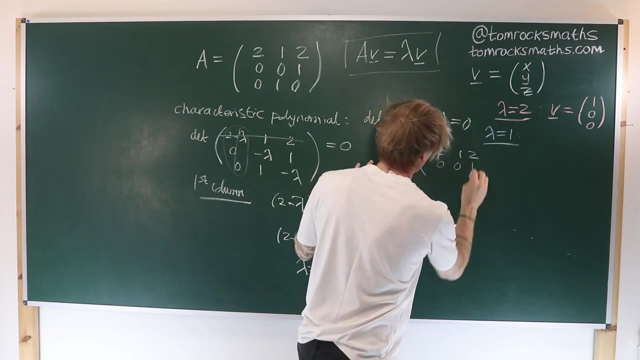 We do the same for the next eigenvalue, which here is lambda equals 1.. So when lambda equals 1, we substitute into our equation. So we have 2, 1,, 2, 0,, 0, 1,. 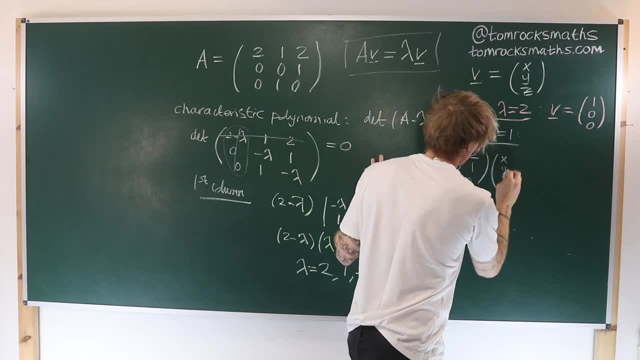 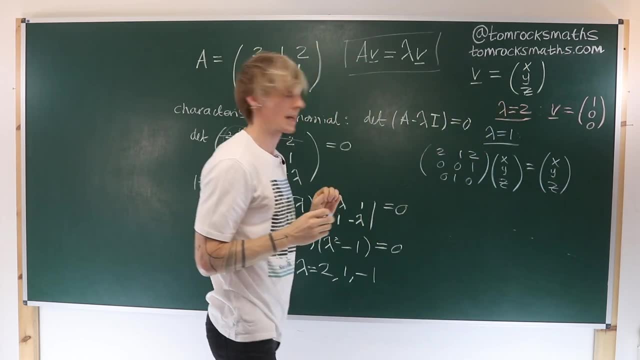 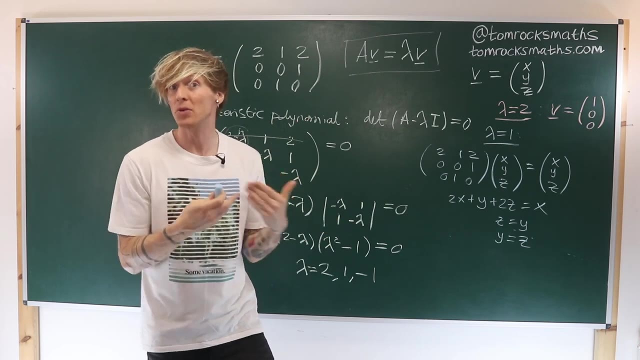 0, 1, 0, times x y z needs to be equal to 1 times x y z, expanding that out. So the last two equations are now consistent. We saw last time they weren't, which meant both variables have to be 0. 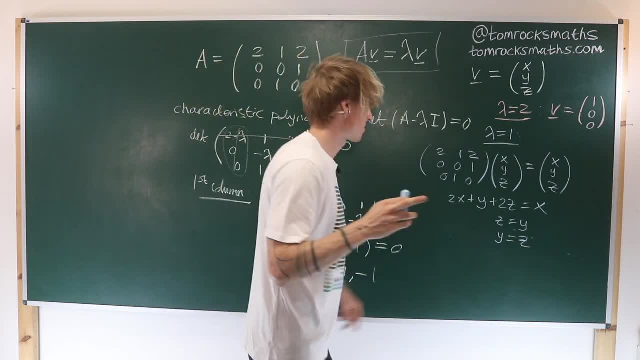 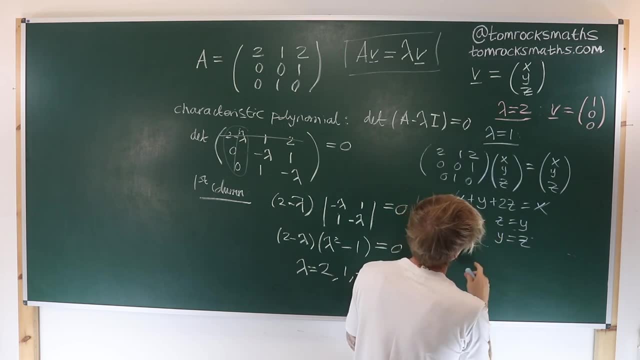 These are now actually telling us the same thing, and so we substitute that into our top equation and subtract an x from both sides. We can now say that y plus 2y plus x has to be equal to 0. So we can say that x is in fact equal. 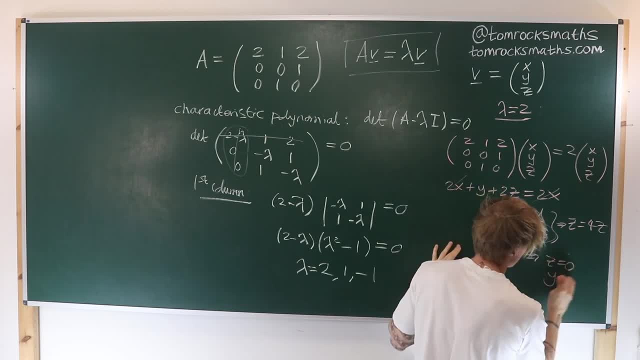 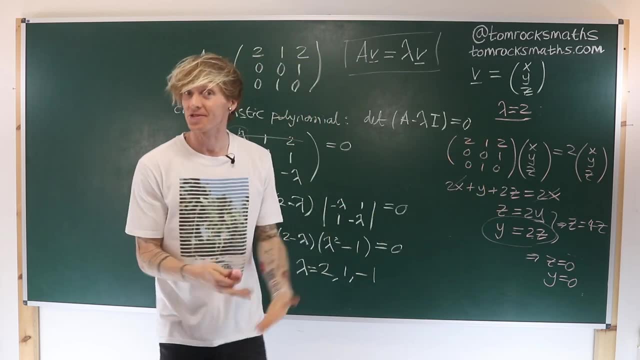 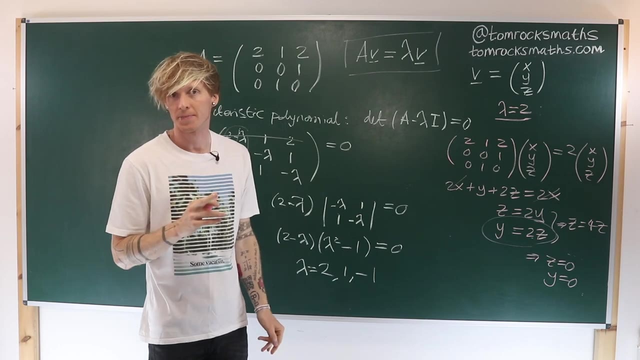 But then y is 2- lots of that. So y is also 0.. And then, going back to our original equation, y plus 2z is also 0. So x is undetermined. y and z both have to be 0.. 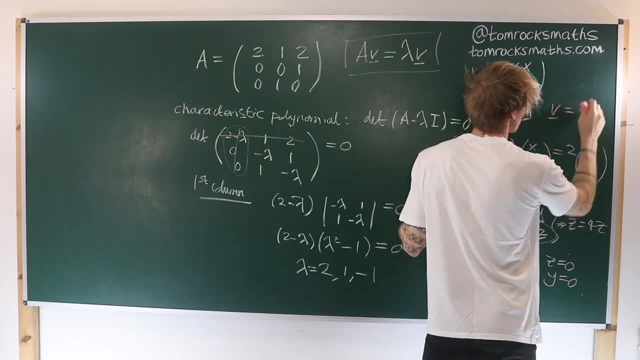 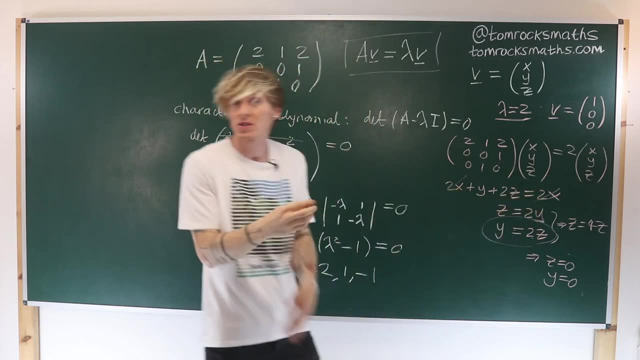 So our eigenvector, writing it as simply as possible, is going to be 1, 0, 0. We have to have y and z being 0, otherwise the equations are contradictory and we can't have that, So they have to be 0. 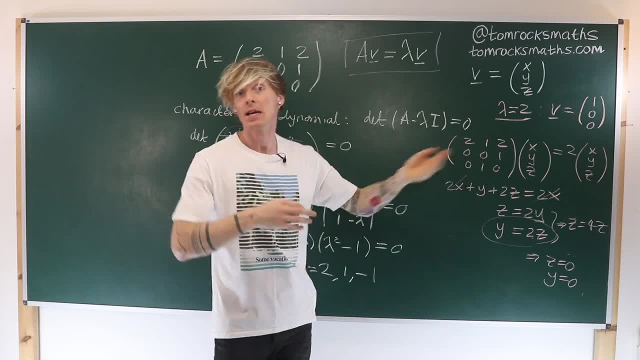 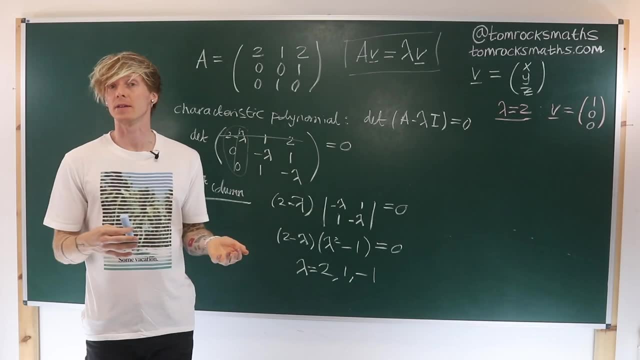 x can be anything. let's just pick it to be 1 to make it nice and easy, and so we actually get the unit vector along the x axis. We do the same for the next eigenvalue, which here is lambda- equals 1.. 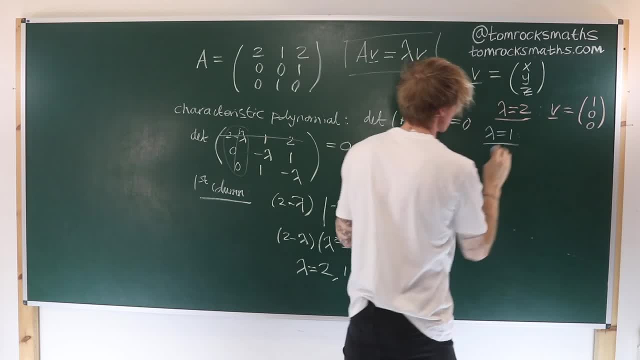 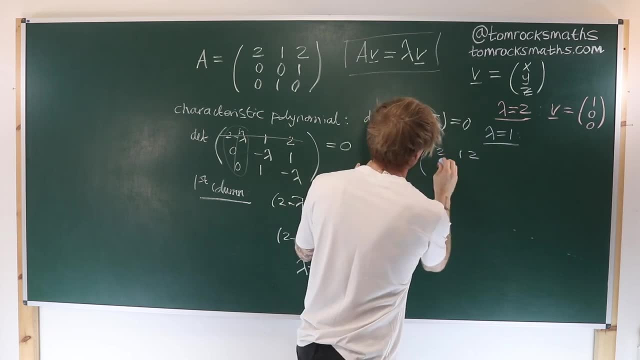 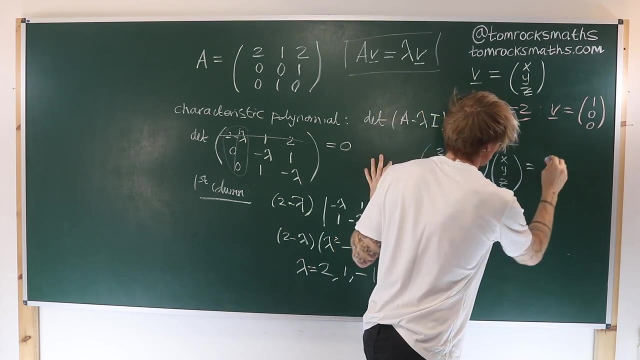 So when lambda equals 1, we substitute into our equation. So we have 2, 1, 2, 0, 0, 1, 0, 1, 0 times x y z needs to be equal to 1 times x y z. 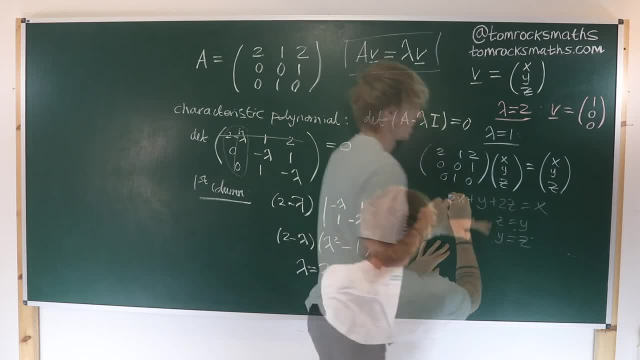 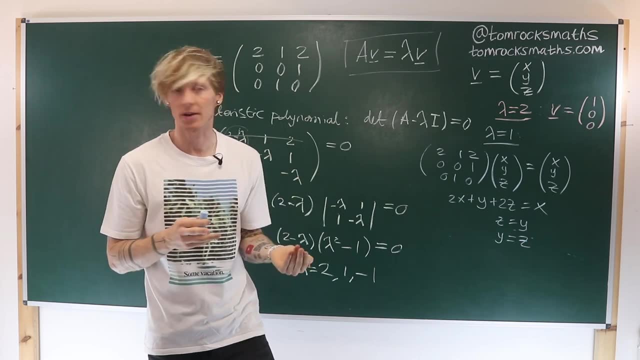 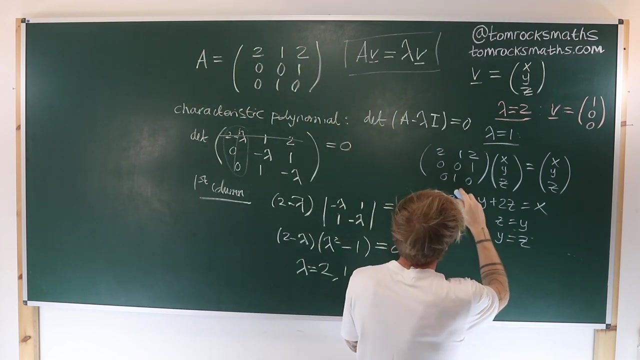 expanding that out. So the last two equations are now consistent. We saw last time they weren't, which meant both variables had to be 0. These are now actually telling us the same thing, and so we substitute that into our top equation and subtract an. 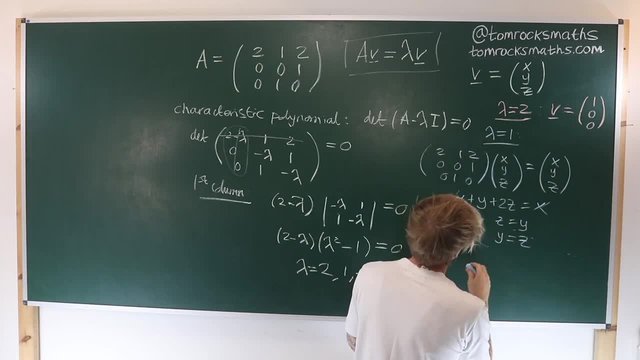 x from both sides. We can now say that y plus 2y plus x has to be equal to 0. So we can say that x is in fact equal to minus 3y, which is the same as minus 3z, As. 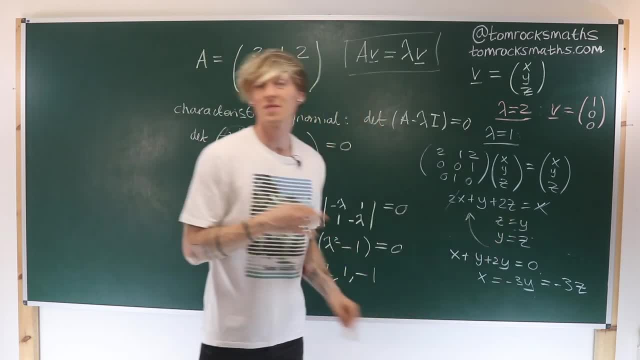 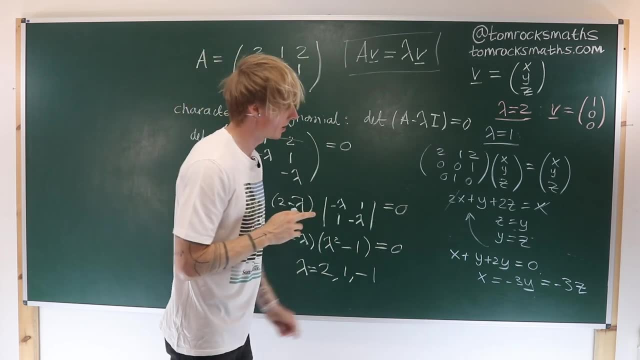 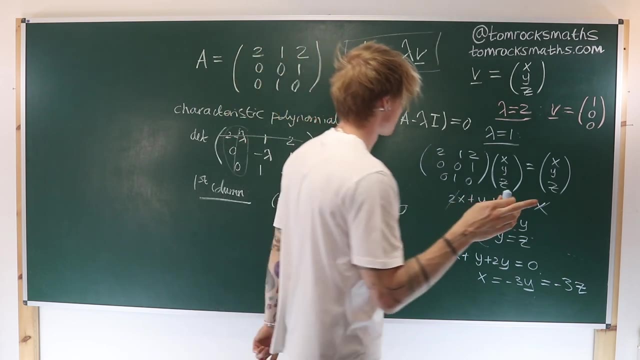 before. we are free to choose the value of each of these variables, provided this equation remains satisfied. So I think here picking y and z to both be minus 1 is going to be helpful. So for v, if I pick y to be minus 1 and z to be minus 1, 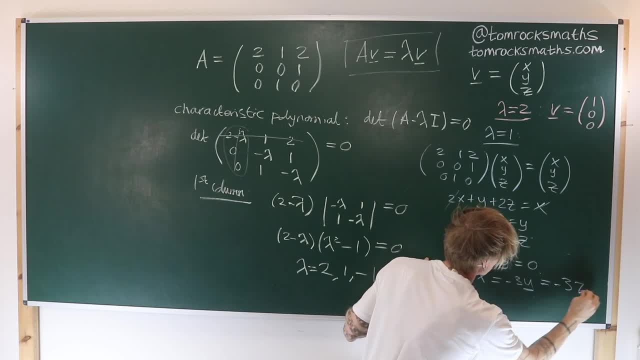 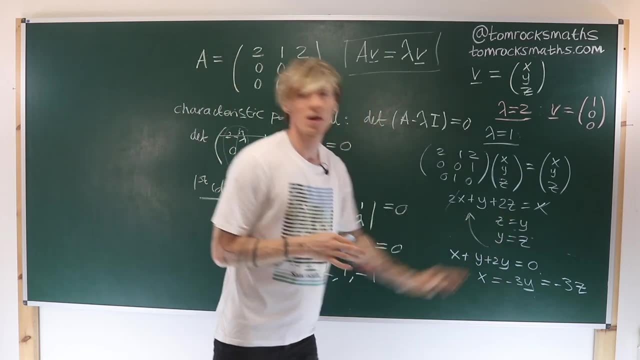 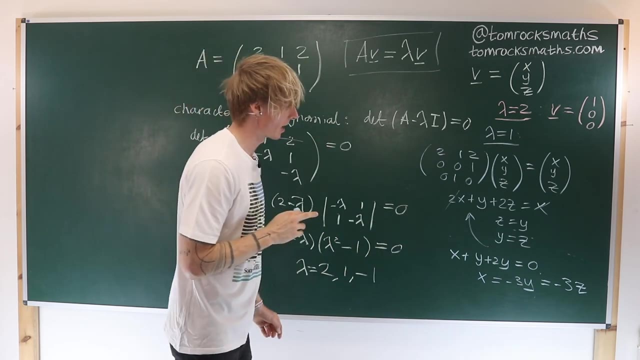 to minus 3y, which is the same as minus 3z. As before, we are free to choose the value of each of these variables, provided this equation remains satisfied. So I think here picking y and z to both be minus 1. 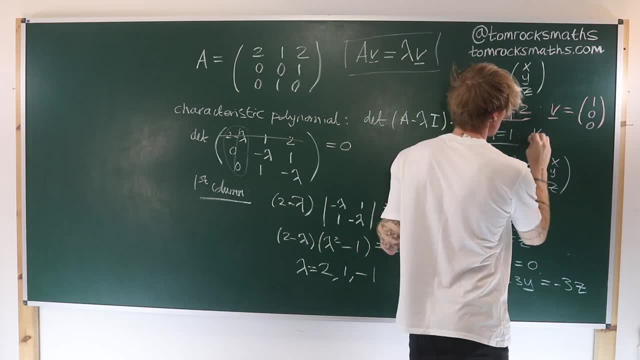 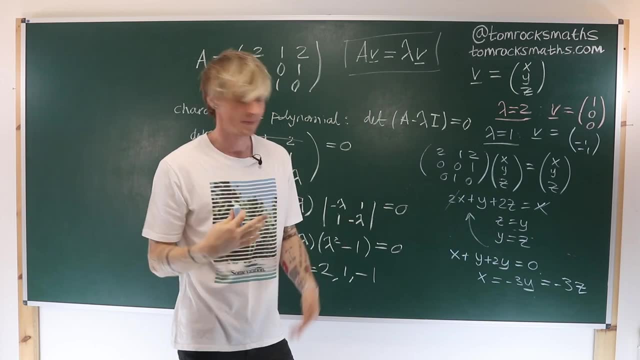 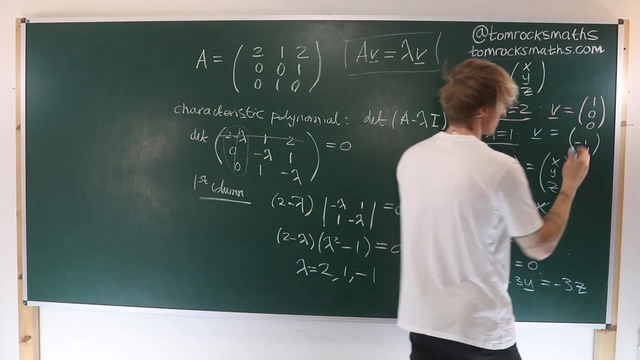 is going to be helpful. So for v, if I pick y to be minus 1 and z to be minus 1, then they are certainly equal. And I've now got that x is equal to minus 3 times y, So minus 3 times minus 1. 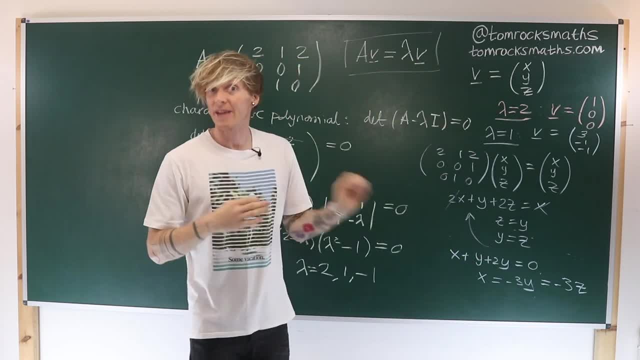 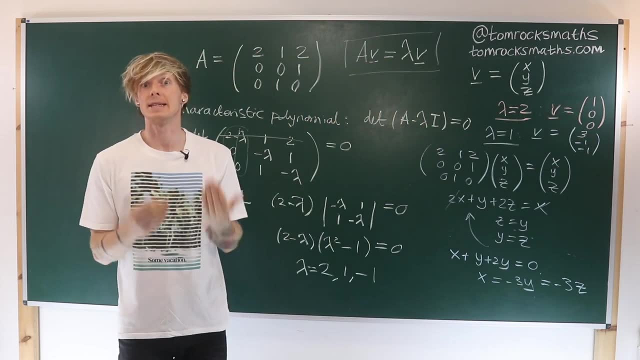 gives me 3.. So the eigenvector here is going to be 3 minus 1. minus 1,, which corresponds to the eigenvalue of lambda, is equal to 1.. Finally, for our third eigenvalue, when lambda is minus 1,. 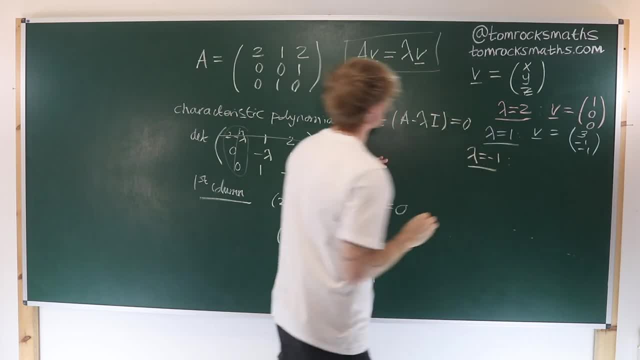 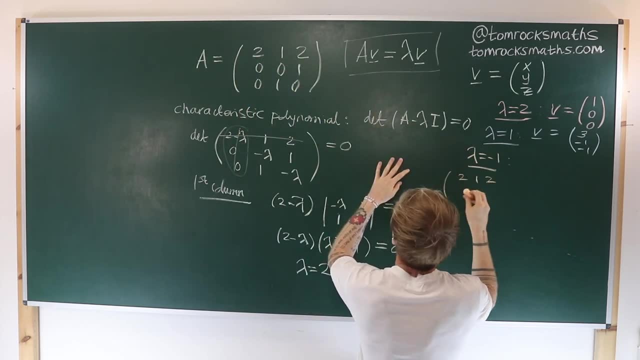 we again substitute into our original equation and we're going to have to solve 2, 1, 2, 0, 0, 1, 0, 1, 0 times x y z equals minus x y z. 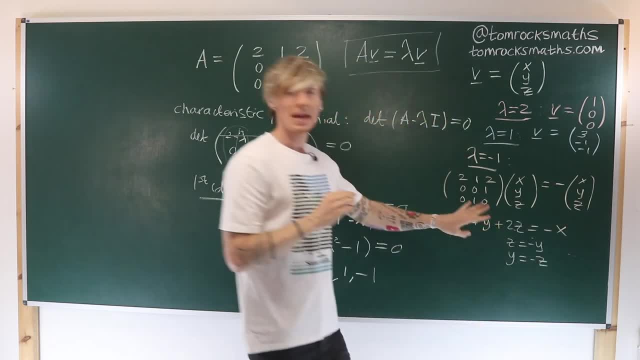 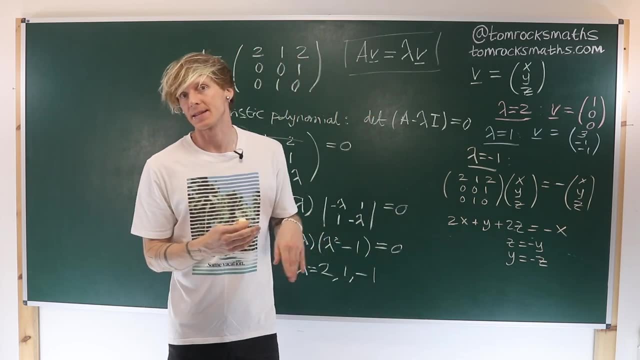 Again. we expand this out Again. these two equations are indeed consistent. It just says that whatever we pick for y, z is the negative of that, and vice versa. So they're fine, Now substituting those into the top equation. 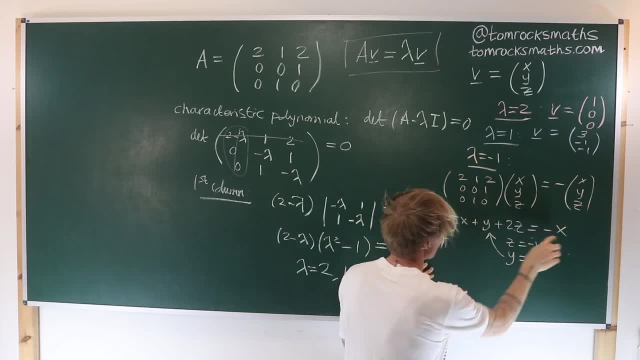 so I'll take this one and plug it in here. I can say: adding the x across 3x plus a y, which is a minus z plus 2z, has to be 0. So I can in fact say that. 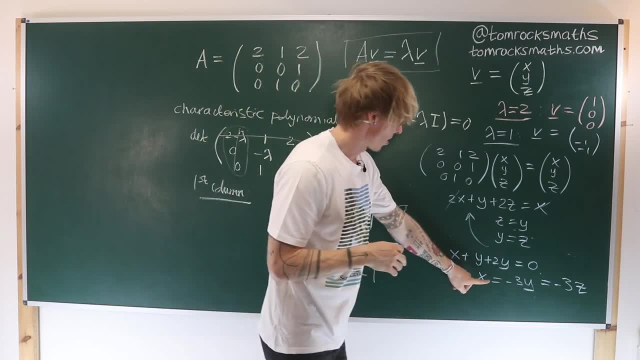 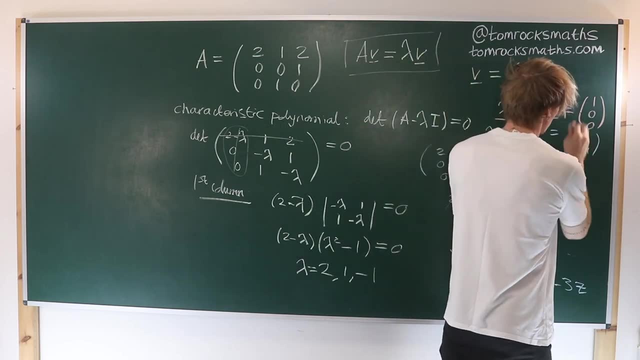 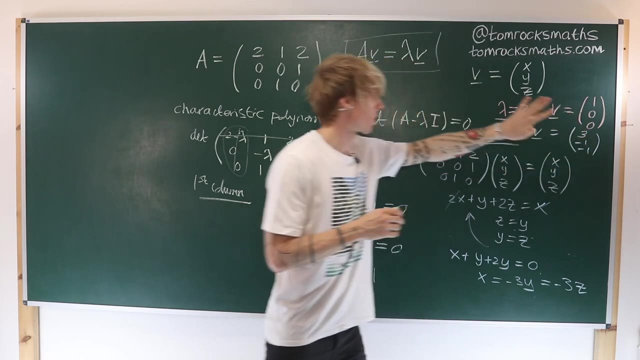 then they are certainly equal. And I've now got the: x is equal to minus 3 times y. So minus 3 times minus 1 gives me 3.. So the eigenvector here is going to be 3 minus 1 minus 1, which corresponds: 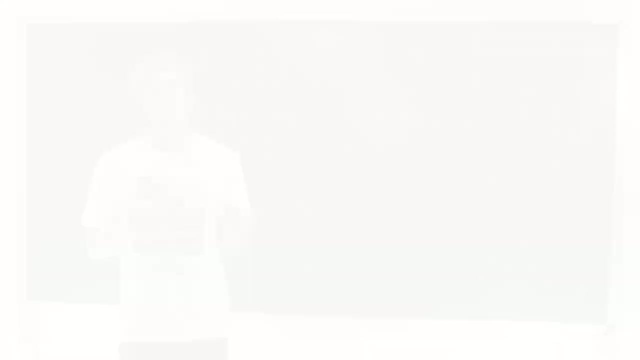 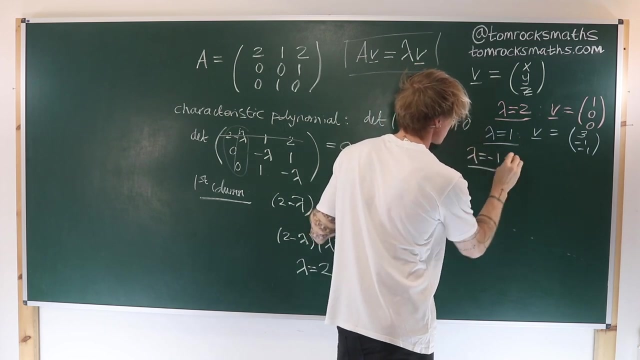 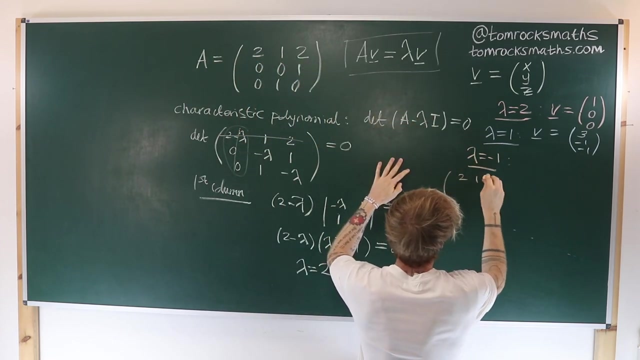 to the eigenvalue of lambda is equal to 1.. Finally, for our third eigenvalue, when lambda is minus 1, we again substitute into our original equation and we're going to have to solve 2, 1, 2, 0, 0, 1. 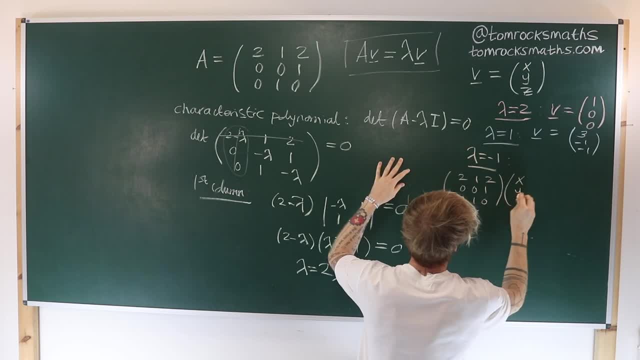 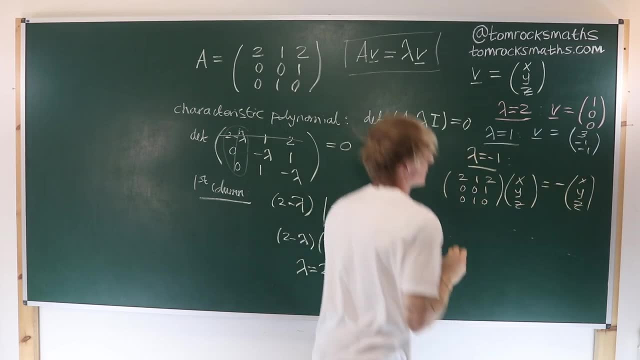 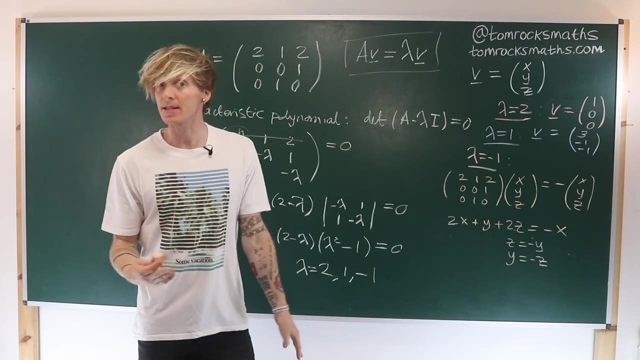 0, 1, 0 times x, y z equals minus x y z Again. we expand this out Again. these two equations are indeed consistent. It just says that whatever we pick for, y z is the negative of that. 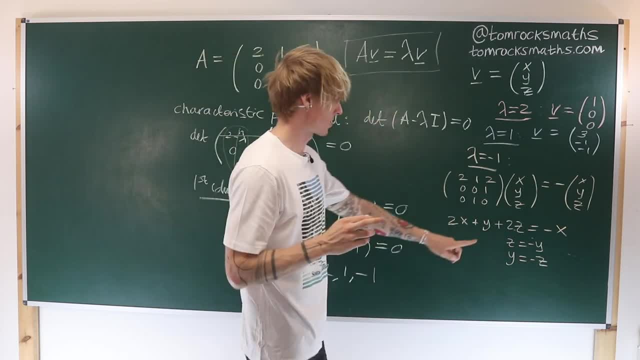 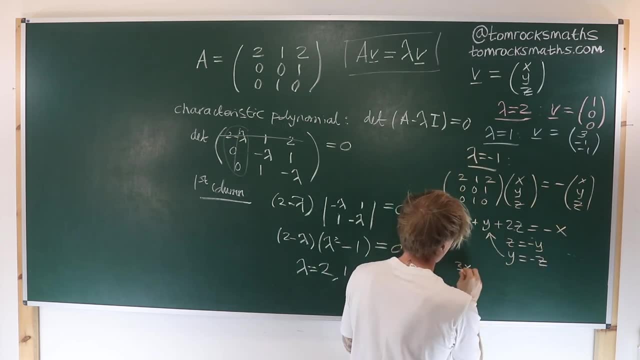 and vice versa. So they're fine Now substituting those into the top equation. So I'll take this one and plug it in here. I can say, adding the x across 3x plus a y, which is a minus z plus 2z, has to be 0.. 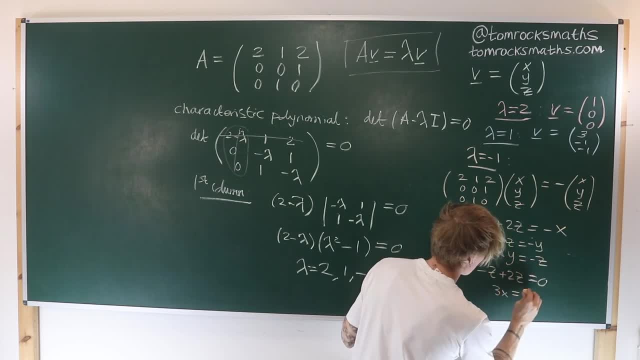 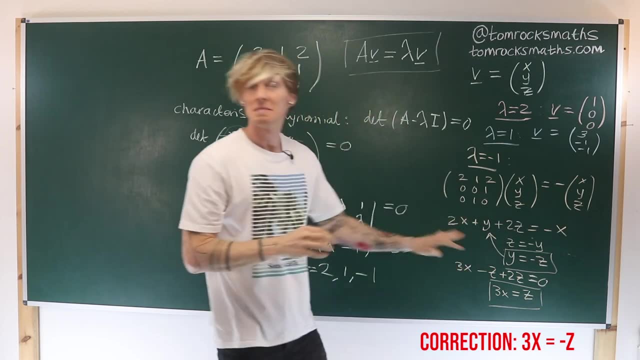 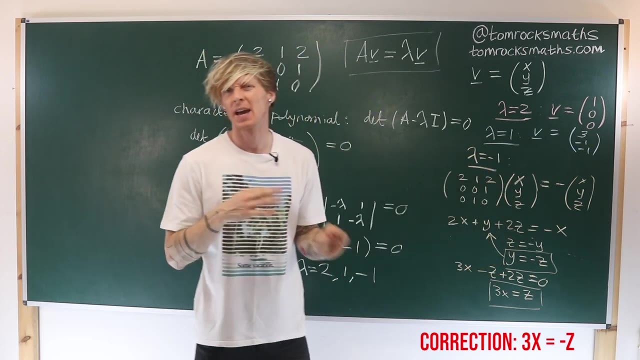 So I can in fact say that 3x has to equal z, and from there I can say y is equal to minus z. So I'm going to start by picking x to be equal to 1 and then making sure I can satisfy both of these equations. So 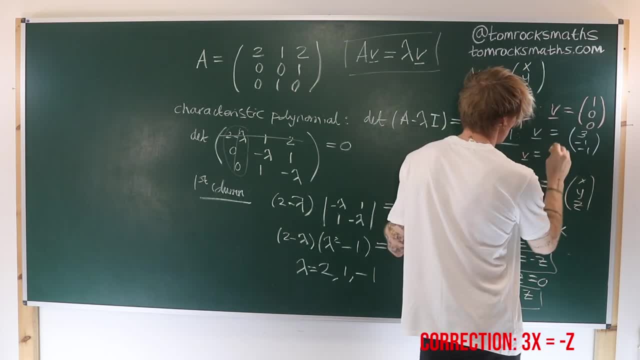 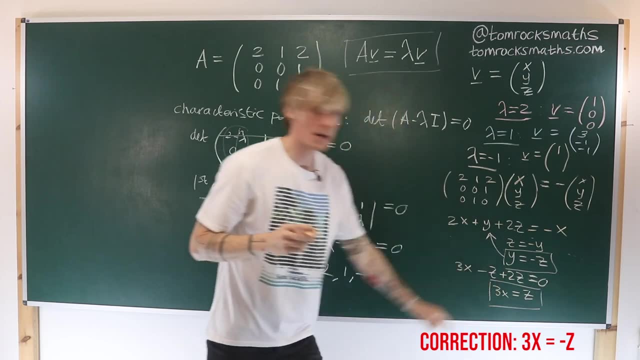 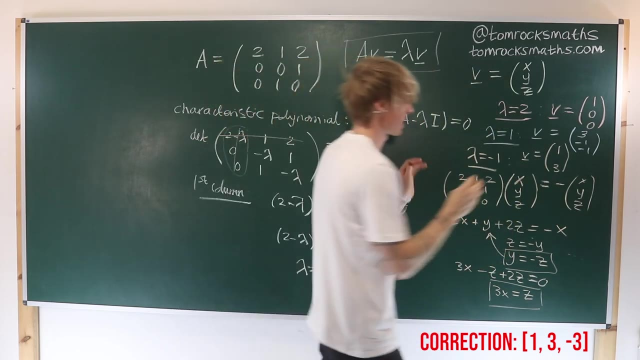 if I pick x to be 1, to hopefully simplify the eigenvector, and we'll see Then, if x is 1, that tells me that z is 3, and then y has to be minus z, so y has to be minus 3.. So for 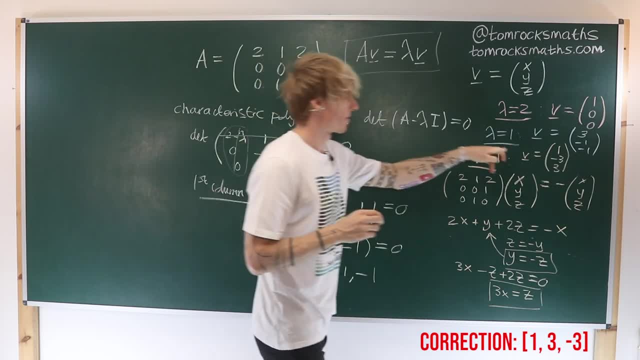 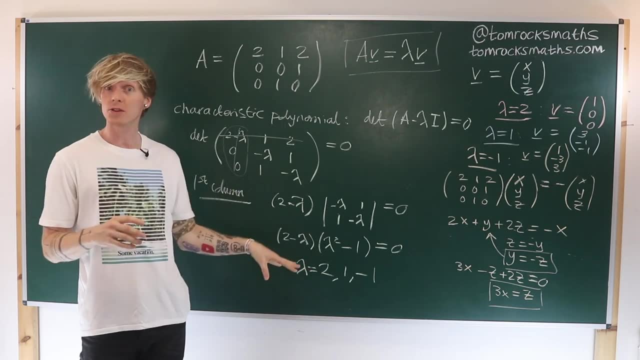 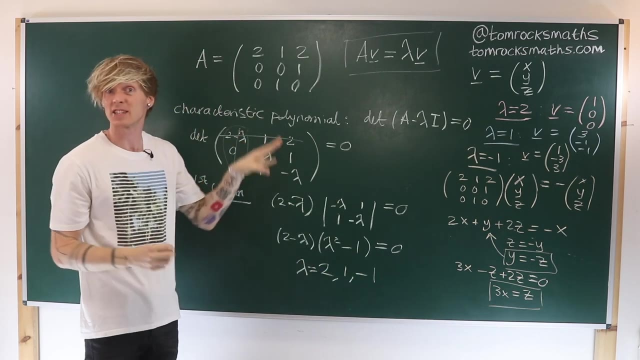 the eigenvalue of minus 1, we get the eigenvector 1 minus 3.. And we're done. We've found three eigenvalues lambda, being 2, 1 and minus 1.. These are the solutions to our characteristic equation or characteristic polynomial. 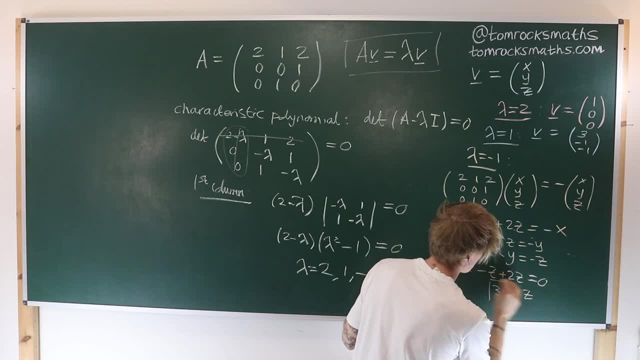 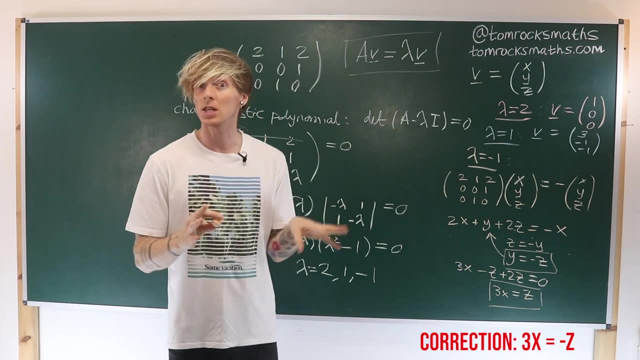 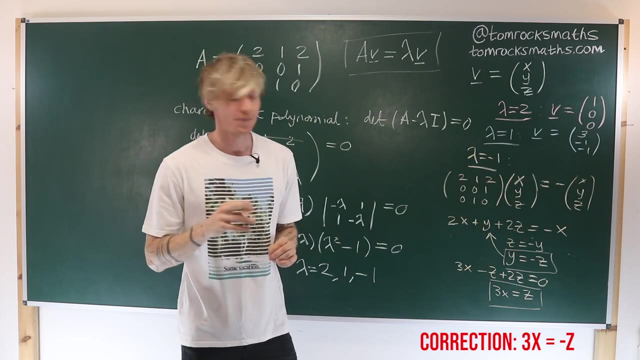 3x has to equal z And from there I can say y is equal to minus z. So I'm going to start by picking x to be equal to 1, and then making sure I can satisfy both of these equations. So if I pick x to be 1, 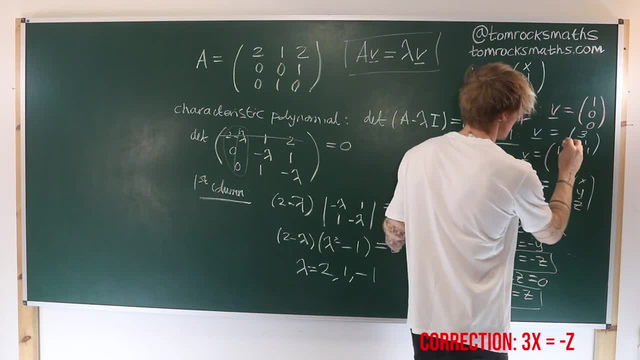 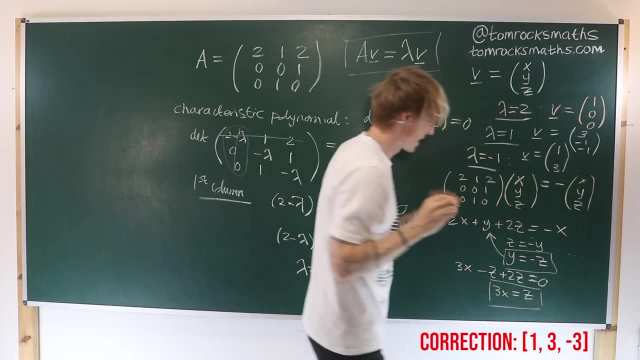 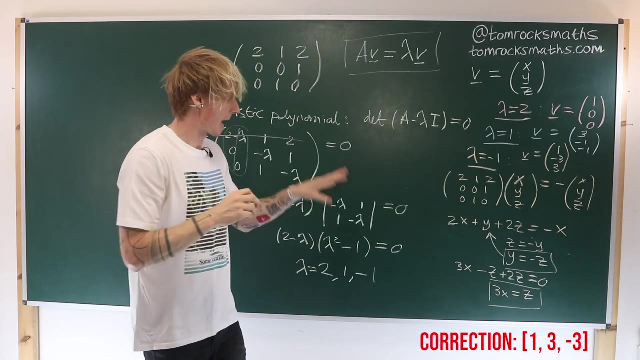 to hopefully simplify the eigenvector, and we'll see then if x is 1, that tells me that z is 3.. And then y has to be minus z, so y has to be minus 3.. So for the eigenvalue, 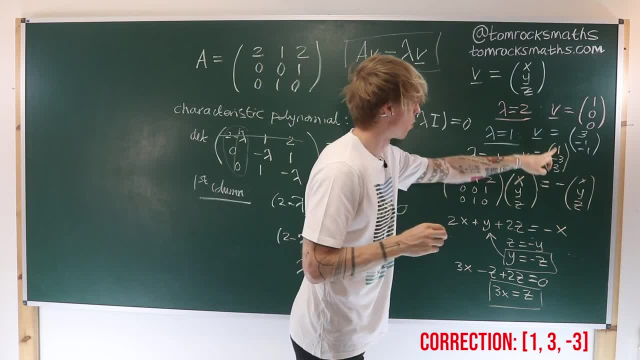 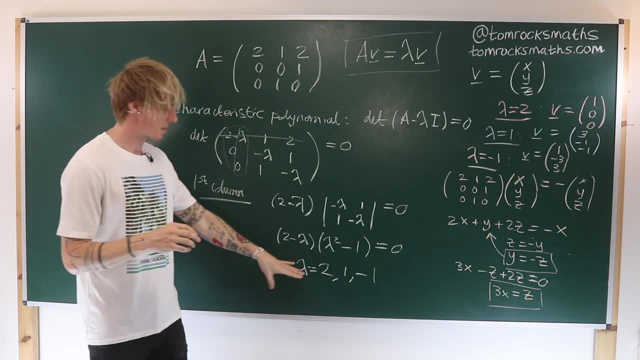 of minus 1, we get the eigenvector 1, minus 3, and 3.. And we're done. We found three eigenvalues lambda, being 2, 1, and 0. These are the solutions to our characteristic equation. 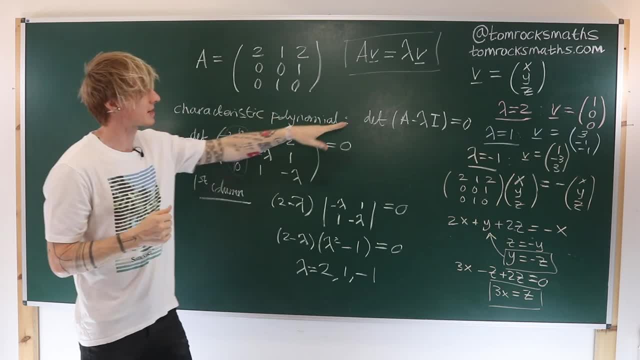 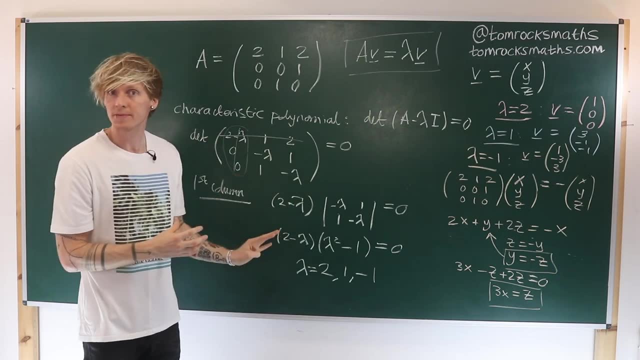 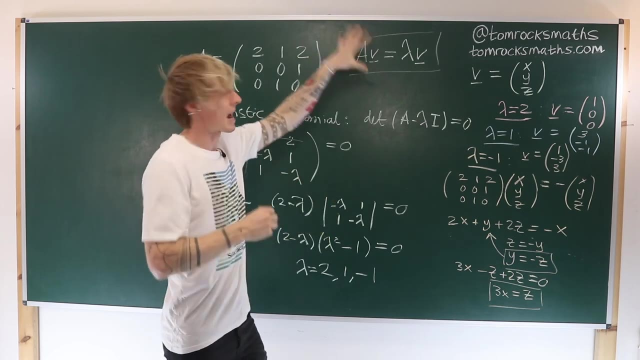 or characteristic polynomial where we solve the determinant of a minus lambda i equal to 0. We found the eigenvalues as the roots of that equation. We've then substituted in to our original expression that we wanted to solve for lambda and v. And now that we know lambda, 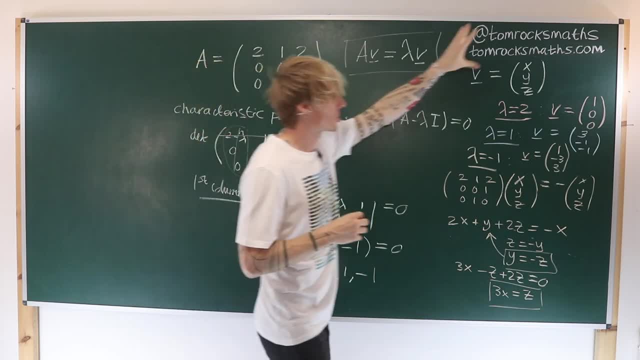 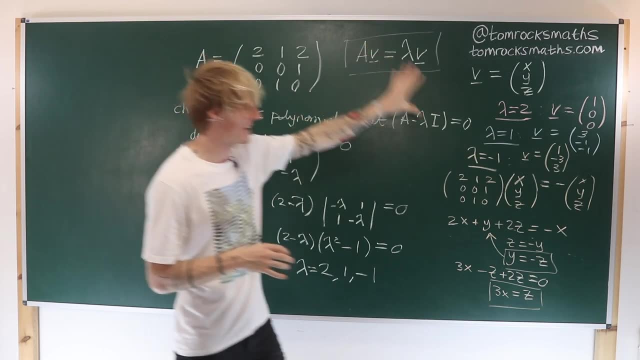 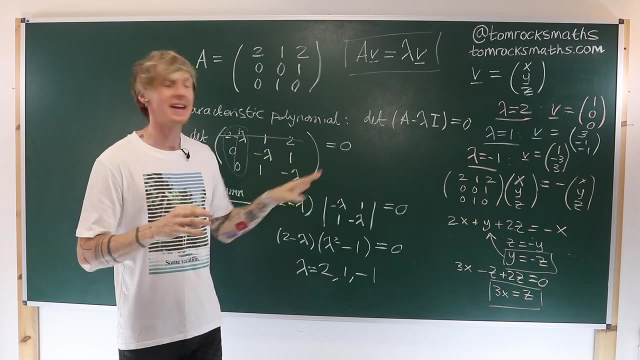 we can substitute in 1 by 1 to find the general form of the eigenvectors. As before, make sure you check your answer. take these values of lambda and v, substitute them into this equation and make sure that I haven't made any algebraic slips. 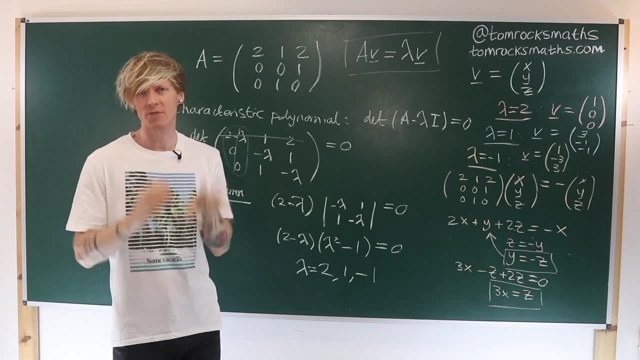 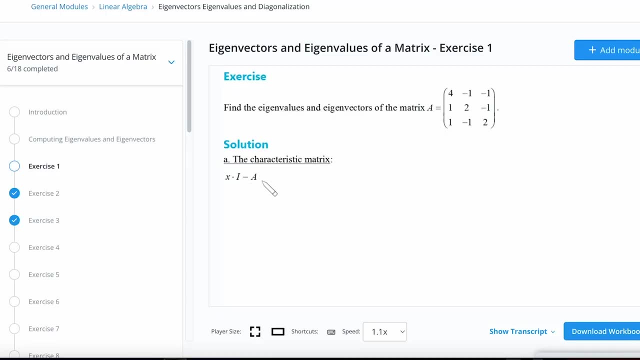 These calculations can be quite complicated, so I really do recommend substituting back in at the end to make sure your solution is correct And for more practice exercises and videos with step-by-step breakdowns of the solutions. once again, I recommend heading over to ProPrep. 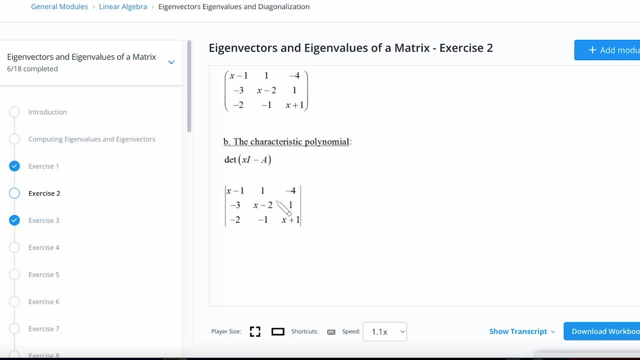 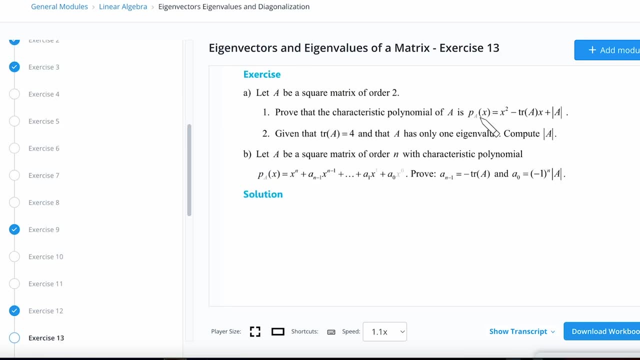 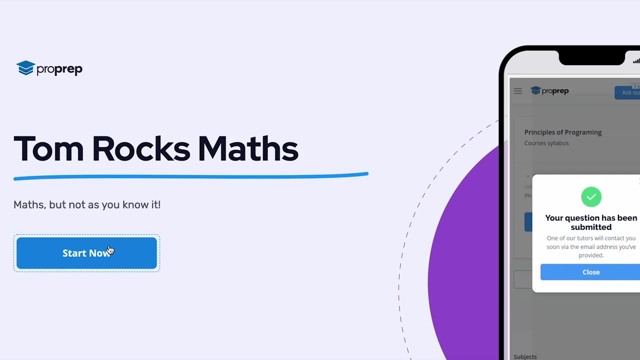 There are 15 exercises for you to check out, beginning with some computational questions similar to those we've looked at here, before moving on to some proofs and a discussion of the properties of the characteristic equation. Remember to sign up using the link in the video description. 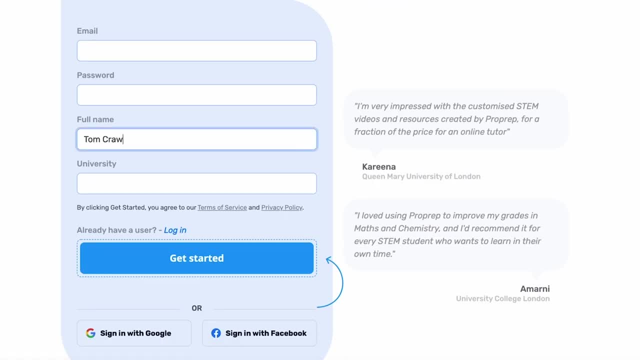 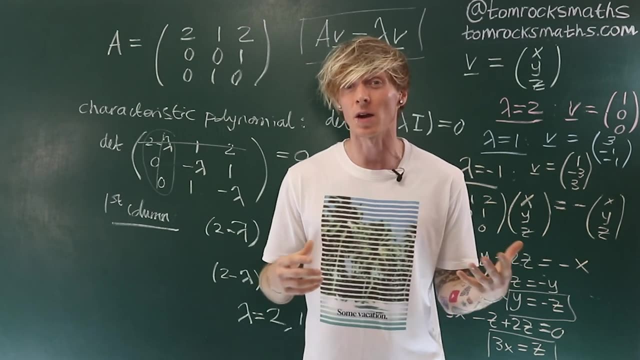 for a 30-day free trial with full access to all of the videos. Thank you, everyone for watching. Please do remember to subscribe to the channel if you've enjoyed the video, and I'll see you all soon, Take care. 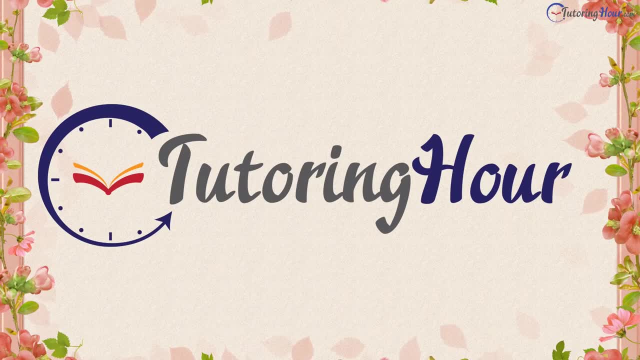 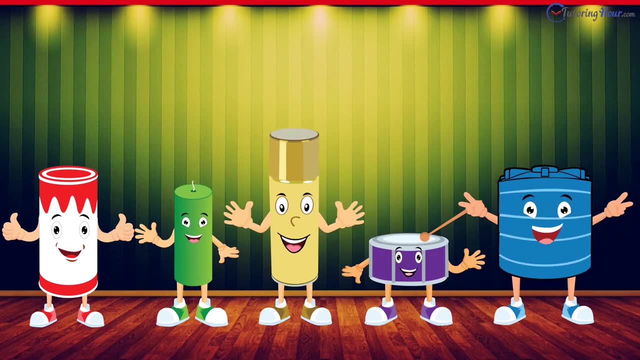 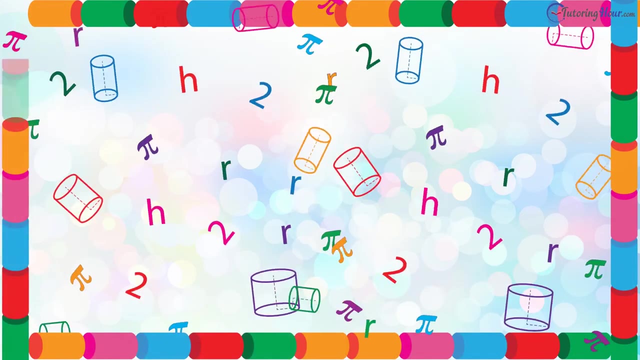 Hello and welcome to Tutoring Hour. Meet the soup can, the candle, the bottle of perfume, the base drop and the large water tank. All these are cylinders. In this video, I am going to walk you through the process of finding the volume of some of these cylinders. Volume is the.